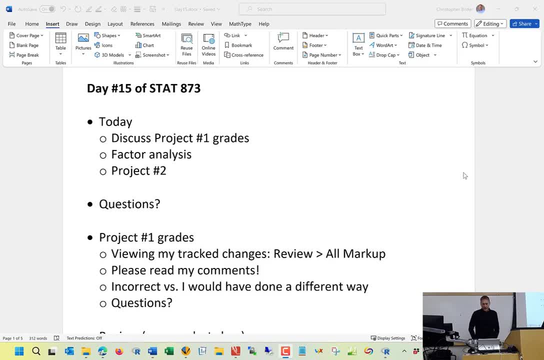 Let's begin class here. So this is day 15.. Some things were about halfway done with the semester. Today we will briefly talk about project number one. We will continue with factor analysis and we will also briefly talk about project number two. Are there any questions? before we begin. 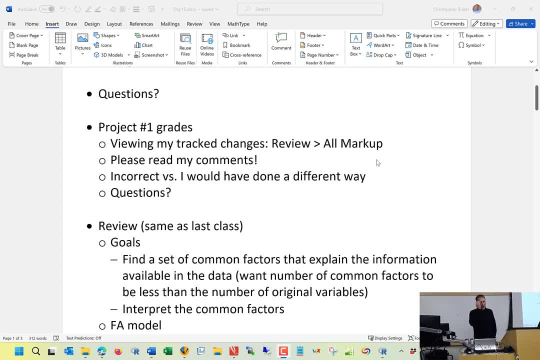 So, with respect to project number one, obviously everyone- well, each group- had a different data set so I don't have an answer key to pass out to everyone. So I tried to make a lot of comments on the projects and hopefully, if I did take off points, it made sense why I did that. But of course, if you have any questions about it, let me know. 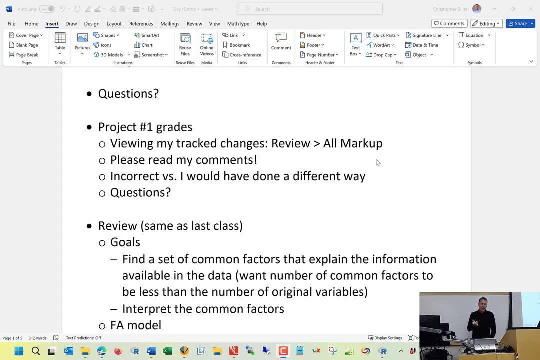 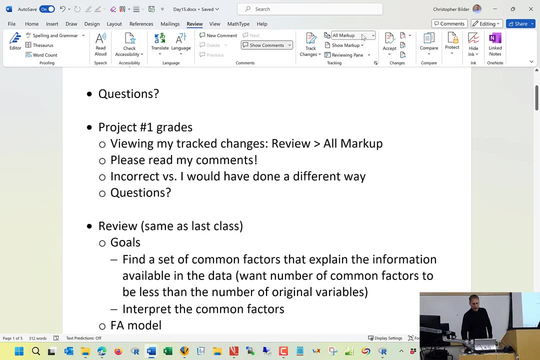 Now, just as a reminder, when you view the project number one, you will see that there are a lot of questions about it. So if you have any questions about it, let me know. Now, just as a reminder, when you view the project number one, you will see that there are a lot of questions about it. So if you have any questions about it, let me know. 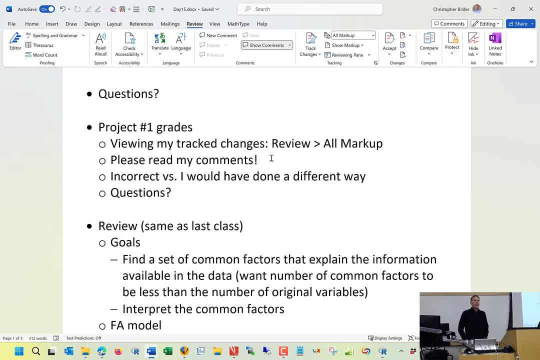 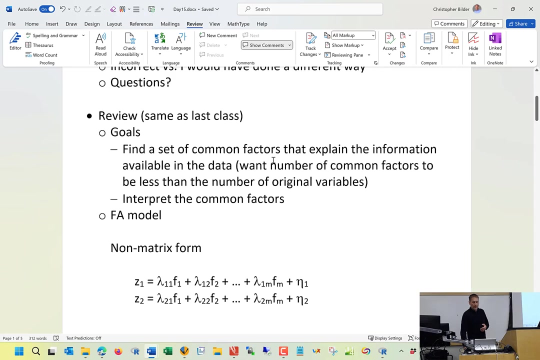 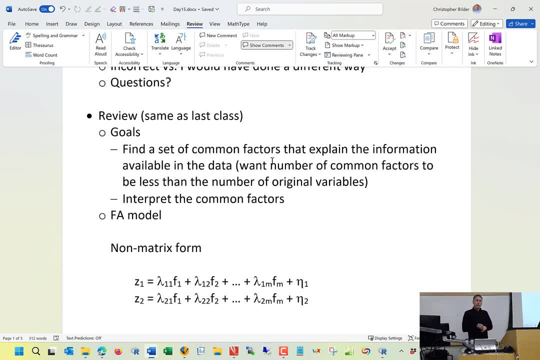 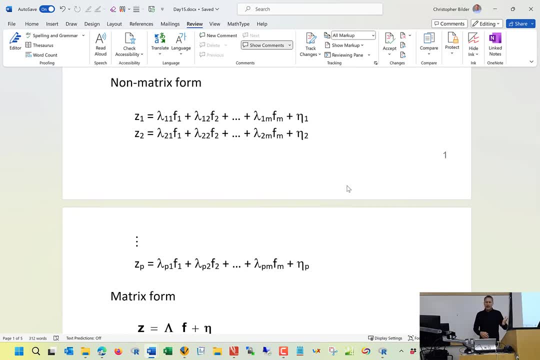 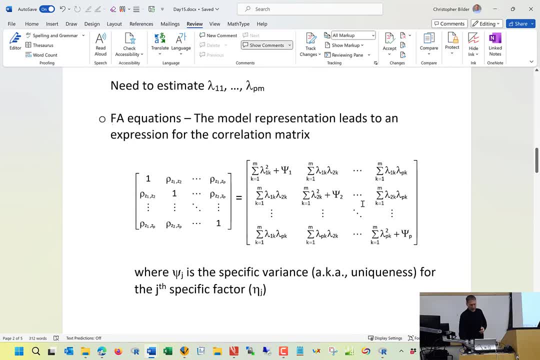 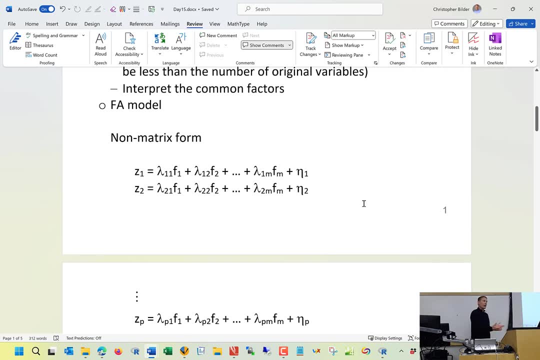 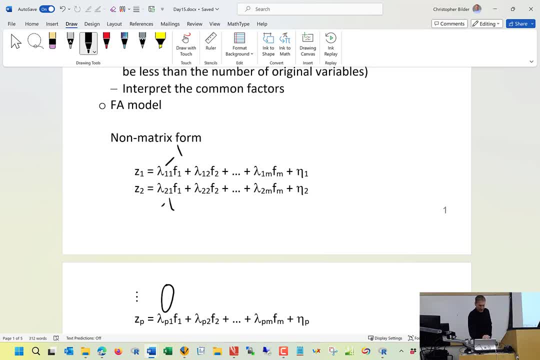 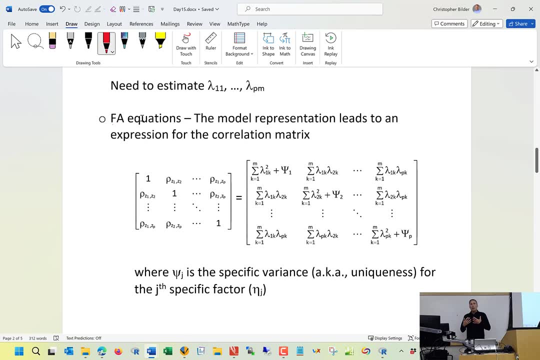 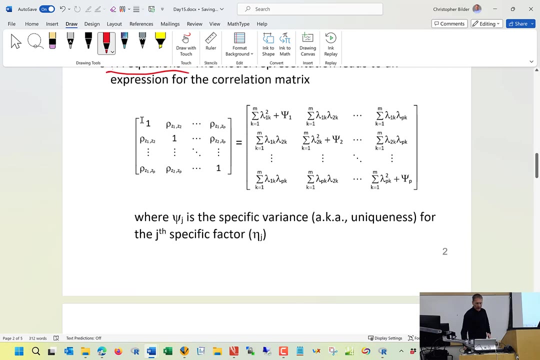 z1 represents whatever z2 represents. now, with this model structure, we can also write our correlation matrix in a particular form and we call this form the vector analysis equations. so notice. for example, 1 is equal to the sum of the lambdas for the first factor, each of these lambdas squared plus now the 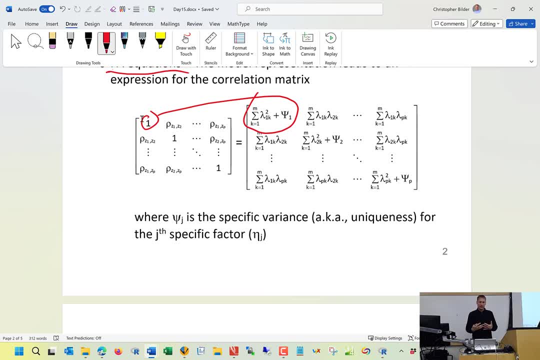 specific variance. this is the variance of the specific factor. also notice here that rows of z1 and z2, in other words the correlation between z1 and z2, is equal to the sum of their corresponding lambdas represented in the first equation. in the second equation, the product of 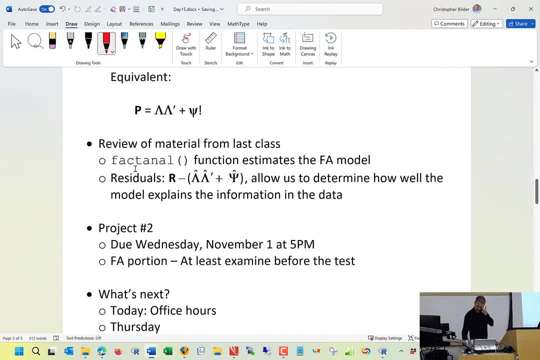 those lambdas, okay. so last time we learned about how we can actually estimate these lambdas. we can use the fact-anal function. it gives us maximum likelihood estimates, and last time we left off talking about residuals. these residuals allow us to assess how well the model is doing, similar to a regression analysis, when we 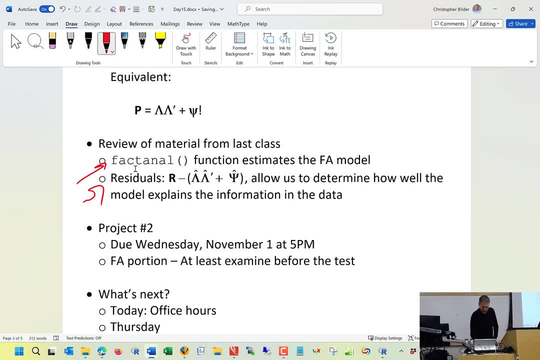 had residuals and you know, based upon these factor analysis equations- this is a, basically a matrix- represent representation of them. we know these factor analysis equations should be set equal to our correlation matrix. well, you want to do the estimation doesn't all work out exactly right. so in the end we 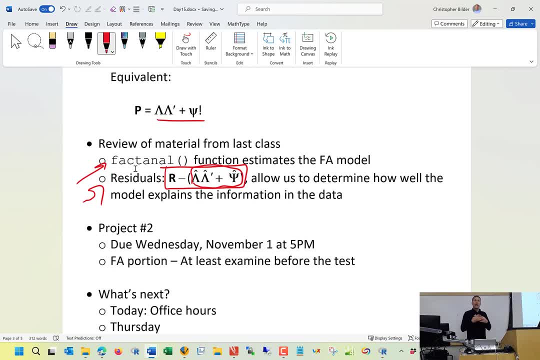 will like these residuals to be as close to zero as possible, as- and if they all are, that says the model is doing a good job. if we have some residuals that are kind of far from zero, then that says okay, this factor analysis model isn't explaining as much about the correlation matrix as we would like and that questions: is this a good model? so 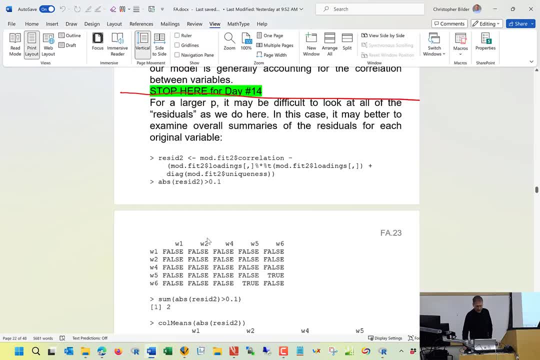 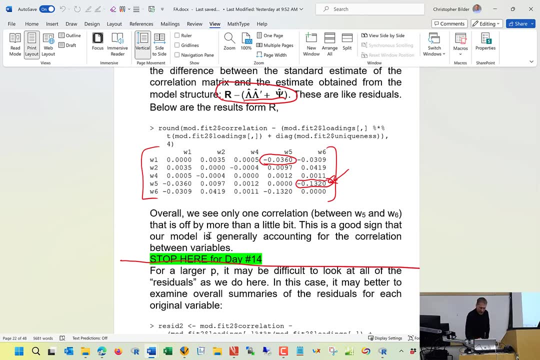 then that leads us then to where we left off. so, with respect to the goblet data, last time we found these residuals and where i have- uh, let's see here just a little bit of racing- we found these residuals using matrix algebra and there was only one residual. that maybe. 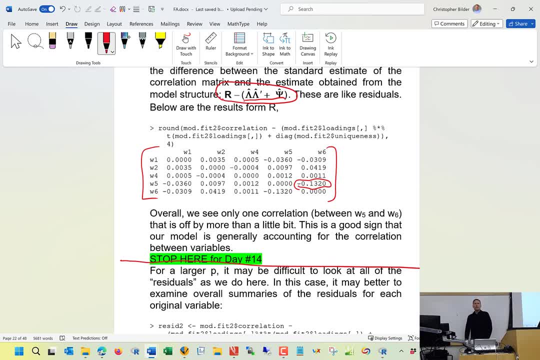 caused us a little bit of concern, but in the end it's not too far from zero. so, uh, overall this seems to be a decent model. now, if i had a residual of, let's say, 0.4, then that would cause some concern, because think of it what it means, and this is the the um. 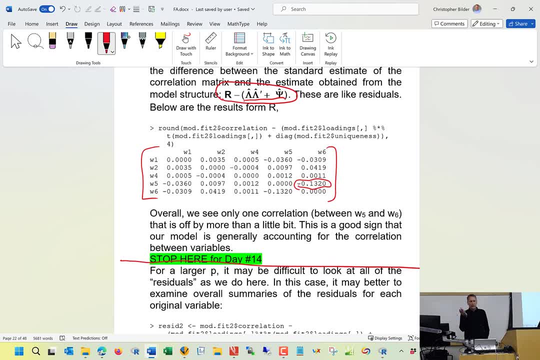 the example that i kind of used last time, where you know, if someone told you the correlation between two things was 0.3 and then they came back a few minutes later- so you know i was wrong, it was actually 0.7- that would cause you some alarm. but if someone instead said the correlation, 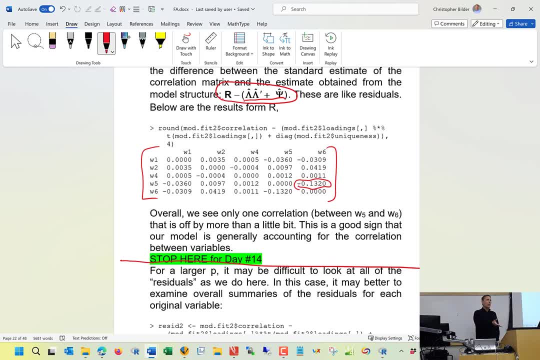 was 0.3 and then say, oops, sorry, i made a mistake, it was 0.4. in the end, in the grand scheme of things, that probably won't make much of a difference to you, and so that's how you can interpret what these residuals represent now. so now getting to new. 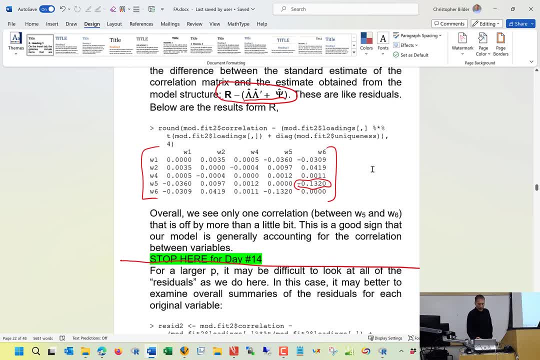 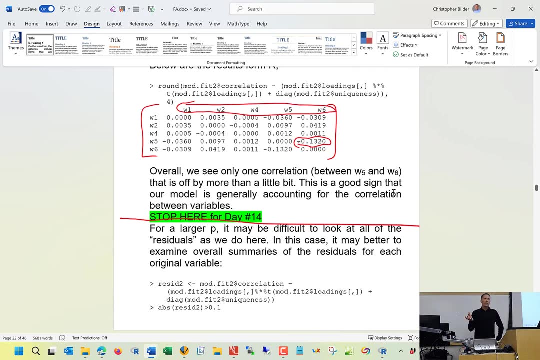 material. there are going to be times where we have more variables than in this case with the goblet data, only five variables. so it might be nice to have, let's say, um, maybe a quick way to check all these residuals: are they larger than what we would like or not? 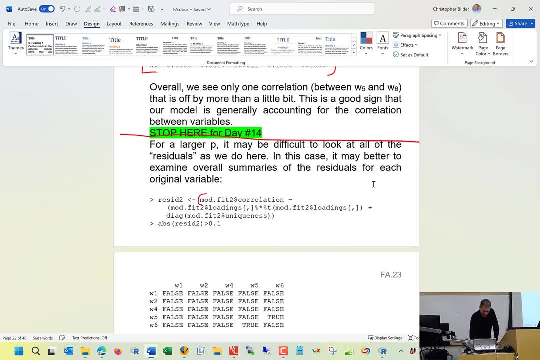 one could do is. i'm not going to go through the details here, but here's the from from last time. here's how we actually use matrix algebra to find these residuals. let's say, i put these into an object called resid 2 and then, if i say, abs for absolute value. 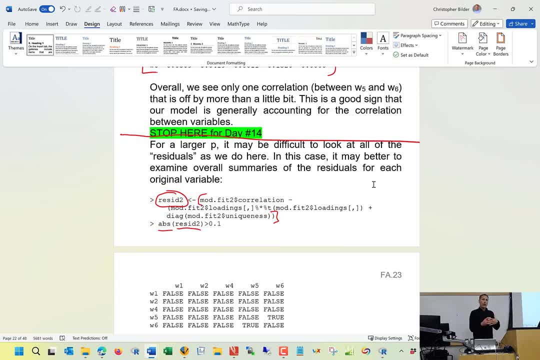 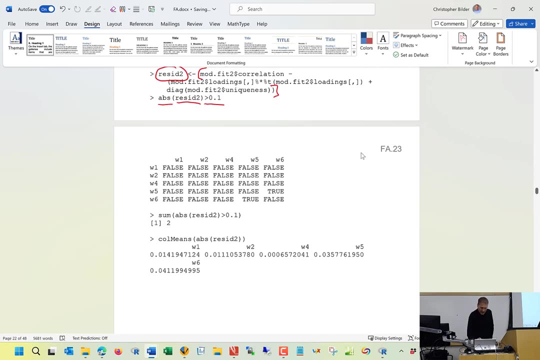 of resid 2. it's going to find the absolute value of all those residuals, one at a time, and then, if i say greater than 0.1, is going to do a logical check: is the abs, is the residual and absolute value greater than 0.1? and if it is, you get it true, it's not, it's a false. so this is a quick way. 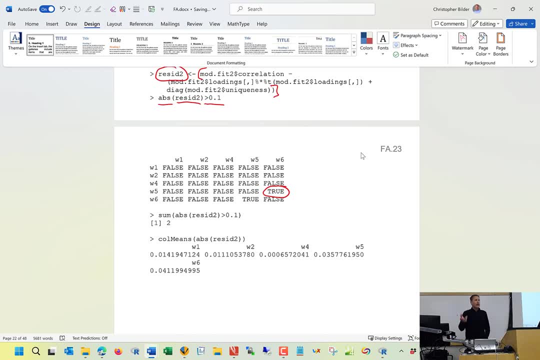 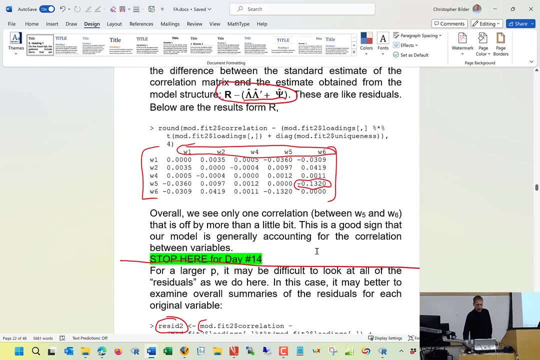 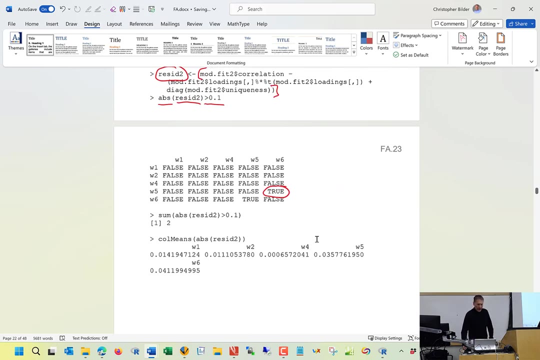 imagine if you had a 10 by 10 or a 20 by 20 matrix. it allows you to see, okay, where is this occurring, and you know that can be easier than looking at every single number that might be in there. another thing that you can do, then, is that if i were to also put the sum function with that. 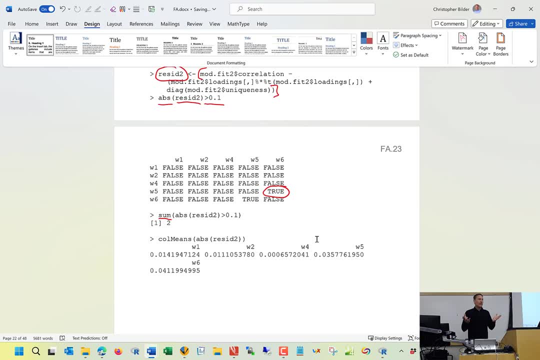 meaning, let's add all up. add all this trues and falses up. you might be thinking: well, how can you add trues and falses up? well, r translates the true to a one, a false to a zero. so notice, here i had a value of two. why? well, because of these two right here. now, remember, if you're going to 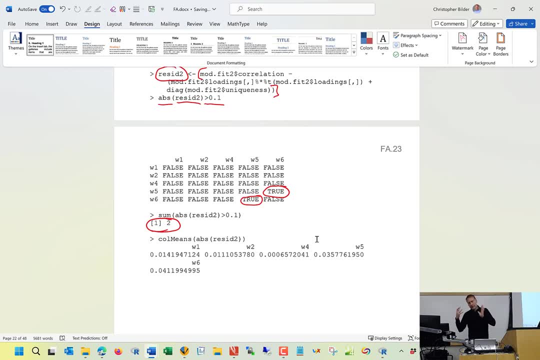 remember that the correlation matrix, and also the, the representation for our model, is going to be symmetric. so how many of these actual residuals are greater than 0.1? only one. so i just always think of this divided by two, two divided by two is one. now you might be thinking, okay, well, if it's. 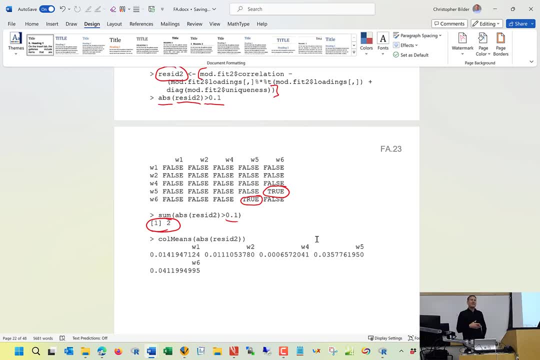 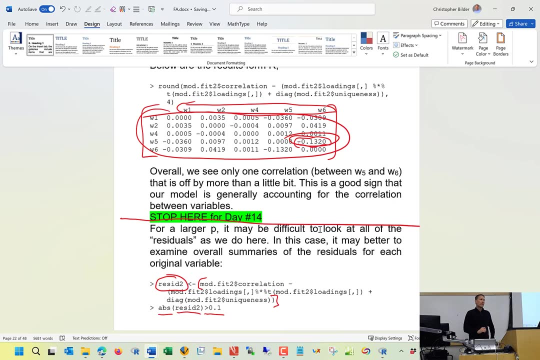 0.1. i'm in pro. i have a problem? no, it's just. this is a number that i put there because i knew that one case where it would come up as true- you know, maybe you know at least 0.2. i start getting worried. 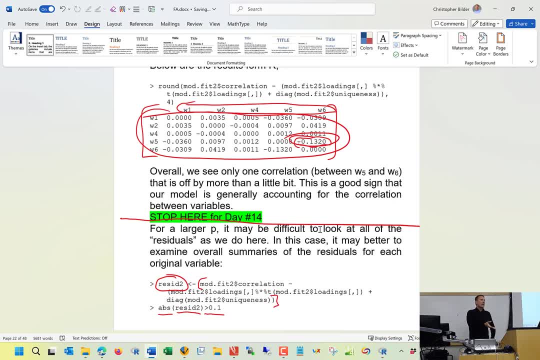 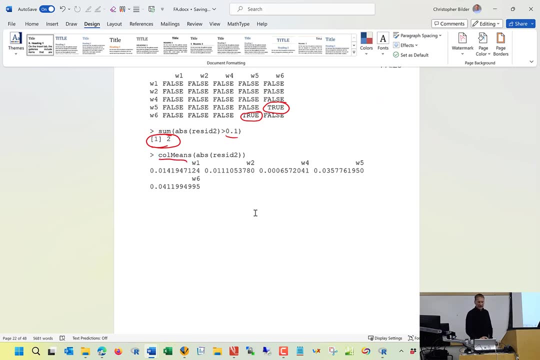 um, if i have, let's say, if i, let's say if i use 0.1 there and i'm having a lot of these residuals coming back to be greater than 0.1 in absolute value, then that would also cause me concern. also, you could use the call means function to kind of get like an average residual for each of the. 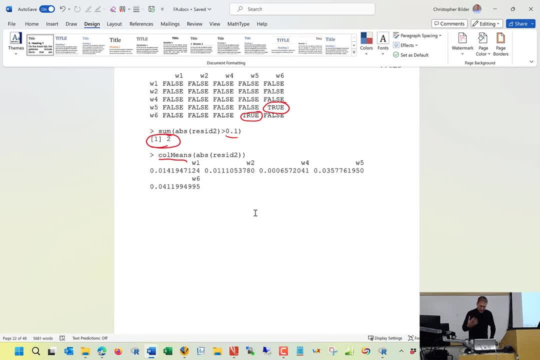 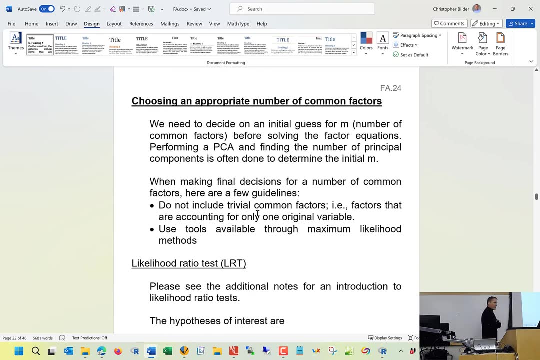 columns, and that can be helpful as well, you know, especially when you have more variables. okay, so now a new topic with factor analysis. so how do we choose the number of common factors? should i use one, should i use two, should i use three? um, and in the goblet example i said, okay, we're going to use two here, what you're going to? 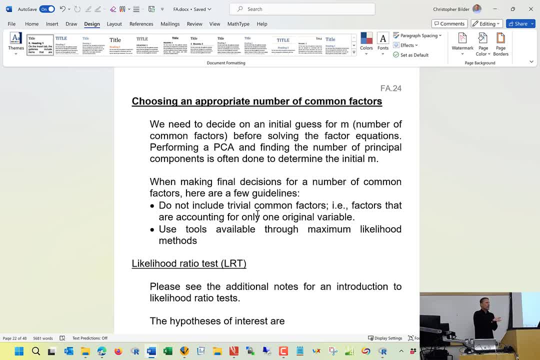 find out a little bit later on. if you even want to talk about how to do maximum likelihood today, you'll need to say: oh, point here. 2 seems to be okay and we'll look at that specifically very shortly. um and so when you decide, let's say how many common factors to use. finally, in the end. 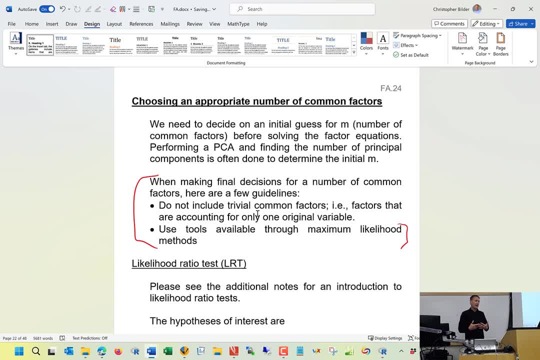 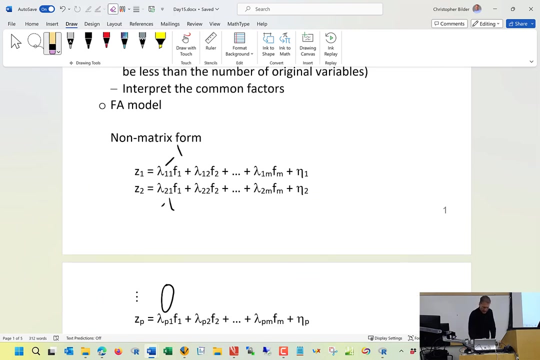 there's two things to think about. first of all, as you will see shortly, allows to say okay, is one better than two, is two better than three, so on. but also something else to think about is this: do not include trivial common factors. what does that mean? let me go back to my model here. let's say for: 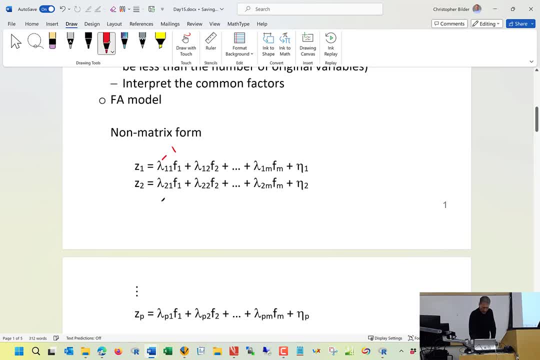 common factor: 1. lambda 1: 1 was 1. lambda 2: 1 was 0, and all the other languages with 0 as well. f1 will be a trivial common factor. what that means is: okay. all it is is just representing z1, so why don't you just take z1 out of your? 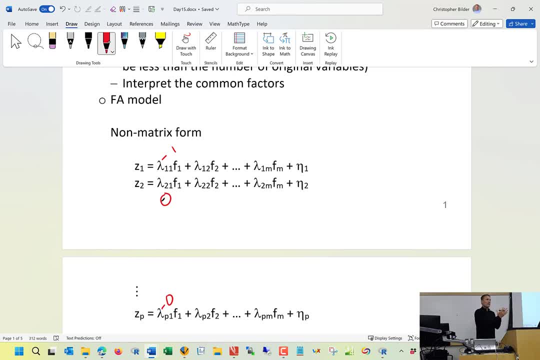 factor analysis. just treat that separately and then do the effect analysis on the rest of the variables. that would be a better way to do it. what this is saying is that z1 is the common factor and z1 is the common factor and z1 represents something that's distinct among all the, in terms of all. 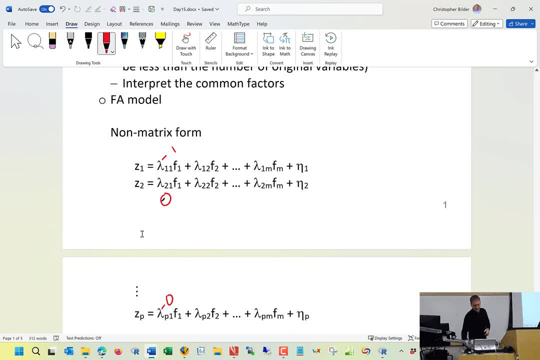 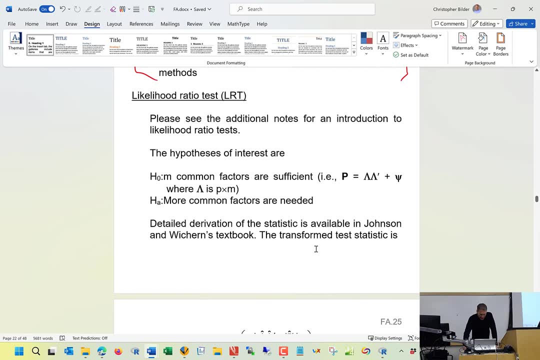 your variables, so just treat it separately. so so we want to avoid these trivial common factors. okay, so one commonly used tool. when one is has a likelihood function, uses a maximum likelihood estimation and one wants to make decisions about a model, one commonly used tool across a variety different applications, not just factor analysis and something called a. 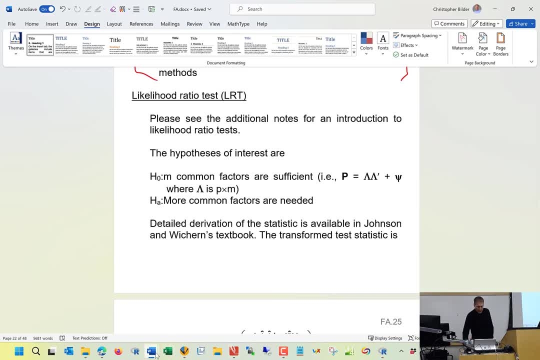 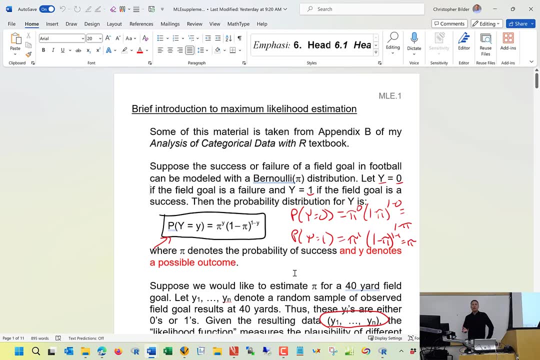 likelihood ratio test, and so in my additional maximum likelihood estimation notes I have a brief introduction in likelihood ratio tests. I wouldn't be surprised that some of you have seen it before what others have not, or you've read hundreds of projects, and so it could be anything that you might. 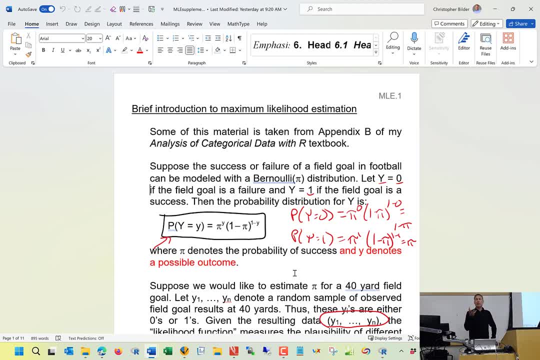 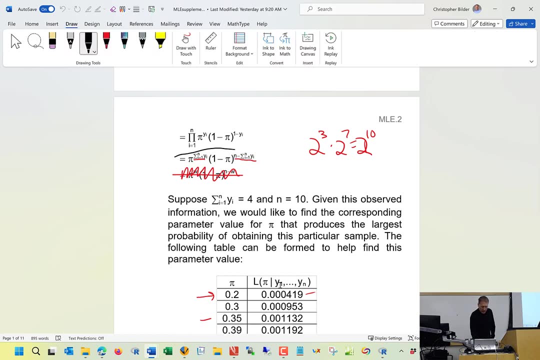 like and figure out. so after etc and etc, etc. and haven't seen it before. we should try that in a few times until we don't follow through here. so whatever you're doing now, just know how the algorithm will deal with that. behaviors function as pi raised to the sum of the y's, which would be the number of successes. 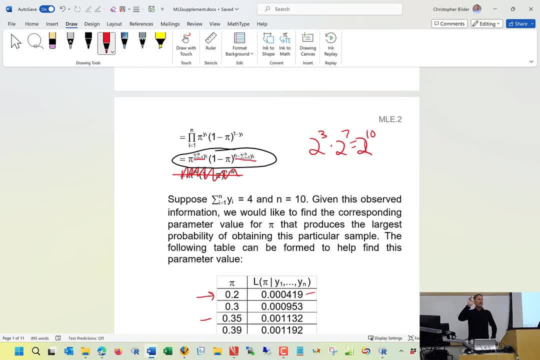 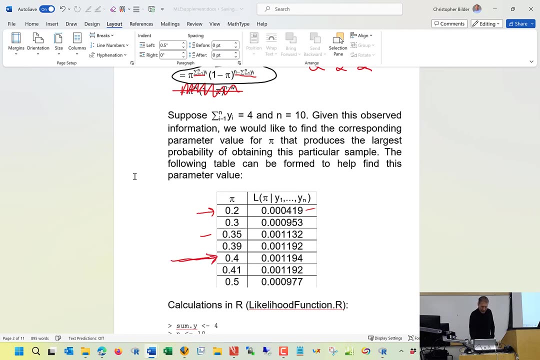 times 1 minus pi, raised to the n minus the sum of the y's, in other words, number of failures power. This was our likelihood function. We used this to find maximum likelihood estimates. The way that we did that was we looked at this function as a. 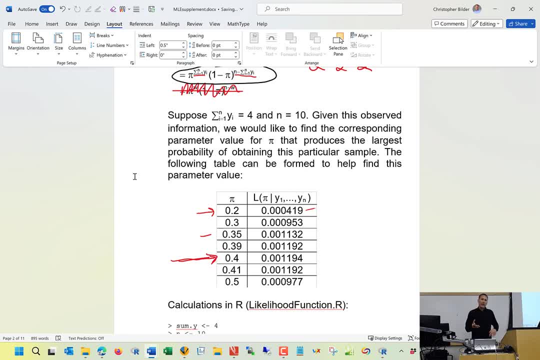 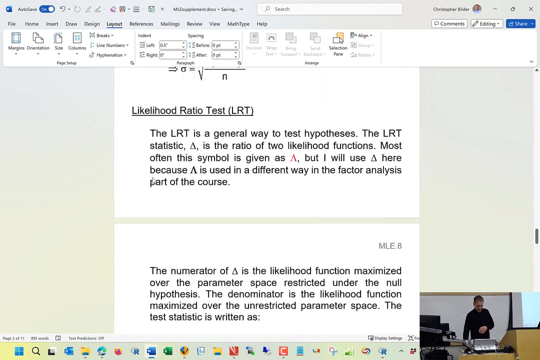 function of pi. The value of pi that made this likelihood function as big as possible represents the most plausible value for pi. That's our maximum likelihood estimate. When we had four successes out of ten trials, it ended up being pi was 0.4, or we call it pi hat. now It's equal to 0.4.. 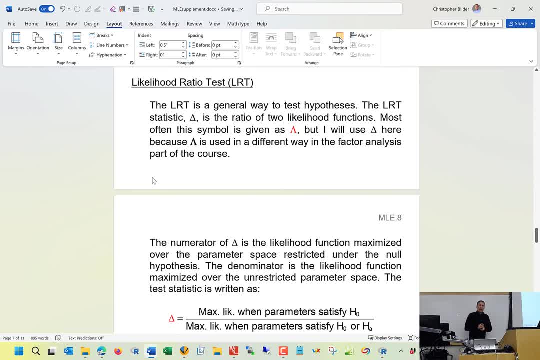 Okay Now likelihood ratio tests. So we're going to form a statistic. You know, in order to do a hypothesis test you need some kind of statistic. We're going to call this statistic. uppercase letter delta. Outside of this class, you typically see people use an uppercase lambda to represent the 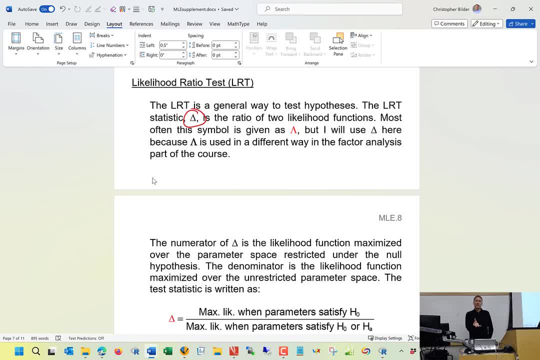 statistic- Obviously lambda in this section- means something else. It's the factor loading matrix. So that's why I just decided to use a delta instead. And this is what delta looks like. Again, it's a statistic, And since I'm 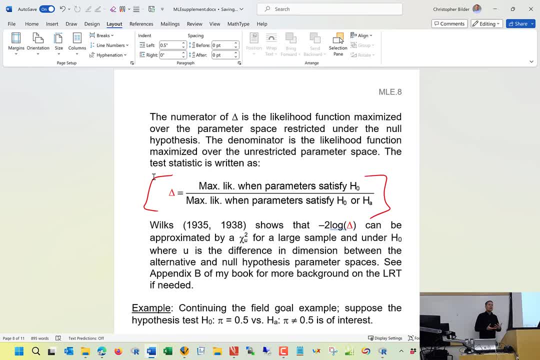 going to call it a likelihood ratio test. as you might expect, it's a ratio of two likelihood functions. In the numerator, we have the maximum possible value of our likelihood function When our parameters for whatever probability distribution we're looking for, or you can think of equivalently in terms of the model- when the parameters 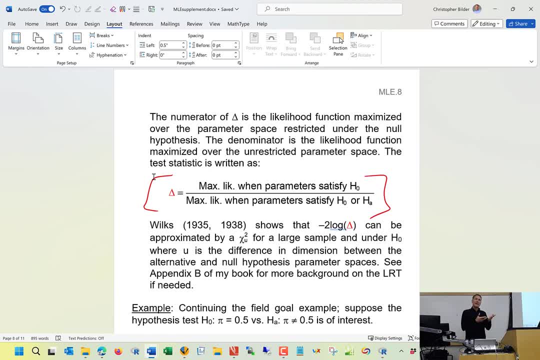 satisfy our null hypothesis, what is the maximum possible value that the likelihood function can take on. That's the numerator. The denominator is a little bit more general. It says what's the maximum possible value that the likelihood function can take on when the parameters either satisfy HO or the alternative. 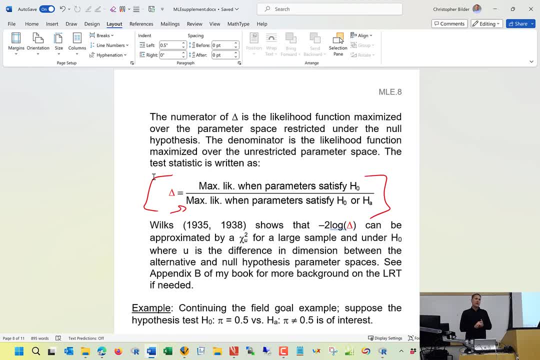 hypothesis HA. And so we can see that what's in the numerator is kind of like a subset of what's in the denominator. and notice, I have HO here, I have HO or HA there, And so it's a ratio. It's always going to be between. 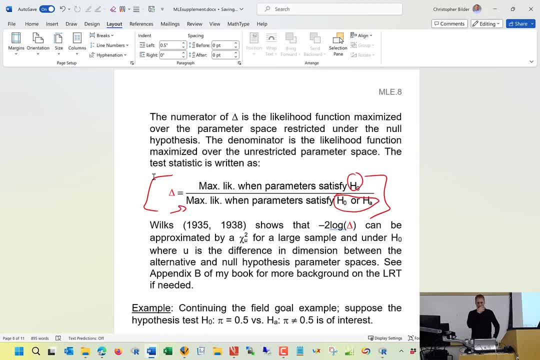 and 1. Now we need to be able to then determine what would be, let's say, an unusual value for Delta if the null hypothesis is true. You know this goes back to your first stat course. You know, like, let's say, if you did a hypothesis, 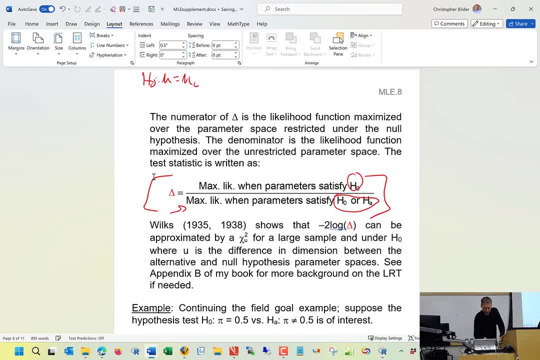 test of. you know, usually the first one that's taught is something like this, where you're testing the population mean, is it equal to some number? we'll call it mu zero or not. And so we assume the null hypothesis is true and we look to see: 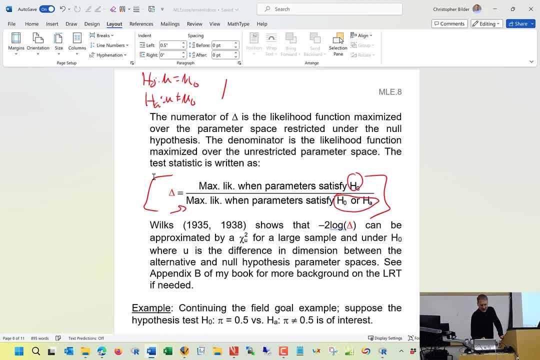 well, what would be an unusual value of some kind of, let's say, T test statistic? So you probably wrote it out something like this: and the sample size, S is the sample standard deviation. actually, X bar is the sample mean. and what you do is you plot the T distribution centered. 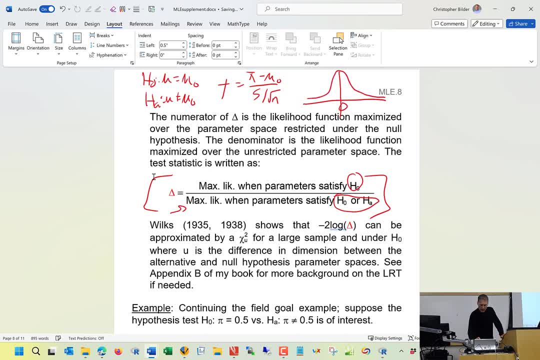 at zero. There is a T distribution and basically anything that's out on the tails of the distribution is an unusual value for your test statistic, if the null hypothesis is true, because there's very little probability of it. And so then, when you have a test statistic calculated on your sample, if it felt 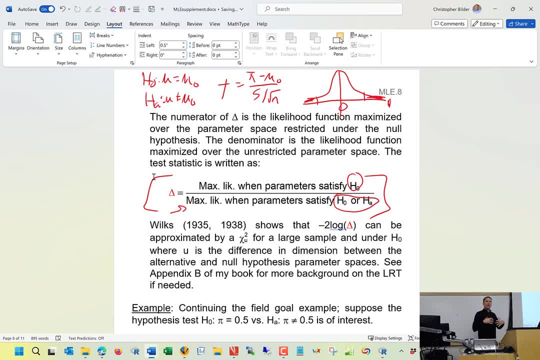 like, let's say right here, relative to that x-axis, then you know, hey, this is a number that's unusual. let's reject HO. It would be very unlikely for HO to be true and still observe this particular data. Now we want to do something similar with. 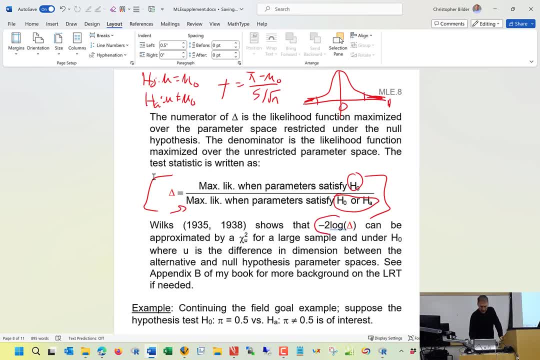 this delta. Now a long time ago, when these likelihood ratio tests first developed, just in general, not necessarily from factor analysis, A particular individual found that if I took negative two natural log of delta, I could use a chi-square distribution with this delta. So what this is saying is that if 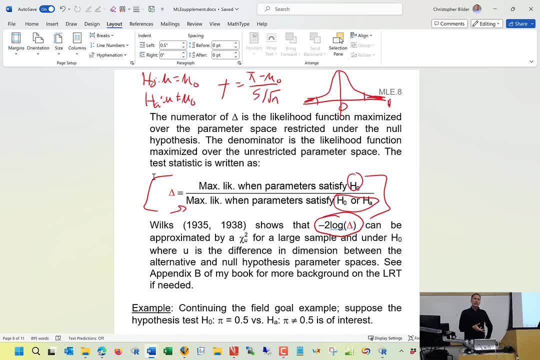 the null hypothesis is true. I would expect my values of delta if I were to go out and take a sample, calculate negative two log delta. go out and take another sample, calculate negative two log delta and keep on doing it over and over and over. 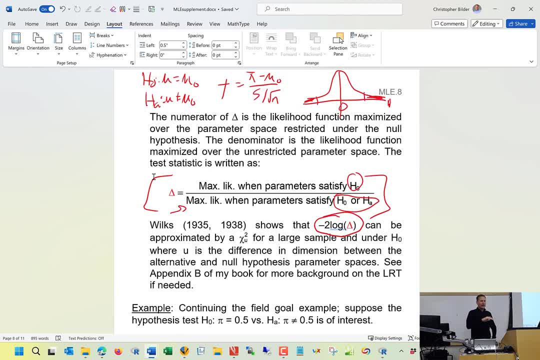 and over again. assuming the null hypothesis is true, I would expect, let's say, a shape of the histogram to be very similar to a chi-square distribution. essentially, Now, this all works out if you have a large sample, and the reason being is: you know, you know what? what stat majors, for example, would learn not until they're a. 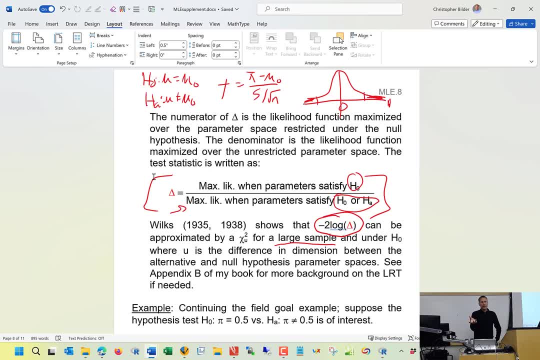 PhD student is, you would actually learn like how you can mathematically prove that in terms of as in, If one goes to infinity, this statistic has a chi-square distribution. Don't worry about it, but that's basically where this comes from, And long as you don't have a small 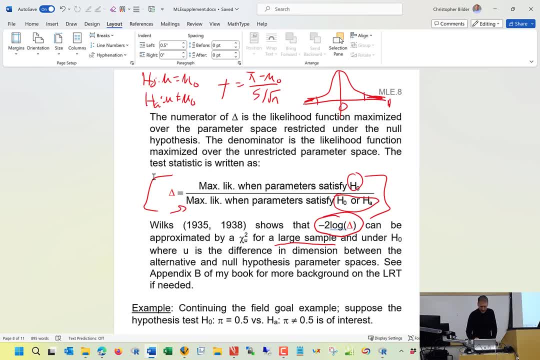 sample size. this is going to work out fine Now with the chi-square distribution. if you remember, there's always a degrees of freedom parameter that controls the shape. The degrees of freedom here ends up being the difference in dimension between the alternative and null hypothesis parameter spaces. 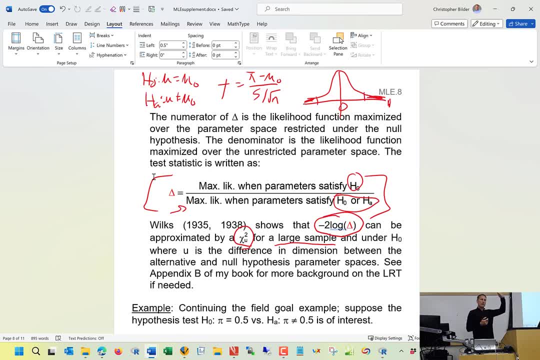 What that just basically means is, if the null hypothesis is true, how many parameters do I have left that are allowed to be anything else- Anything. And conversely, if the alternative hypothesis is true, how many parameters do I have that can be any number? It's attracted? 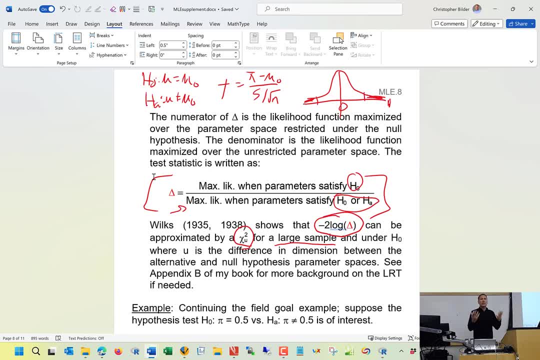 to, and then you get the degrees of freedom Now for us, um, um R. when we actually do this. in fact, analysis will actually provide the degrees of freedom for us, and we actually do this in subtraction, So we don't need. that's why you need to worry. 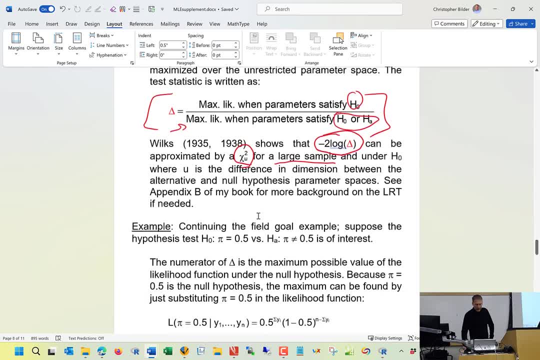 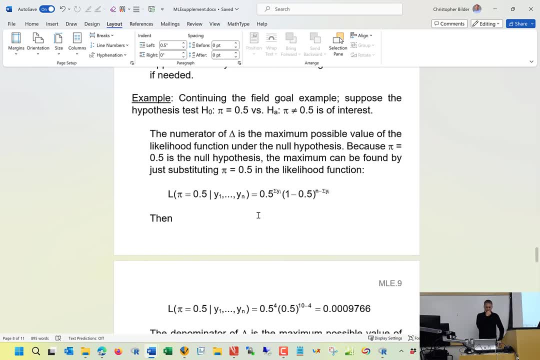 about some of those details. Okay, so let's look at an application. Yeah, So in this example, can you- I mean, I couldn't follow- what was the answer of the unusual value for the? uh, what null hypothesis, is true. so can you tell me what the answer is? 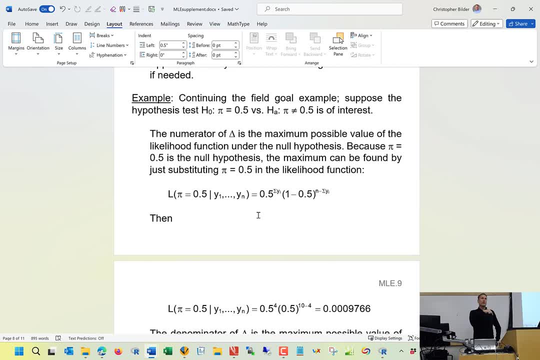 Sure, Uh, we'll do it in this example and if there's more questions, bring it up. And one reason why I like to, I like to um say it in that way, which was more general than maybe what you've experienced in another course, is that you know, in another course you know, 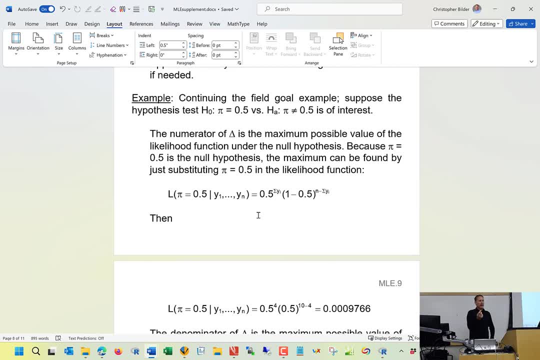 you're often given like a cookbook. you could say in terms of: okay, uh, if I'm greater than the one minus alpha quantile from a particular distribution, then I know to reject, otherwise I don't reject, And that is one way to teach it. 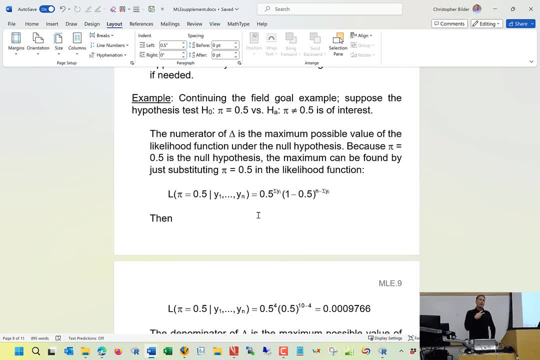 But it also doesn't allow you to, uh, gain an intuitive feel for why. that is the recipe for deciding to reject or or don't, And- and hopefully with some of the stuff I'll, I'll say here that that will be helpful. 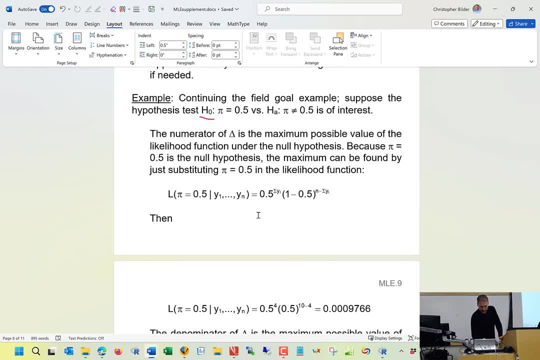 Okay. so let's go back to this field goal kicking example. Let's say simply: I want to test: is pi equal to 0.5 or not? Okay, So I need to find first of all delta ratio of two likelihood functions In the numerator- I assume the null hypothesis is true- and find the maximum possible value. 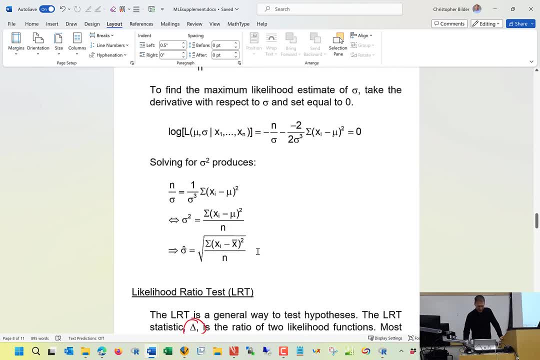 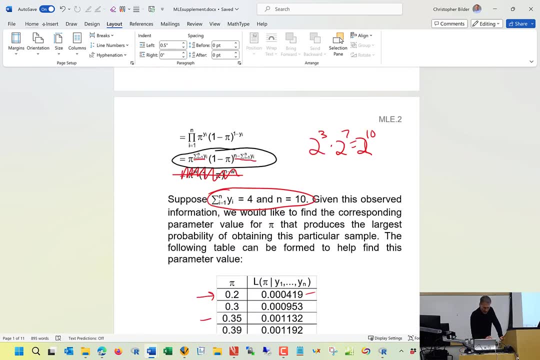 that that likelihood function can take on. Well again, let's go back to what the likelihood function looks like. This likelihood function is here. Now notice: there's only one parameter in that likelihood function. So if pi is 0.5, I put that in there. 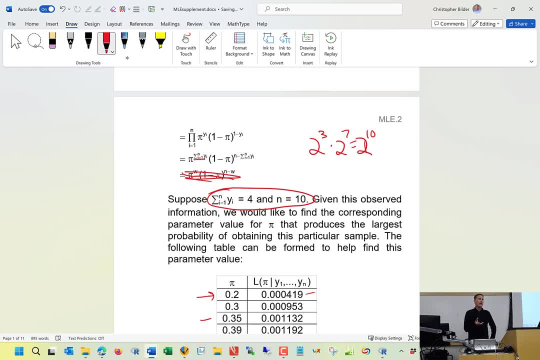 I put in my data values. let's say again: I observe four successes, ten trials, And that's just what the likelihood function is. it can't be anything else. So the maximum possible value of the likelihood function in this particular case is simply: 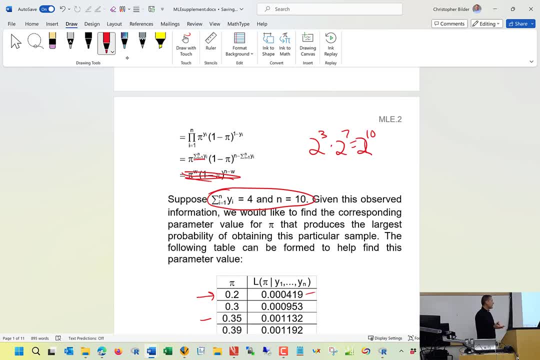 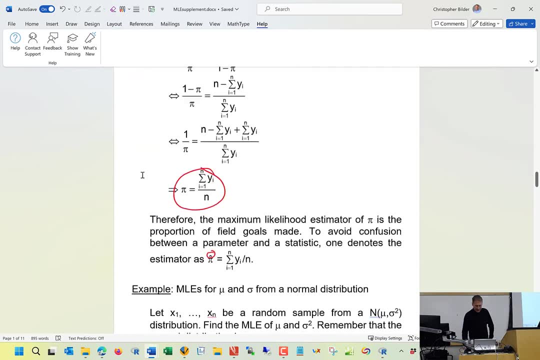 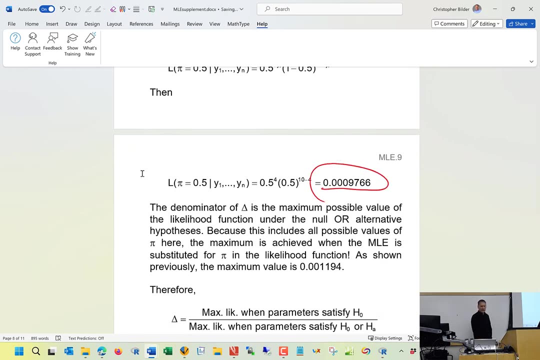 0.5 in there for pi, put in some of the y's of four, put n in ten, And that's what the maximum possible value of that likelihood function can be, Which is 0.5.. Okay, Which ends up being 0.0009766. 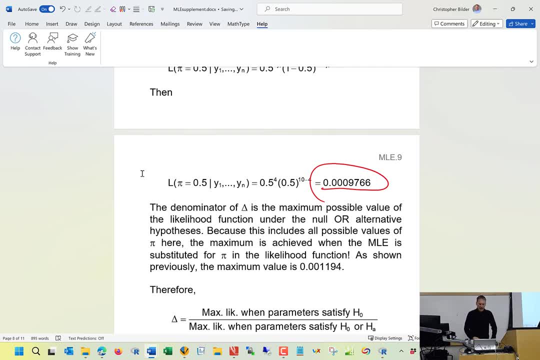 So that's my numerator. Now in the denominator I need to find the maximum possible value of the likelihood function when parameters satisfy HO or HA. HO is, pi is equal to 0.5, HA- pi does not equal 0.5.. 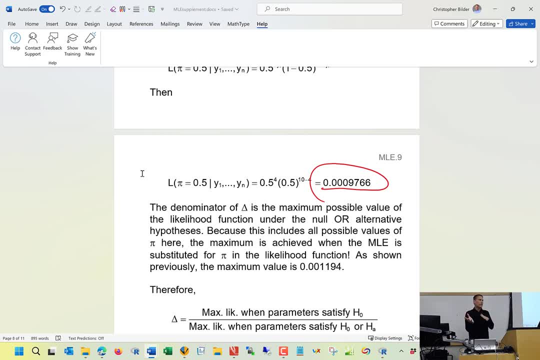 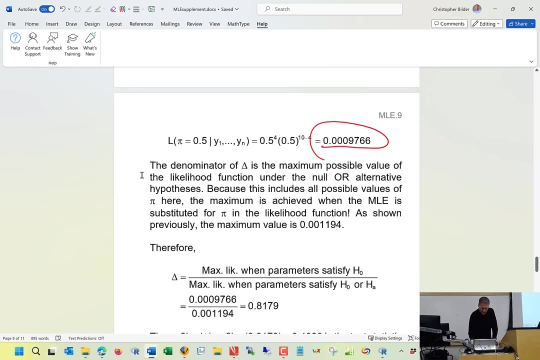 So the range of possible values of pi is 0 to 1.. Okay, So what is that maximum possible value of the likelihood function? We've already found it, Because that's where we were finding the maximum likelihood estimator, So that maximum likelihood estimator was 0.4.. 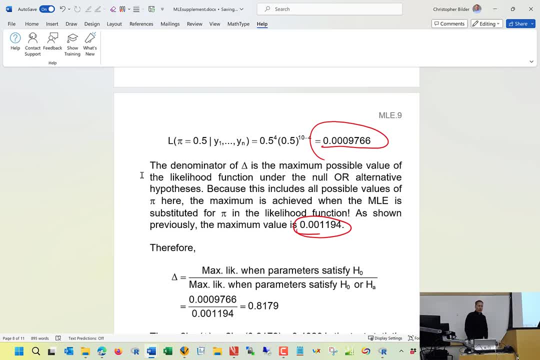 You just simply stick that into your likelihood function and you get 0.001194.. This corresponds to that table of different values of likelihood function that we found before. So now, if I take the ratio, I get 0.8179.. Okay, 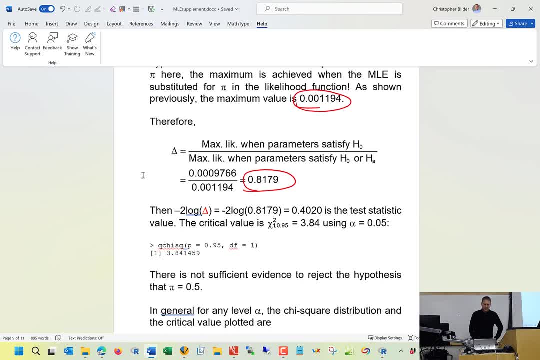 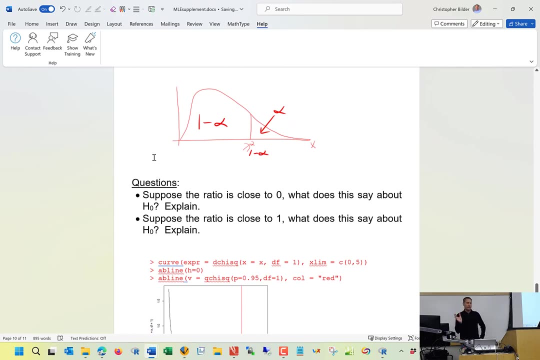 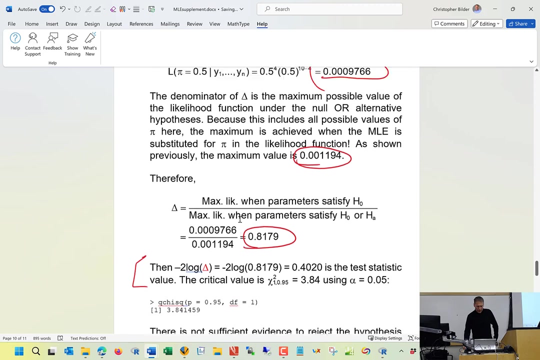 So that's 0.4.. Okay, Now, before we do this next step, I'm going to jump ahead here. I have two questions for you, Just in general here, Not necessarily for the field book. example: Suppose my ratio. 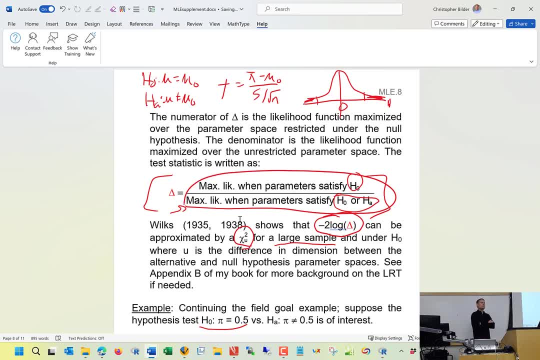 Suppose this ratio here: It's close, It's close to 1.. What do you think that says about the null hypothesis? I think I heard someone say it's true, Is that right? It's kind of saying that, Yeah, All of the possible times that we misdemean, not to name, not to give them a satisfied 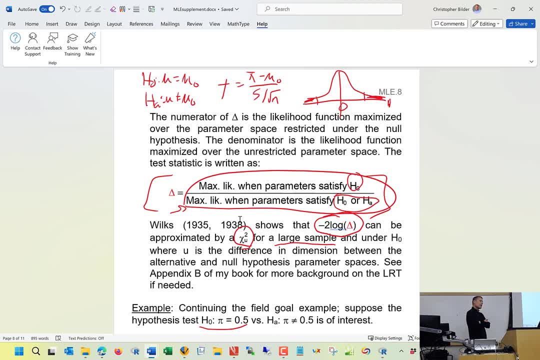 ratio. I think maybe we should say it this way: It's reasonable to have our null hypothesis. you know, yeah, essentially That our null hypothesis is reasonable given this observed data, Because if I take away that, having only the H0 restriction, my likelihood function isn't. 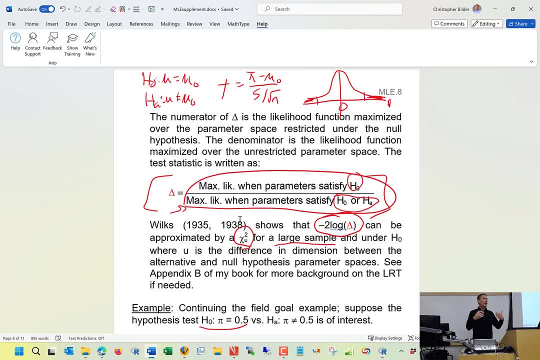 that much higher. Another way the likelihood function is measuring is the plausibility of particular values of your parameters, And so if the numerator is close to the denominator, I'm going to have a delta value that is close to 1, suggesting what's happening under H0 is reasonable for a particular problem. okay, 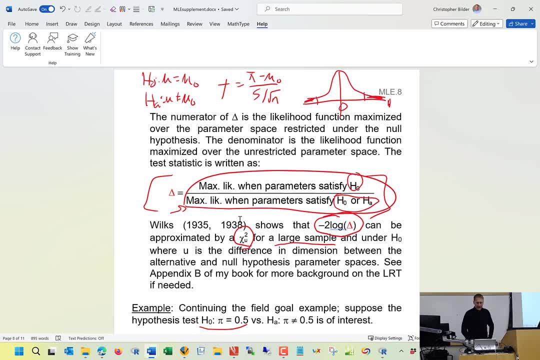 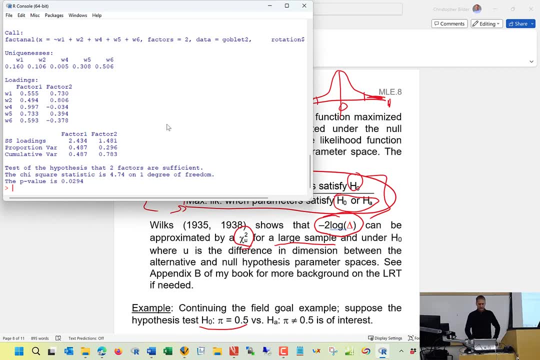 So what happens then when I take negative 2 natural log of delta, though? So I make this little transition. Well, let's just take a look at some possible values. So let's say, negative 2 log, is this big enough? 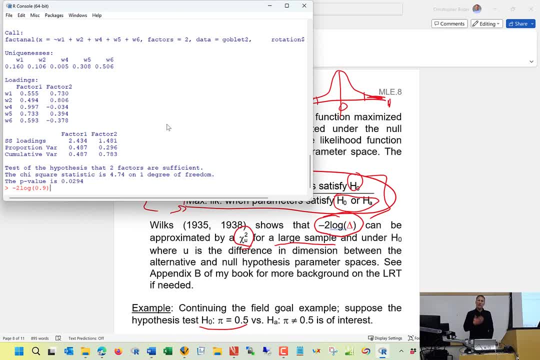 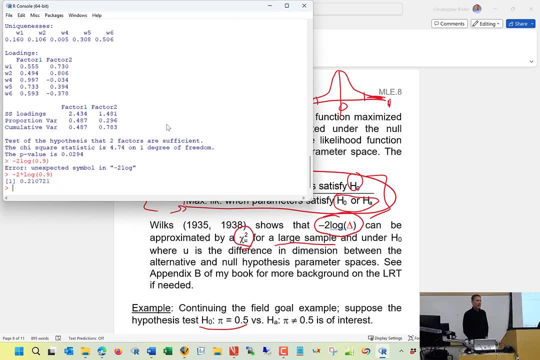 Negative 2 log of 0.9, so 0.9 is kind of close to 1, oops, use the right syntax. you get a value of 0.21, okay, Well, let's say it's 0.99.. 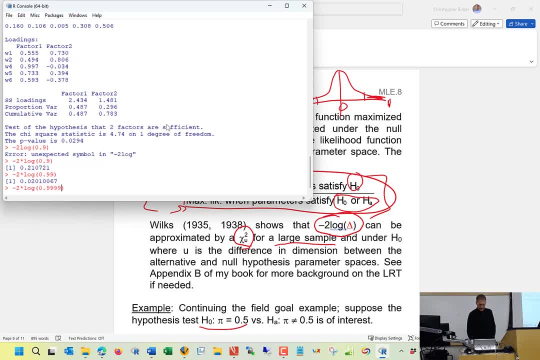 Okay, 0.02.. And I keep on getting closer and closer to 0.. So the closer that negative 2 log delta is to 0,, the more evidence there is that, yeah, what's happening under H0 is reasonable. 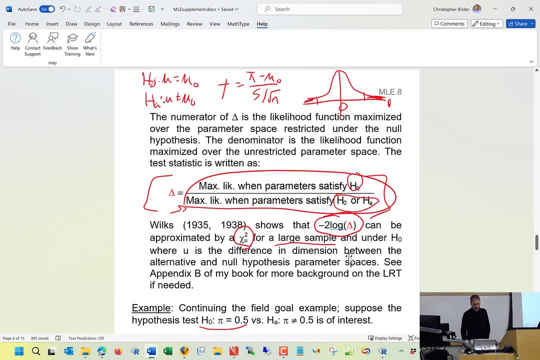 Now let's look at it from the alternative point of view. Let's say this ratio is close to 0. What does that say about the null hypothesis 0. Then it's likely false. Again, think about what a likelihood function measures. 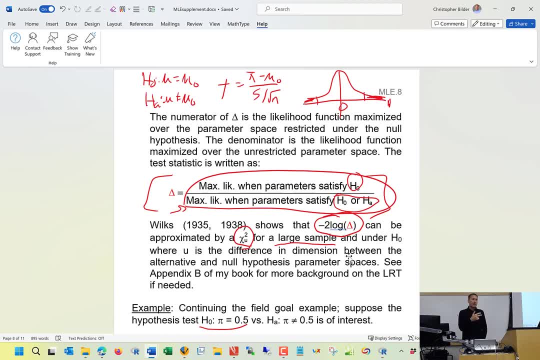 It measures how plausible your parameter values are. And if you don't have that H0 restriction anymore and that denominator then is much, much higher than what's in the numerator, That says then 0.99.. restriction of HO, it's just not reasonable, it's not plausible given your 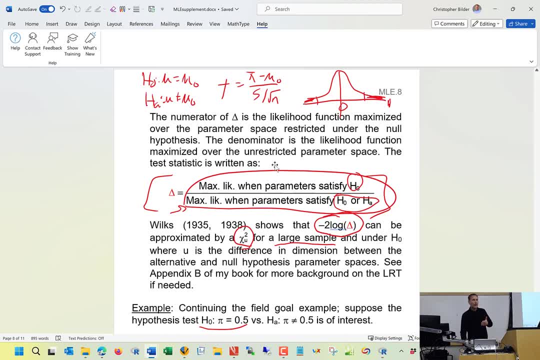 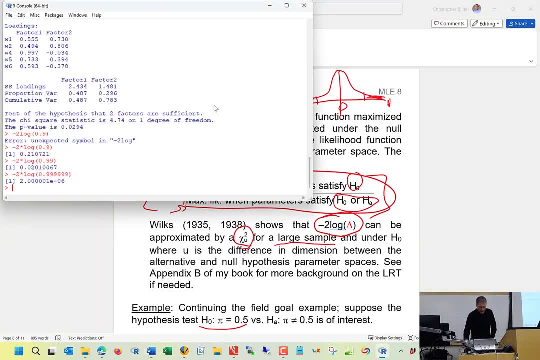 data, And so delta will be close to zero when the null hypothesis is false. What does that mean, then for our transformation? Well, let's look at point one there. for delta, okay, You get a value of 4.6.. Suppose I put. 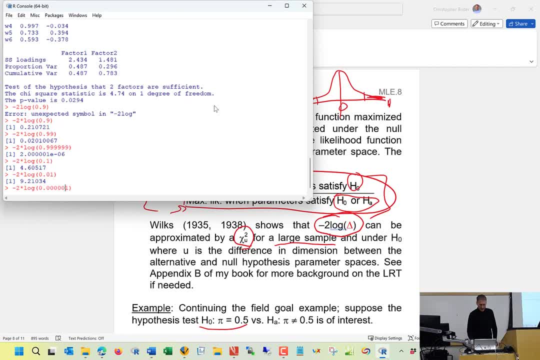 0.01 in there for delta and you can see that as delta goes to zero, negative 2 log delta increases. So when should you reject HO For a small value of negative log delta, negative 2 log? When should you reject HO For a small value of? 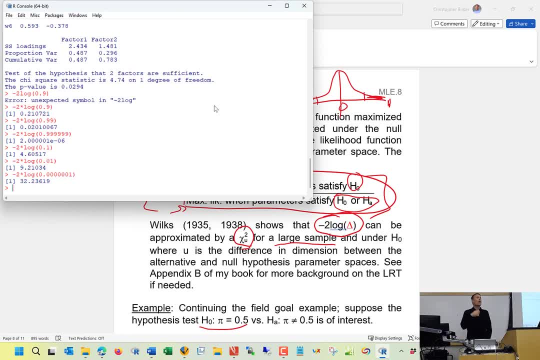 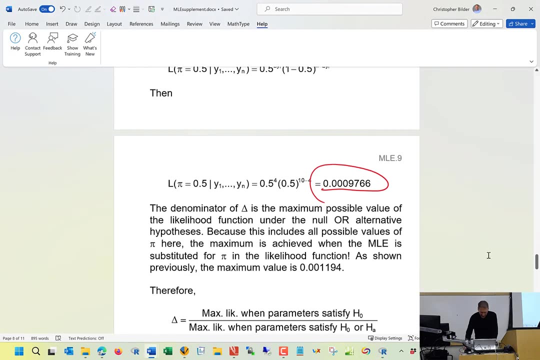 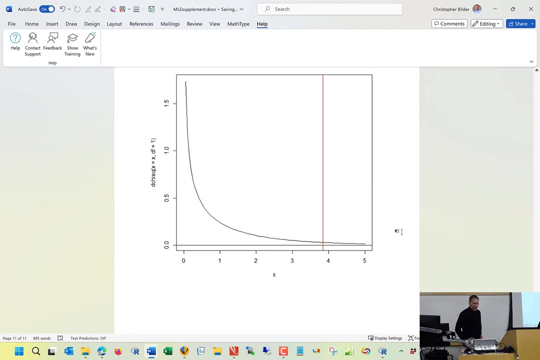 negative 2 times log of delta or for a large value, And then you might think: well, how large is large? That's where this chi-squared distribution comes in. So actually I did a little bit of a quick little plot here, So here's a plot of a chi-squared. 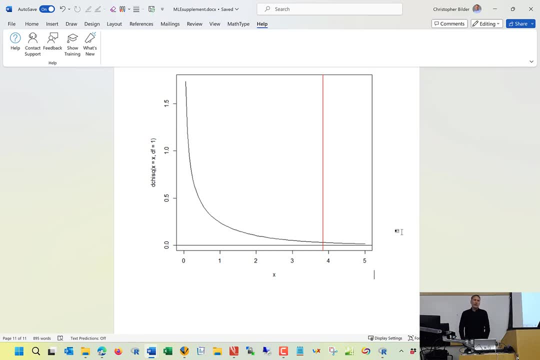 distribution with one degree of freedom, which happens to be the number of degrees of freedom we have for a field goal kicking problem. The reason being is because in the null hypothesis, if pi is 0.5, we have no more parameters. In the alternative hypothesis, pi is not. 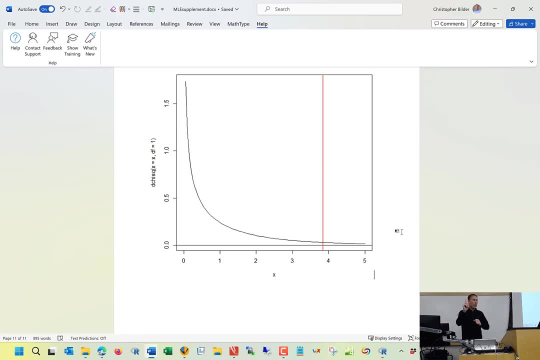 constricted, and so we have one parameter. So if I take 1 minus 0, we get 1.. To put it more precisely, it's the difference in dimension of the alternative hypothesis space versus the null hypothesis space. That's the formal way that I put it. 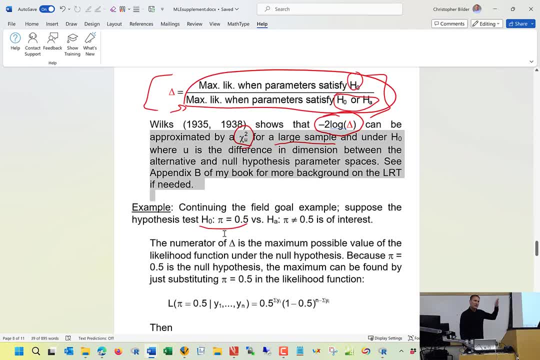 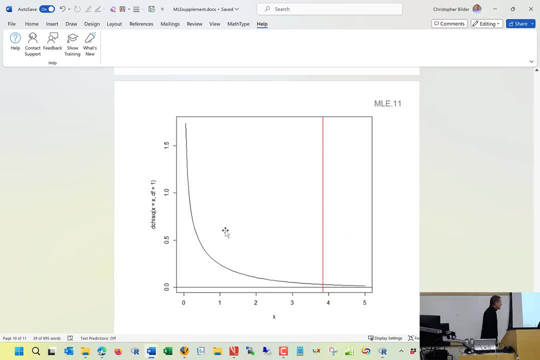 Right up here. So it's just the difference in the two possibilities for the number of parameters we have available to you under HO and HA. So this is an actual two-scale plot of a chi-squared one distribution. We can see it's really a right skewed distribution. 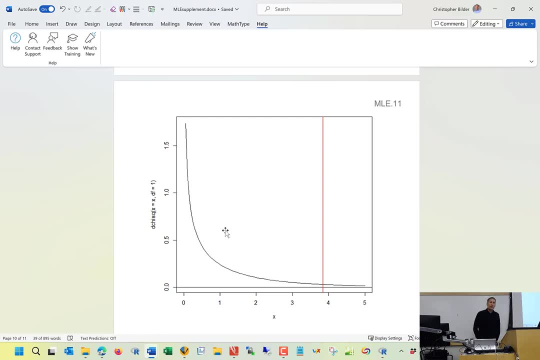 And similar to what I was showing you before relative to the t distribution when we did a hypothesis test for mu. we're looking for unusual possible values relative to the x-axis. Where do I have little probability underneath the curve And we can see that. 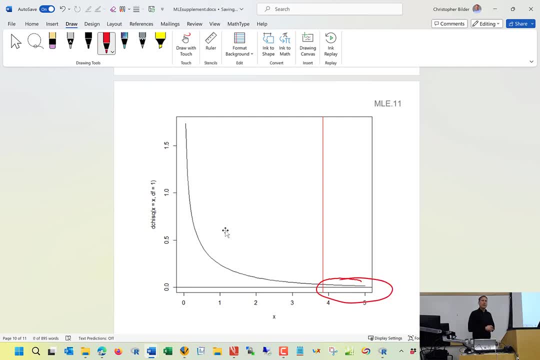 as we get farther and farther out on the x-axis. I have little probability there And in fact where I drew this line here, this is the 0.95 quantile from a chi-squared distribution. People will often denote this as chi-squared. then the subscript 0.95, comma 1.. This value 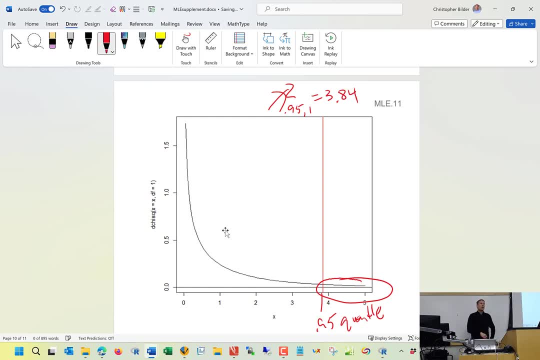 is 3.84.. So if I wanted to use, let's say, alpha 0.05 for my hypothesis test as a way to quantify what's unusual and what's not, I would use this as my critical value. And so if I have 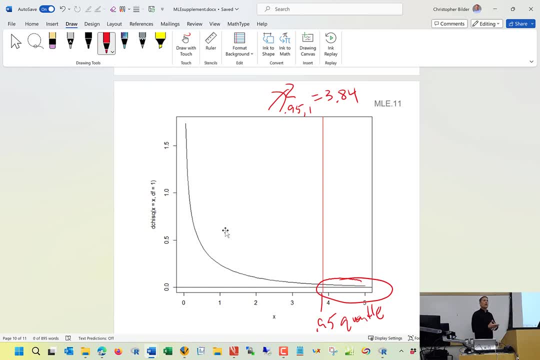 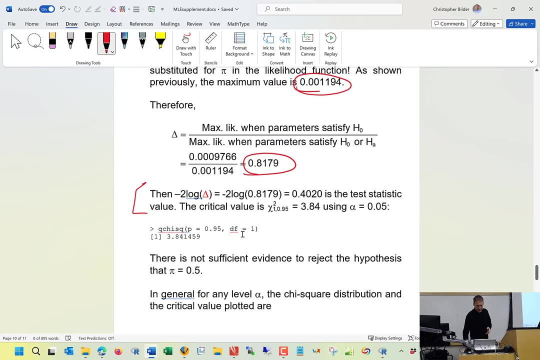 a negative 2 log delta that's greater than 3.84, I reject. Otherwise I don't reject. So in this particular case here we can see that negative 2 log delta ends up being 0.4.. That is less than 3.84.. 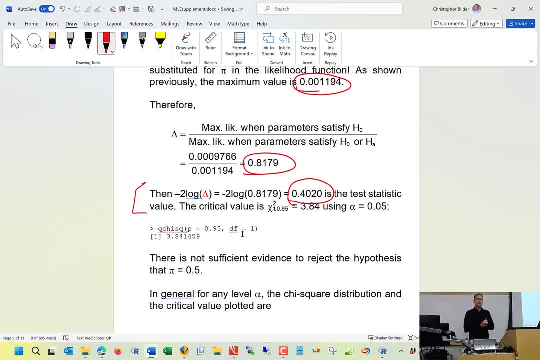 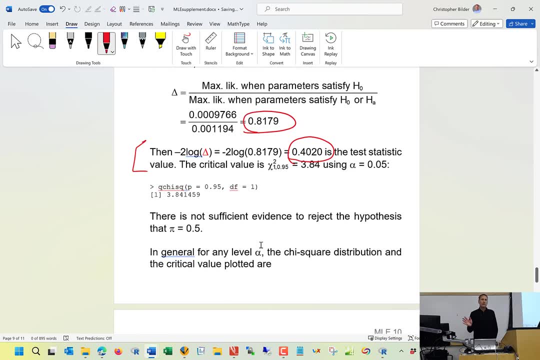 So I would say: don't reject Now, just as a little bit of a warning. this doesn't mean HO is true. It just means there's not reason to believe that it's false, given the data. Hopefully in your very first STAT. 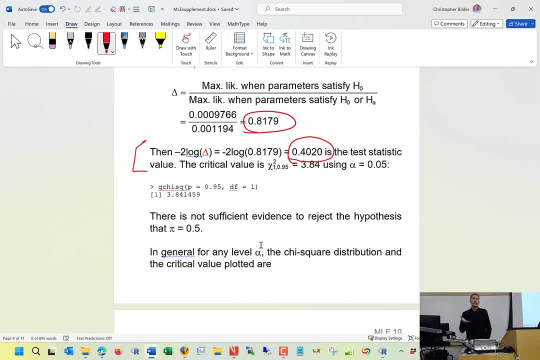 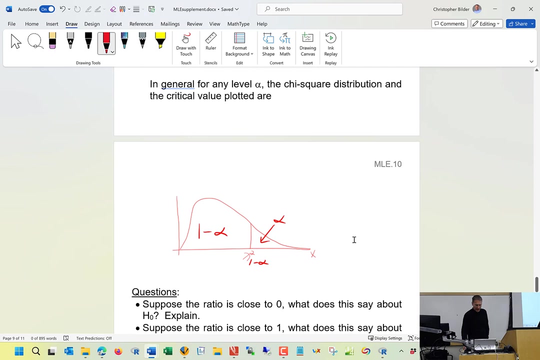 course your instructor emphasizes, we can never prove the null hypothesis to be true. if any hypothesis does So on a project or a test. If you end up saying HO is true, I will actually take off points for that. Okay, Any questions about this? introduction to a likelihood ratio test. 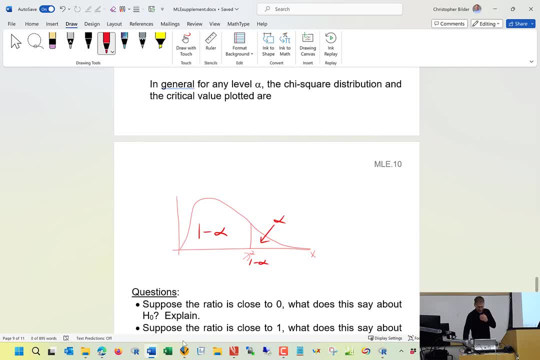 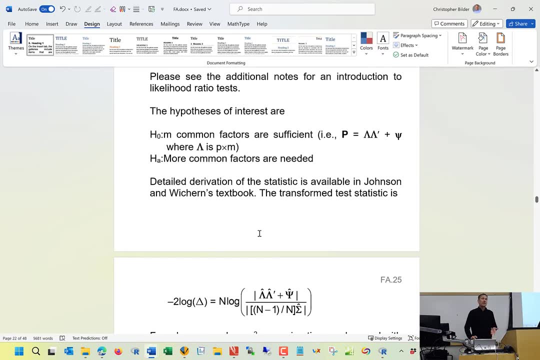 Is it intuitive, hopefully? You know just a ratio of two likelihood functions and we look to see what are our unusual values. So now, let's apply this now to factor analysis. Now our hypotheses become much more complicated. Okay, The null hypothesis is that we have m common factors. What that basically means is that you have all these corresponding lambdas. Those are parameters that we're actually testing. The alternative hypothesis is that more common factors are needed. So instead of m common factors, we need maybe m plus 1 or m plus 2 or so on. 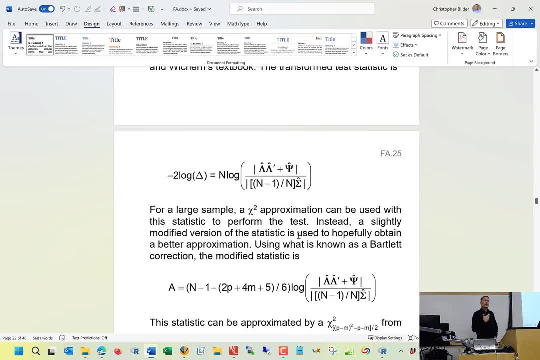 Okay, One could derive the negative 2 log delta statistic. You're not responsible for this. As you can see, it's kind of messy. in the end, We're working with a much more difficult distribution, But it's the same concept here in terms of how you can think of what this negative 2. 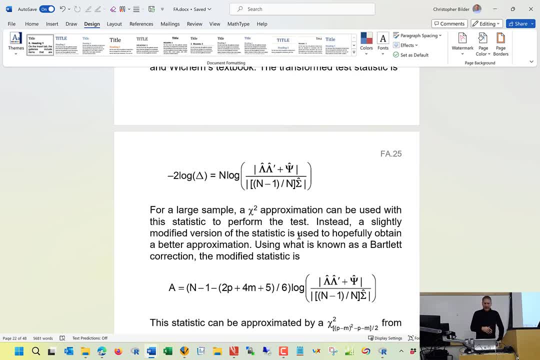 log delta is actually measuring. Now, what people who do research and statistics such as me will realize- Now what people who do research and statistics such as me will realize- is that they are able to measure a negative 2 log delta. 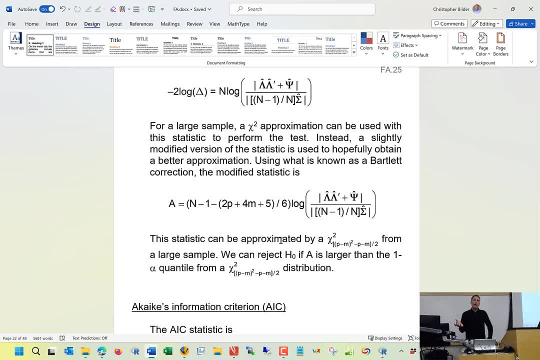 And there's a number of cases where they're able to measure a negative 2 log delta. Okay, often concerned about is: well, how well does this, in this case, a chi-square distribution approximation, actually work? and if there's cause for concern, can I get a better approximation? and so what this person by the name of Bartlett did, a 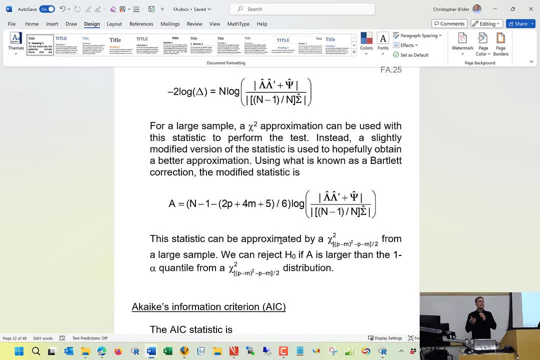 long time ago he actually did a little bit of a change to the statistic that ends up being leading to a better approximation for a chi-square distribution. so, rather than negative log Delta, exactly instead what we end up we're going to use as a statistic black of a better letter word called a and you. 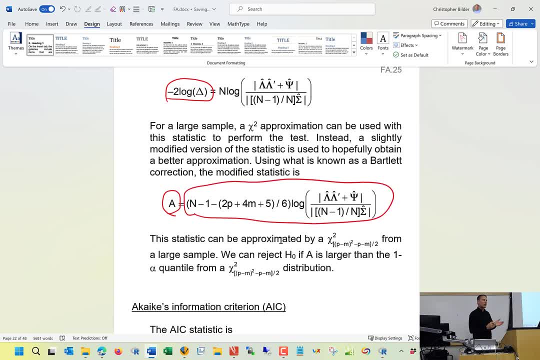 can see it looks kind of like the one that we had above, but there's some small modifications to it. remember M's. a number of common factors will be under null hypothesis. P will be the number of original variables that you have. capital. n is your sample size, of course, like Sigma. hat is your estimate covariance. 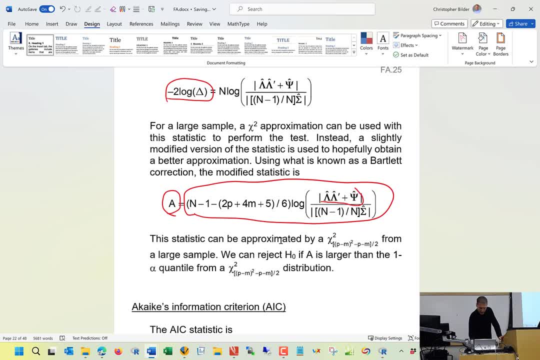 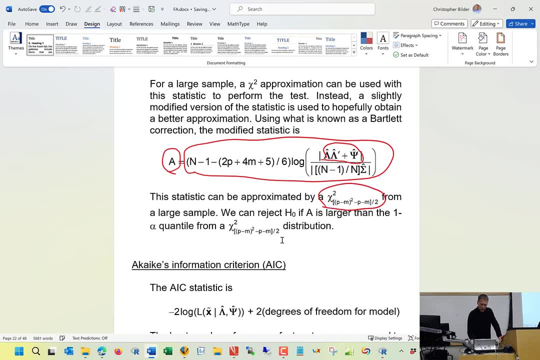 matrix and then the stuff that's in the numerator right here represents from your factor analysis model. so we end up using a chi-square distribution approximation with a. in the end there's the corresponding degrees of freedom. as you can see, it's kind of a messy expression for it, so we will apply that. 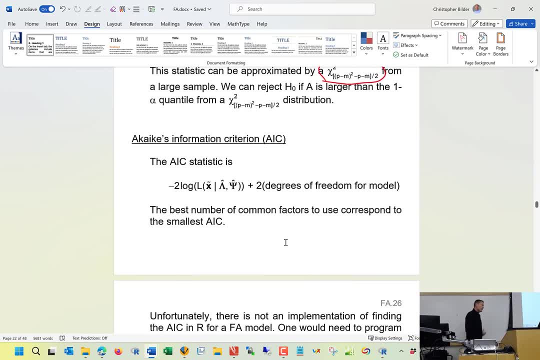 shortly now. for those of you who come in here with some experience with black hood methods, you might also know about using what are called information criteria to choose between different models. basically, the smaller the information criteria value, the better the model is, in particular the most commonly used ones. let's call it: take these information criteria, and so we. 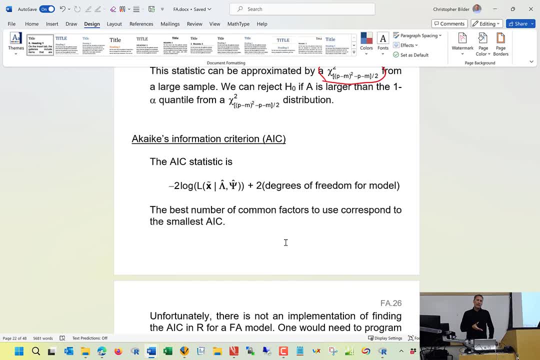 could actually form this here and say: okay, the factor analysis model relative to the number of common factors that has the smallest AIC represents the best model, the best number of common factors to choose. however, there isn't a good way to implement this in R. I've never been able to find. 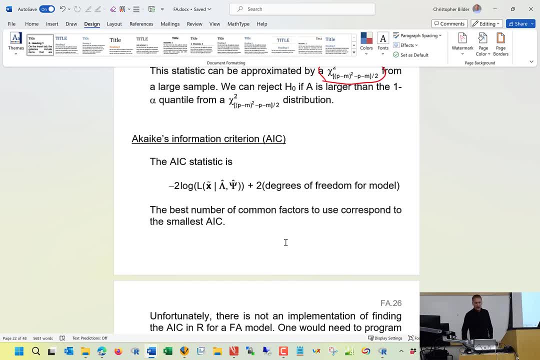 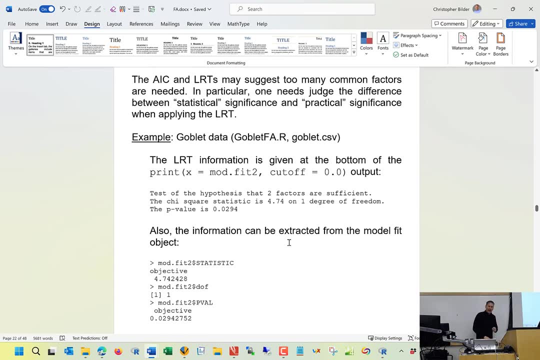 one. if you happen to find one, let me know. so I would like to use that. so for that reason, we will not look at it here. and, lastly, we need to talk about something, hopefully, that you talked about in your first act, and that is the difference between practical. 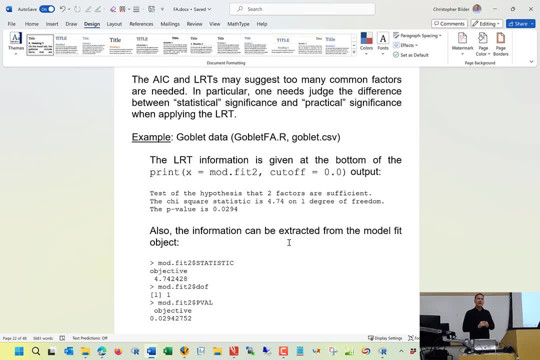 significance and statistical significance. you know, again, we relate it to this hypothesis test of mu is equal to mu zero versus mu not equal to mu zero. you know you, let's say, if you reject a show your instructor might have said, okay, we have, we have a statistically significant result, maybe like the p-value is really. 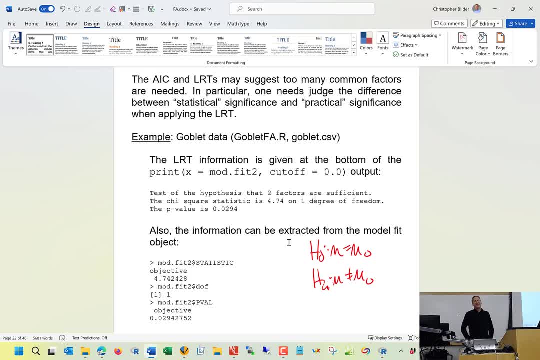 small, so we're going to call that statistically significant. the problem, though, with that is as follows. let's say this is an example- I often like to use an introductory class. let's say that I'm interested in doing a hypothesis such as this, where I'm interested in the mean GPA of all students here on campus. I 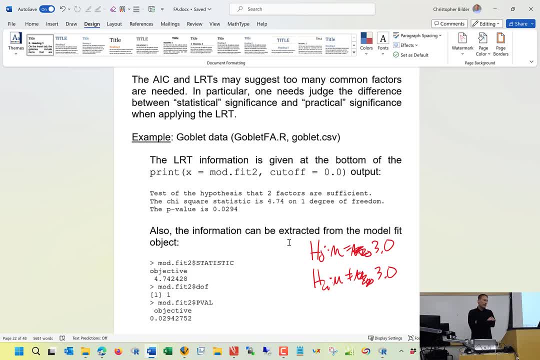 don't have access to all the student records, that would be like in the Registrar's office. instead to take a sample, I would need to actually, let's say, add a sample of the GPA of all students. that would be in the Registrar's office. instead to take a sample, I would need to actually, let's say, add. 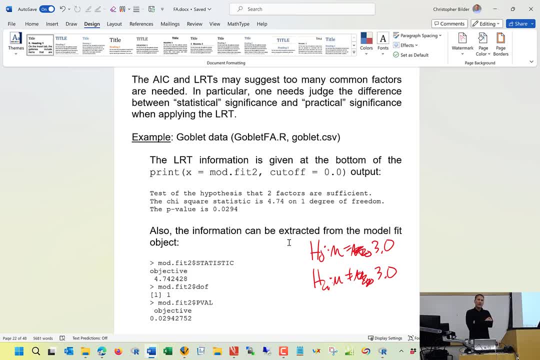 maybe a hundred students. what is your GPA? Based upon that, I do a t-test. to do the hypothesis test. Let's say I reject HO. I have a statistically significant result, But let's say that I can now, let's say, access all student. 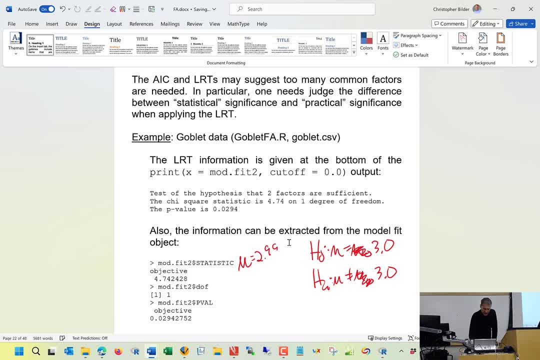 records like 25,000 students here on campus, And I find out that the true mean GPA is 2.999999.. Okay, so even though I had a statistically significant result, is this practically significant? No, And that is a problem with hypothesis testing. 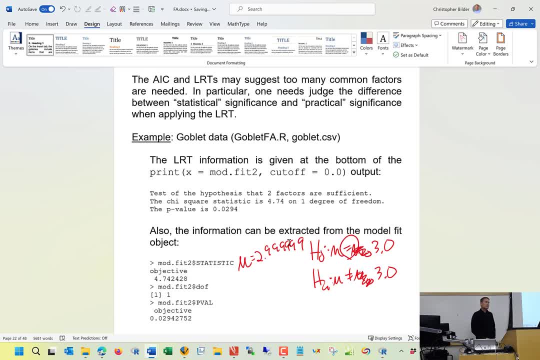 Especially when you have like an equality here. I can typically find a sample size. If I'm allowed to go as high as I want, then I'm going to get it in the end. get a p-value that's less than .05.. Because it's so hard to be exactly this. 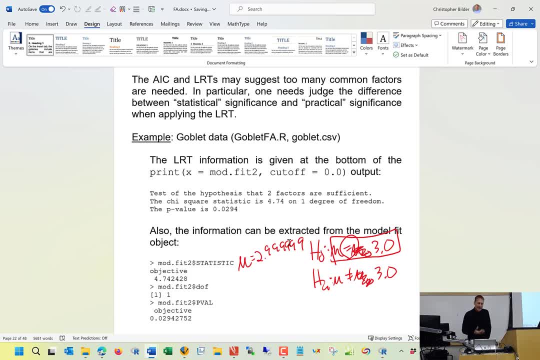 And so, in the end, what ends up happening with these likelihood ratio tests is that they can actually lead to a situation where it says: you need more common factors when, in a practical sense, you don't. How do you judge what's practical? Well, you don't. 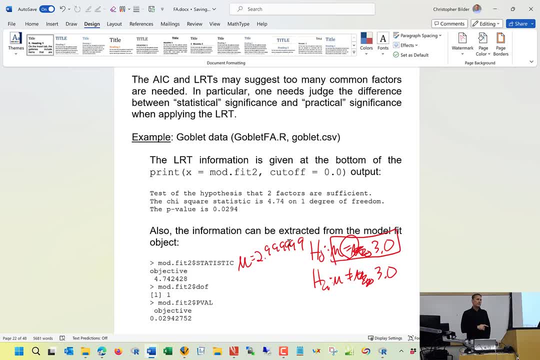 That's where you look at those residuals. You know, if I, let's say, did a hypothesis test and said, hey, you should have more common factors. But then I look at the residuals and all the residuals are, let's say, less than .05.. Now I might be thinking, oh, wait a second here. I think this model does an. 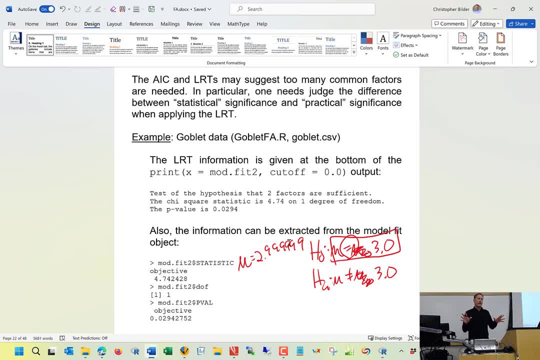 adequate job still, And so, even though the hypothesis says you need more common factors, I can go against it. So think of this likelihood ratio test as one tool in your toolbox for deciding how many common factors to use, But don't necessarily say I have to go exactly by that. 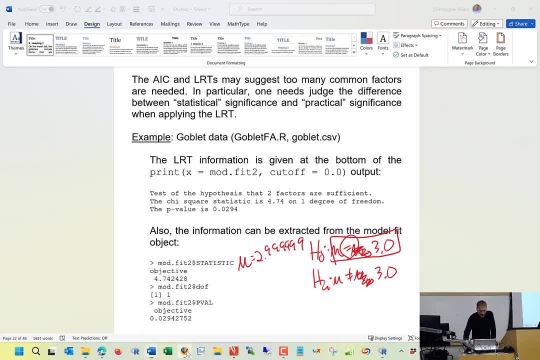 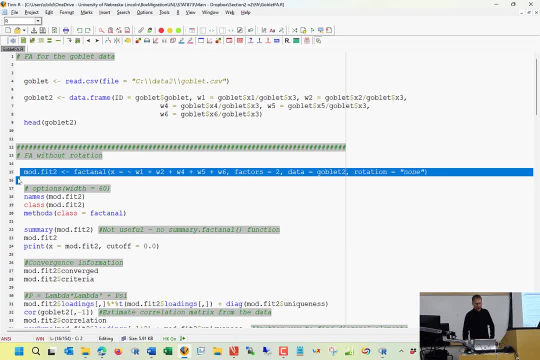 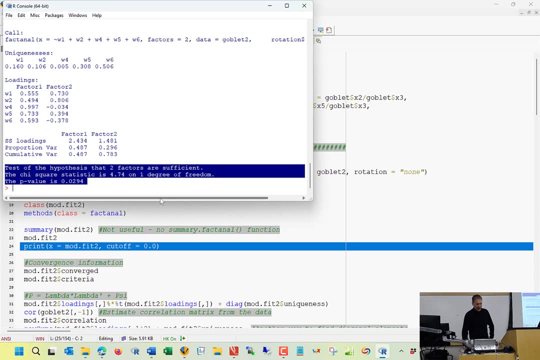 Ok, so let's now apply this to the GALA data. So again, I can use FactAnno to estimate the factor analysis model. When I use the print function with the corresponding results at the very end of the output is where I get the information about the likelihood ratio. 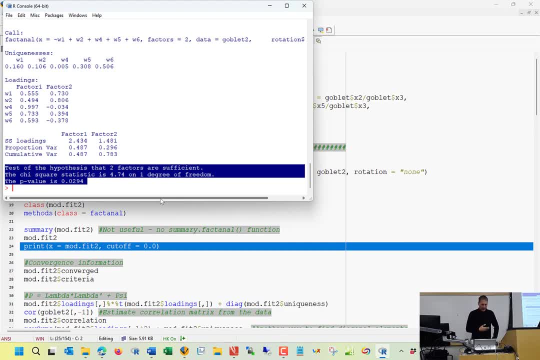 test, And so notice that R says tests the hypothesis that two factors are sufficient. That's Ho Ha would be more than 2.. The chi-square statistic value is 4.74.. That is our aim. Let me actually write that down. 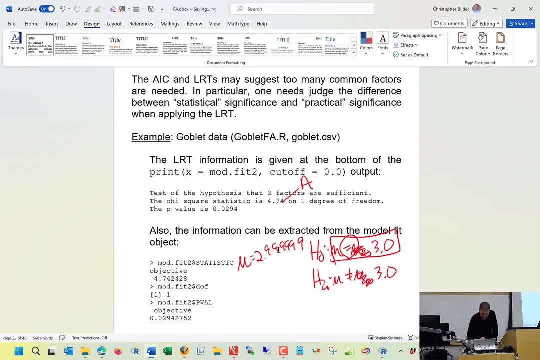 So this is our A. Two factors are sufficient, essentially our HO P value of .0294.. So should I reject or don't reject HO? Well, you know, depends upon what algorithm you use And what we've, over the last five to ten years in statistics, have tried to emphasize, to. 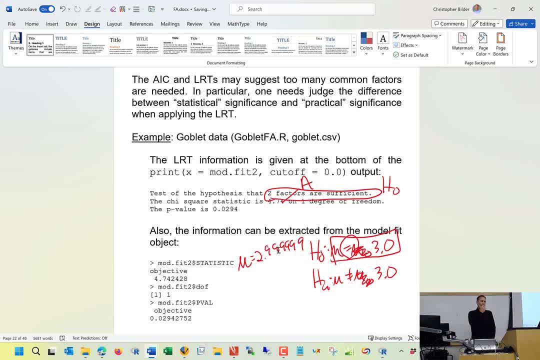 students is that you got to be careful there about using a strict- let's say .05- cutoff. You know, because if I use .05 as my alpha level, I would reject. It would say more common factors are needed. But if I use alpha .01, I would say: don't. 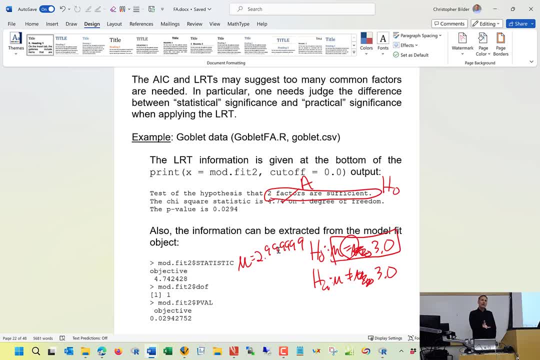 reject HO. So in these particular situations it's best to say: well, there's marginal evidence to suggest that more common factors are needed. It's not strong, it's marginal, And that's the way that hypothesis testing was originally when. 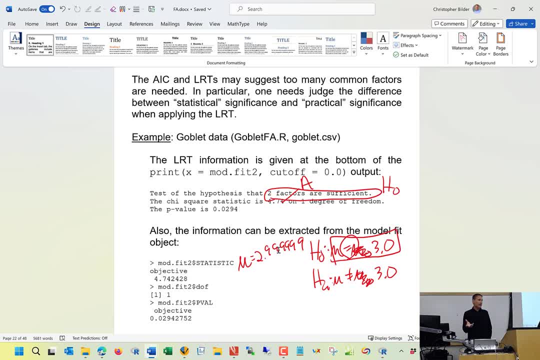 it was first developed was meant to be interpreted as: Unfortunately, over the years, people got away with it and they chose strict guidelines. You know, if I had, let's say, a P value of .049,, hey, that's great. I reject If I have a P value of .051,. 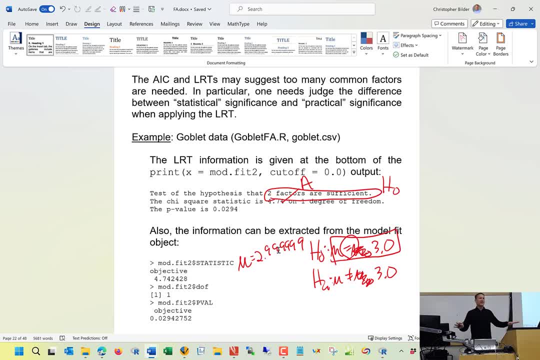 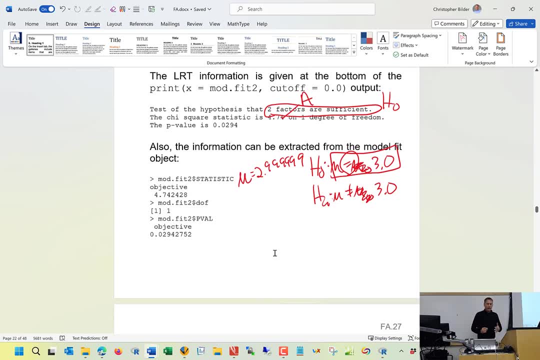 oh, then I don't reject. Oh no, it should be exactly the same interpretation. You have marginal evidence? Okay, Now, if you want to, you can go inside a modfit2.. Remember, that's a list. type of object: an arm, And I can extract out statistic. Here is my A. I can also. 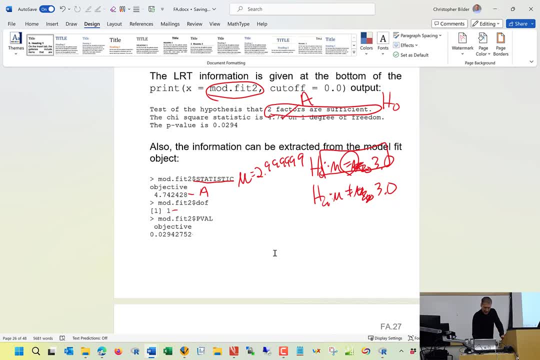 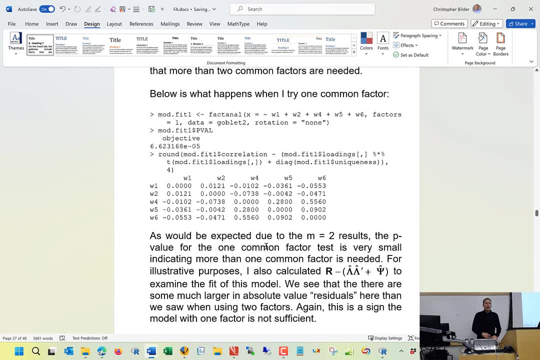 extract out the degrees of freedom, which ends up being 1.. And I can also extract out the P value as well. Okay, So we have marginal evidence, Just .049, Based upon this, that maybe more common factors are needed Before we look at more common. 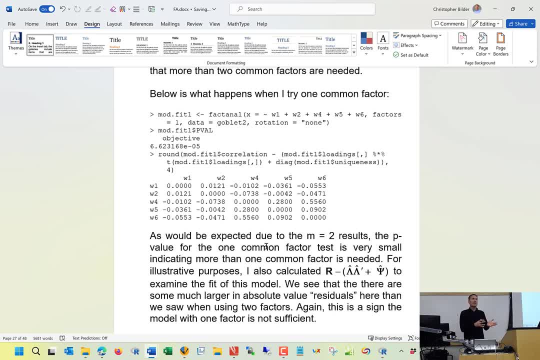 factors, though, how about we look at just one common factor and see what happens? Now? you would expect in this situation, all right, the P value to be smaller, because 2 is kind of marginal, And if I'm only using 1, then you might say, okay, I don't know if I maybe. 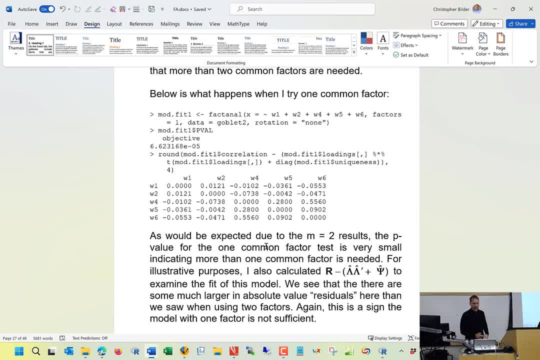 2 is not working. I doubt 1 would work, And so what would happen if I use 1? So I say 1.. Here's my P value. It is much smaller. One reason why I want to show you this is: 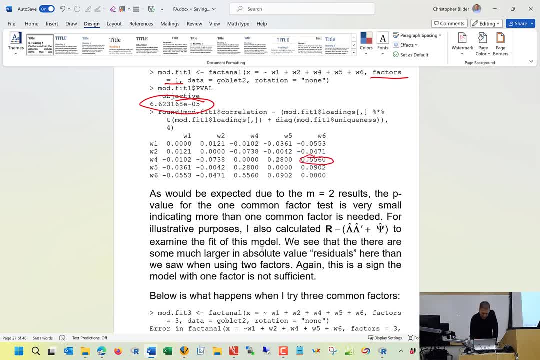 take a look at this, Look at the residuals. So I use the same matrix algebra tools as what we saw before to find those residuals. Look how big in absolute value those residuals are. This is a big warning to you that hey, this factor analysis model with only 1 common 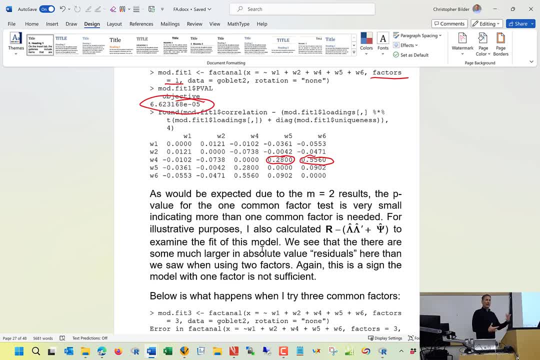 factor is just not going to work, And so I'm going to use this one And I'm going to use not sufficient. So this is a good illustration of how those residuals are kind of matching up with what the p-value is representing. Well, what if I? 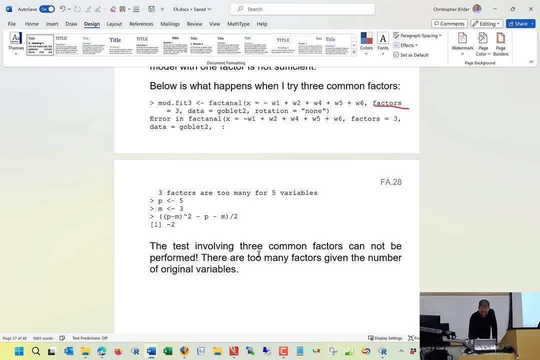 use three common factors. So I say factors equal three, and the graduates there. Three factors are too many for five variables. This corresponds to some stuff that we were talking about last time, where you can have, let's say, multiple solutions, That's it, And so I can't even use two. I can use one, I can use two. 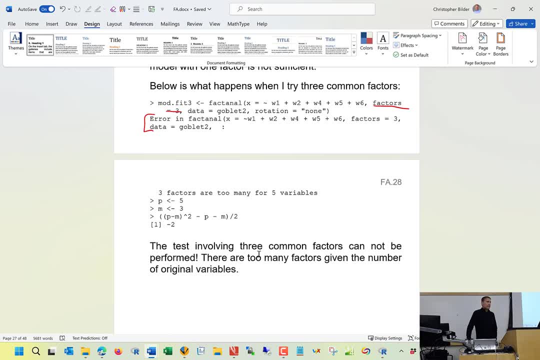 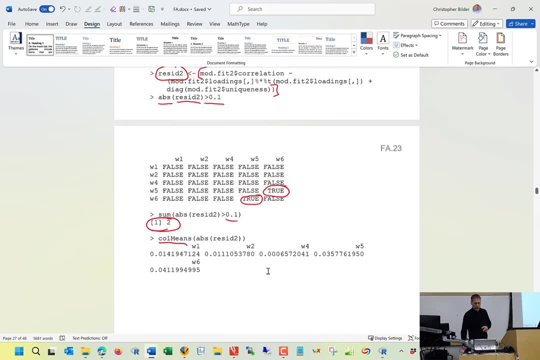 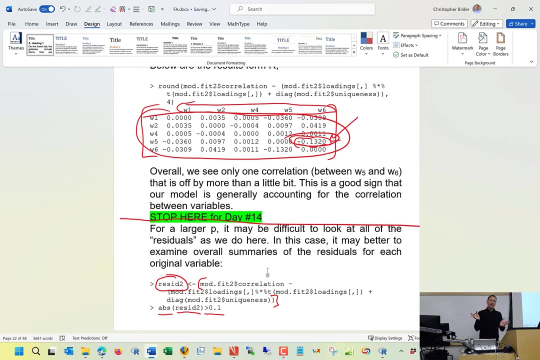 Two is definitely better than one. And from a practical context again, if I go back to my residuals for the two, you know in only one case where there's maybe a little bit of concern, but it really wasn't that much, And so, based upon this, I'd be satisfied with two common factors. I wouldn't really have a problem with these. 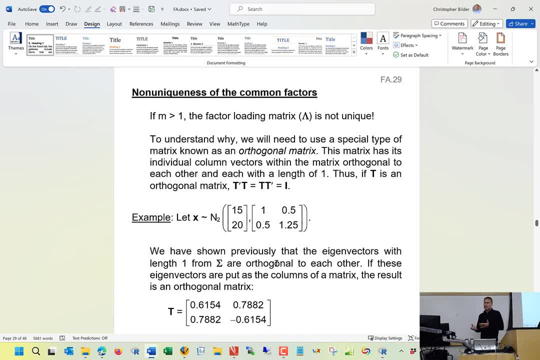 So you know like, for example, if I had a question that I wanted to answer, I would go back to my residuals, But for your own, as you will see for project number two, you're going to need to apply factor analysis to your data that you use for. 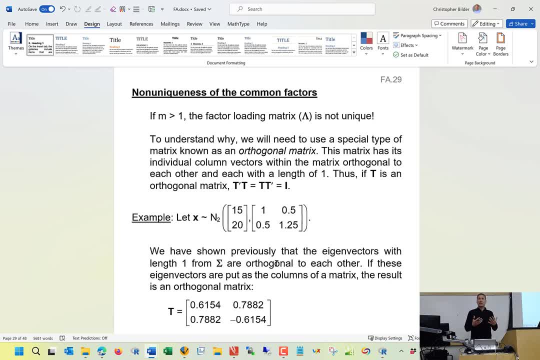 project number one, And one of the questions will be how many common factors are needed, And so you're going to need to do some like hypothesis tests. look at the residuals to make that judgment. Now you might be wondering: okay, well, where's a? 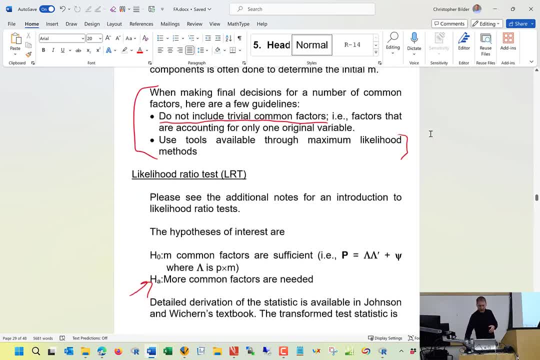 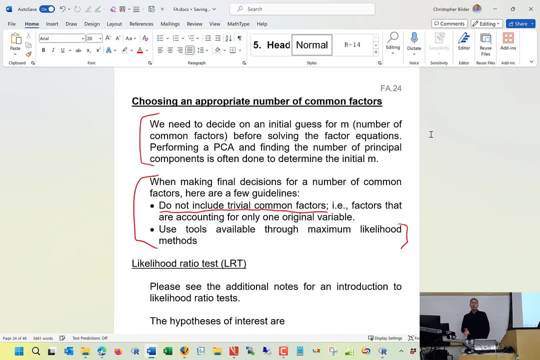 good place to start in terms of the number of common factors, And I, unfortunately I did skip over that. You know, where I would start is look at your principal component analysis. how many principal components you chose. Why don't you start with that first, as the 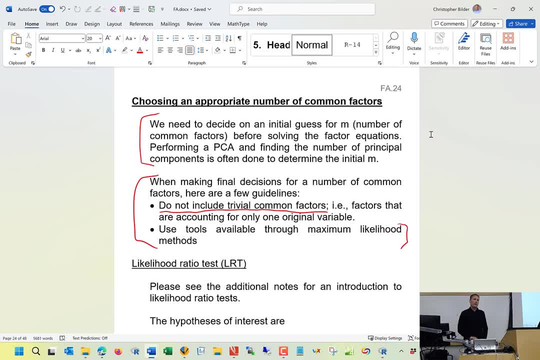 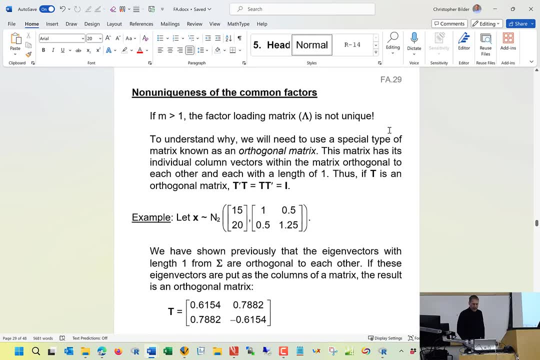 number of common factors, see how well that does and adjust accordingly. So this next set of notes talks about the non-uniqueness of the common factors. This is both a strength and the problem with using factor analysis. This is what's going to allow you to have multiple different 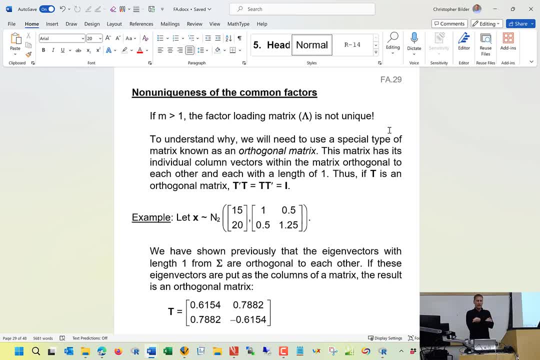 interpretations for what your common factors represent. That's why this is called non-uniqueness of the common factors. To help understand why this occurs, we need to introduce what's called an orthogonal matrix. so we've talked about orthogonal vectors before, so if I have 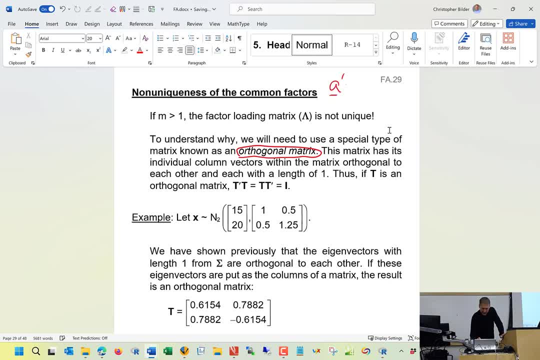 let's say a vector a- if I take the transpose it times- a vector B, and let's say these vectors are orthogonal to one another. what's the end result here? zero in the geometric sense you can think of like how the x-axis on a two-dimensional 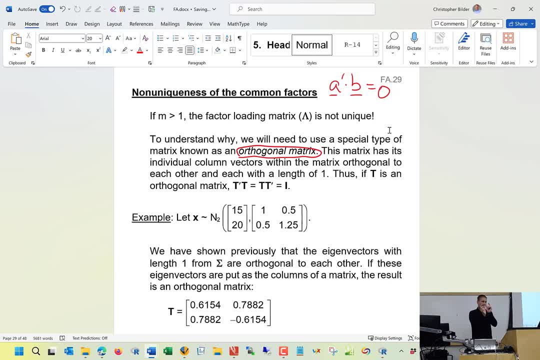 plot and the y-axis on a two-dimensional plot, how they're perpendicular to one another. that's what basically this idea of orthogonality represents. now suppose I form a matrix T of orthogonal vectors as the column. so maybe, for example, here's my matrix and I'm just going to put a here and B here to represent first. 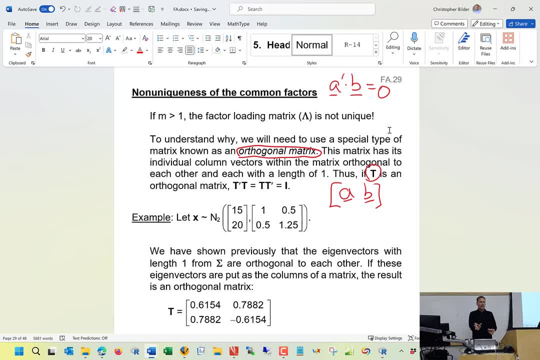 columns and ends. the first column is A, the second column is B. This is going to be like my T matrix. Now, if I were to take T, transpose T and multiply it all out, I will get the identity matrix back. Why? Well, the off diagonal elements will be basically what? 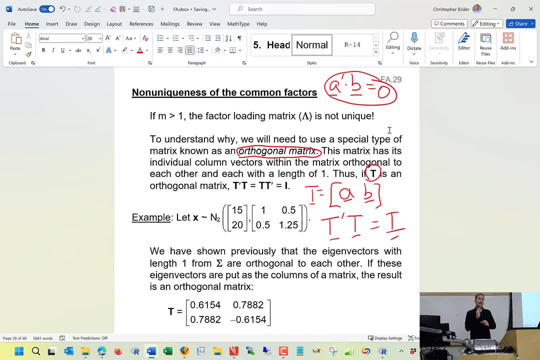 happens here. The diagonal elements would be like A transpose times A- and something that I failed to mention as well- because each of these orthogonal vectors have a length of one, And so if I take A transpose times A, I will get one, So 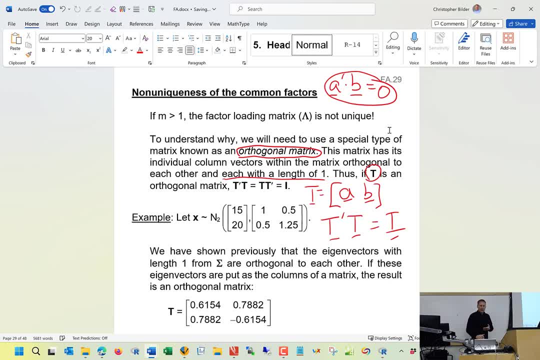 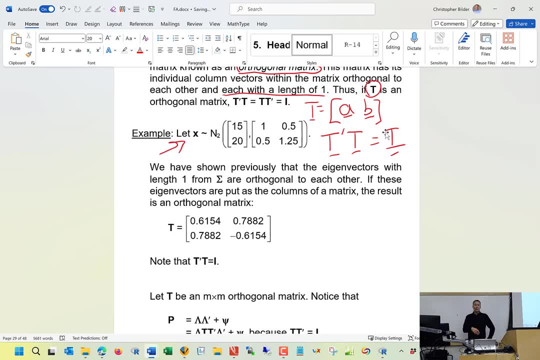 that's why you get the identity matrix back. A little example: back in the data distributions and correlations section we looked at this bivariate normal distribution. we found the corresponding eigenvectors for the covariance matrix. so here was one eigenvector, here was the second. 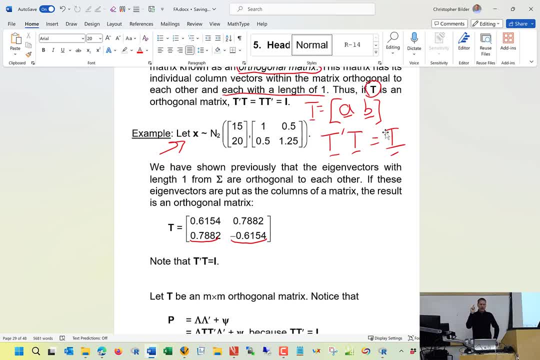 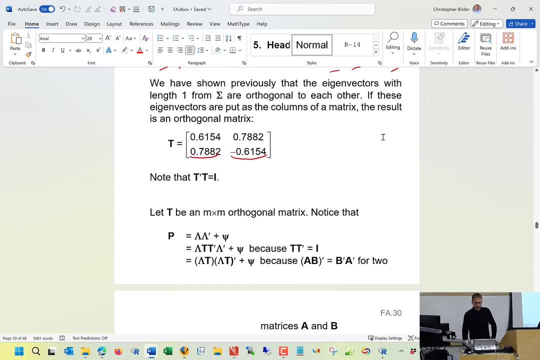 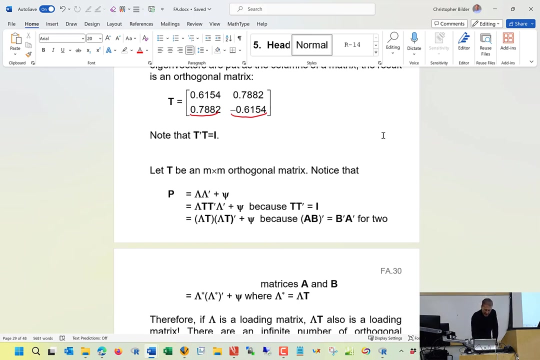 eigenvector. and if you were to actually take T, transpose times T, you get the identity matrix right on your okay. so where does this orthogonal matrix then come into play here? factor analysis: well, let's take a look at our factor analysis equations. so, based upon our factor analysis model, our correlation matrix. 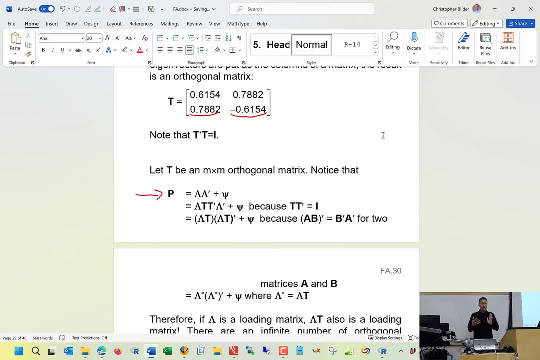 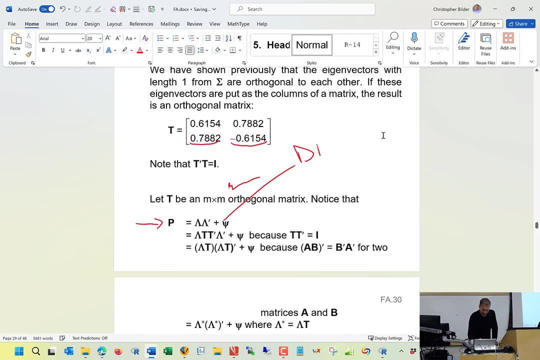 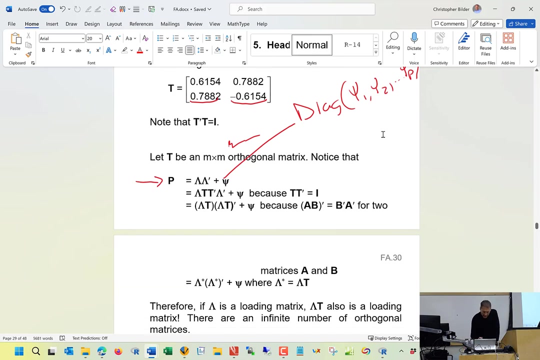 can be written as: lambda active loading matrix times, lambda prime plus psi. you remember what psi is the diagonal matrix where I have, let's say, psi 1, psi 2 down to psi P on the diagonal. these are the specific variances, the variances of the specific factor. now I'm going to do a little bit of a. 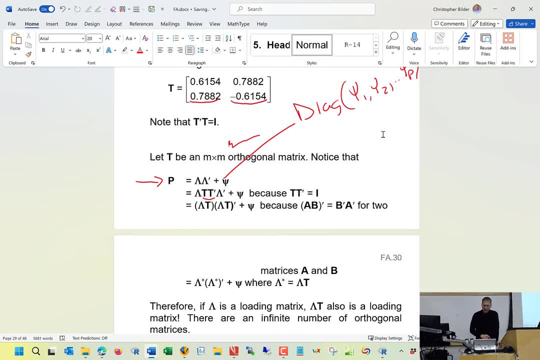 mathematical trick here. suppose I put here- I'm going to do a little bit of a mathematical trick here- suppose I put T in T prime, right between these two labels. this doesn't change anything, because T times T prime or T prime times T is equal to the identity matrix, the. 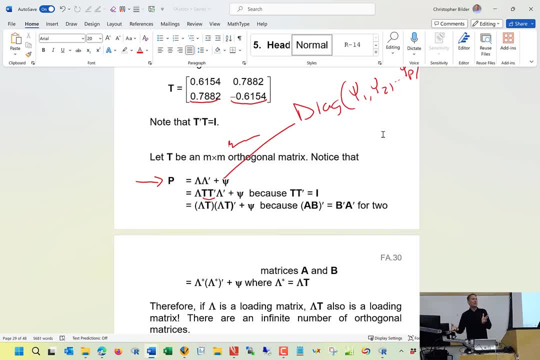 identity matrix times any other matrix. is that any other matrix back? so nothing changes. but what I can do is rewrite some stuff. now suppose I put lambda and T together and I put lambda and T together and I put lambda and T together and then notice I have a T prime times lambda prime. well, again, using some 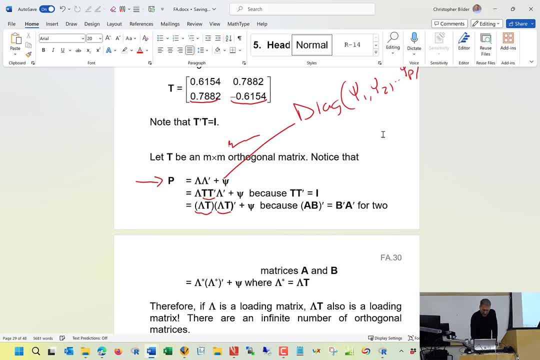 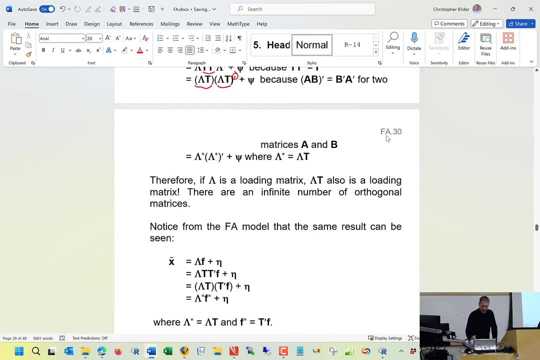 matrix algebra results. I can rewrite this as lambda T, that whole thing transposed. and how about we just redefine some stuff? so let's let lambda star now be my lambda T, and so I get back to where I was before, kind of with my. and so I get back to where I was before, kind of with my. 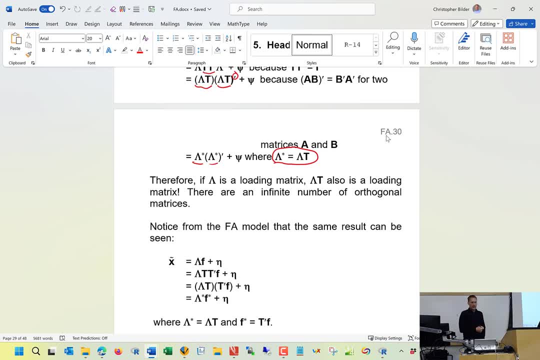 original factor analysis equations. we original factor analysis equations, we original factor analysis equations. we just have a little star there and so just have a little star there and so just have a little star there. and so essentially all I've done is now preserve. essentially all I've done is now preserve. 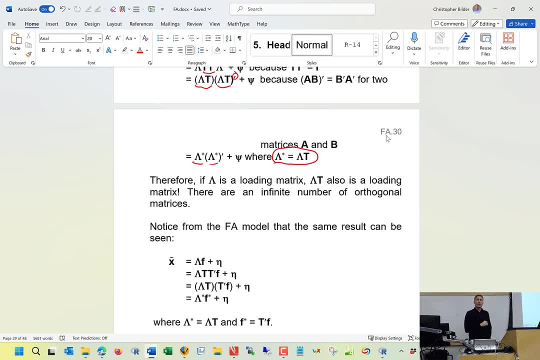 essentially all I've done is now preserve the equality there, but now I have a new the equality there. but now I have a new the equality there. but now I have a new set of factor values. that's all don't. set of factor values, that's all don't. 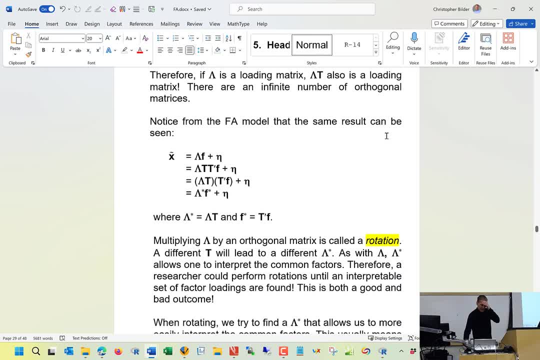 set of factor values, that's all. don't see that a little bit better. let's look, see that a little bit better. let's look, see that a little bit better. let's look at this from the perspective of a, at this from the perspective of a, at this from the perspective of a factor-analysis model. for some reason, I 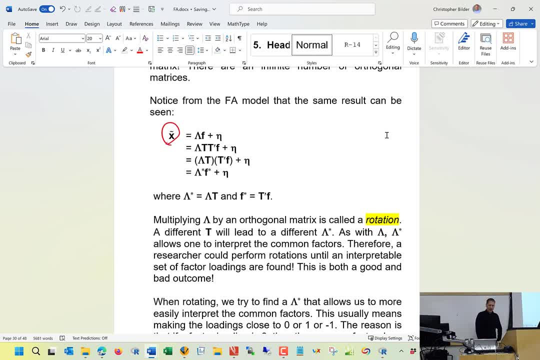 factor-analysis model. for some reason I factor-analysis model. for some reason I decided to put next to me that you can, decided to put next to me that you can, decided to put next to me that you can. let's see there if you really wanted to. let's see there if you really wanted to. 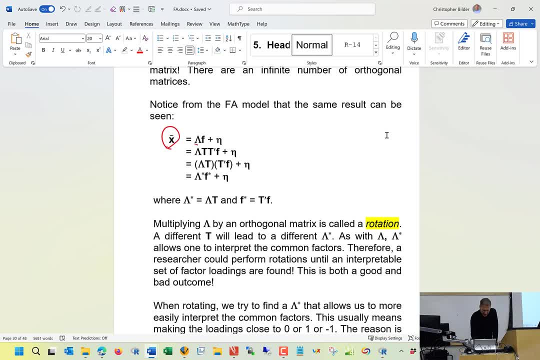 let's see there if you really wanted to. so X tilde is equal to lambda times F. so X tilde is equal to lambda times F. so X tilde is equal to lambda times F plus 8. I've written them all in terms of plus 8. I've written them all in terms of. 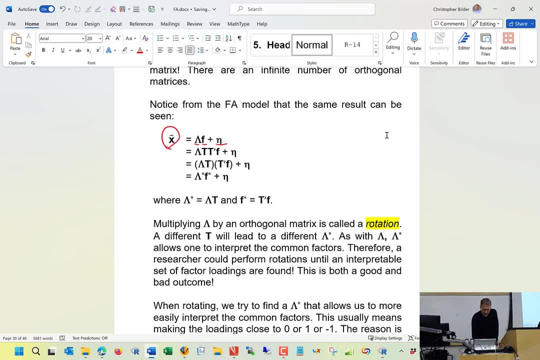 plus 8. I've written them all in terms of matrices. let's put my TT prime in there. matrices: let's put my TT prime in there. matrices: let's put my TT prime in there, and that doesn't affect anything. I and that doesn't affect anything. I. 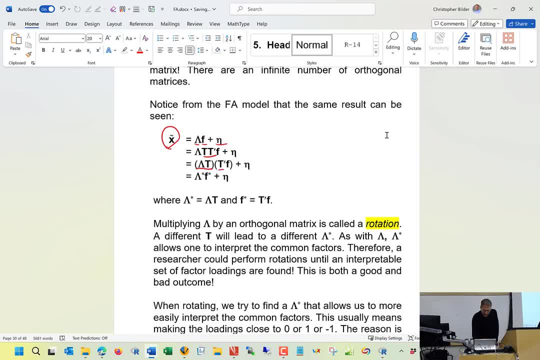 and that doesn't affect anything. I reorganize some stuff, so I have a lambda reorganize some stuff, so I have a lambda reorganize some stuff, so I have a lambda T. I have a T prime F now as well, and T. I have a T prime F now as well, and 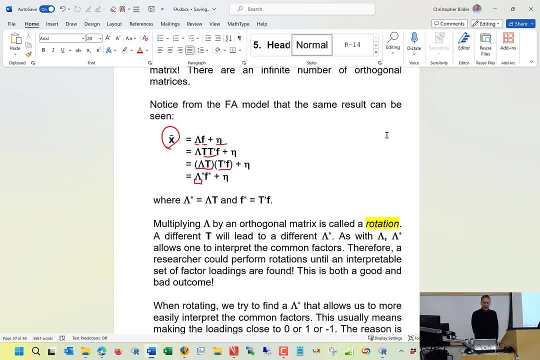 T. I have a T prime F now as well, and how about we just say, okay, we'll call that? how about we just say, okay, we'll call that? how about we just say, okay, we'll call that lambda T, lambda star, and we'll call lambda T, lambda star, and we'll call? 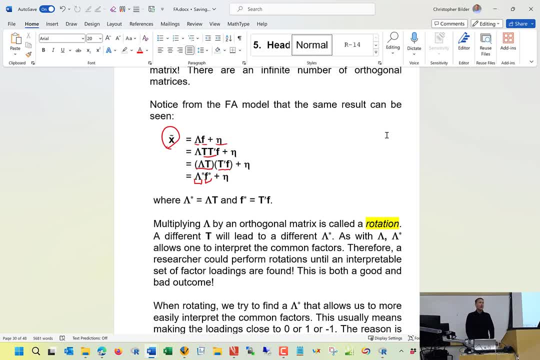 lambda, T lambda star, and we'll call T prime times F F star. and now I have T prime times F F star, and now I have T prime times F F star. and now I have this new model. these F stars are a new. this new model, these F stars are a new. 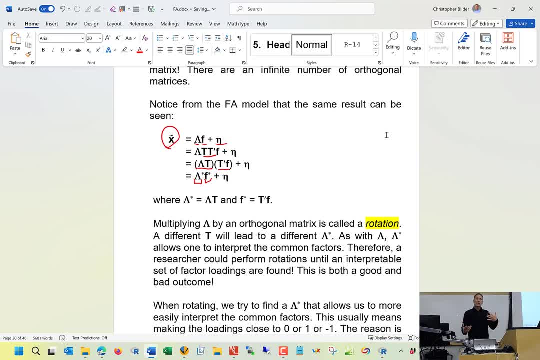 this new model, these F stars are a new set of possible common factors. we use set of possible common factors. we use set of possible common factors. we use the, the, the quantities inside of lambda, the, the quantities inside of lambda, the, the quantities inside of lambda star. to now try to interpret this: 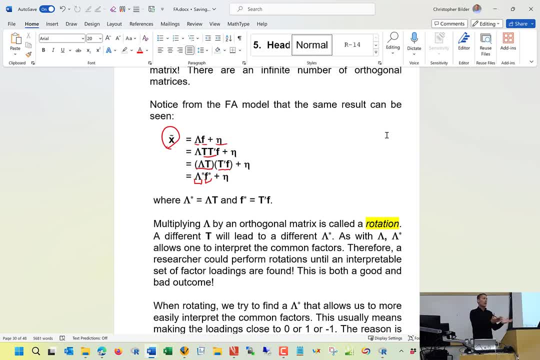 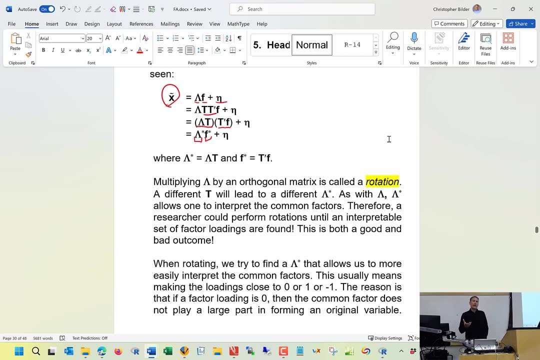 star. to now try to interpret this star. to now try to interpret this interpretation will likely be different. interpretation will likely be different. interpretation will likely be different from our original lambda already. so what from our original lambda already? so what from our original lambda already? so what we see here is that we have nine unique 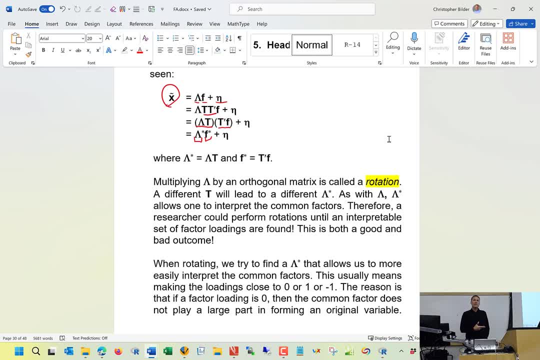 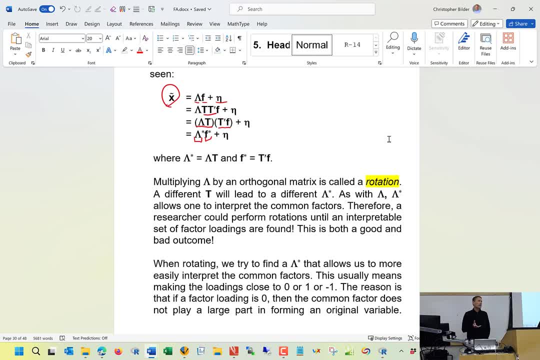 common factors. in fact, there are many, many, many more different of these team, many, many, many more different of these team. many, many, many more different of these team matrices that I could use and I can matrices that I could use and I can matrices that I could use and I can get different common factors in the end. 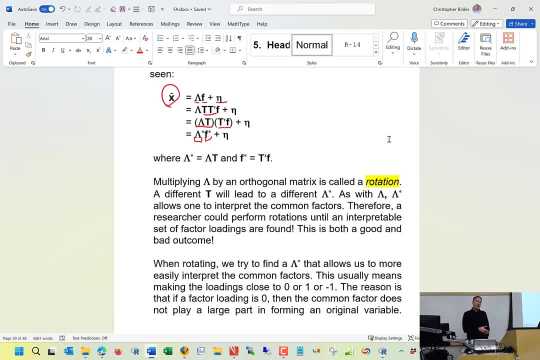 get different common factors in the end, get different common factors in the end. this, hopefully maybe is setting off some. this, hopefully maybe is setting off some. this, hopefully maybe is setting off some alarm bells- that okay. so you're saying alarm bells, that okay. so you're saying: 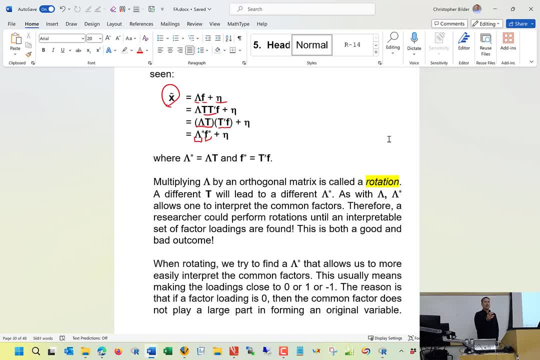 alarm bells that okay. so you're saying that I could get different common, that I could get different common, that I could get different common factors? I had many different common factors. I had many different common factors. I had many different common factors. sent you as I want, yeah, that's. 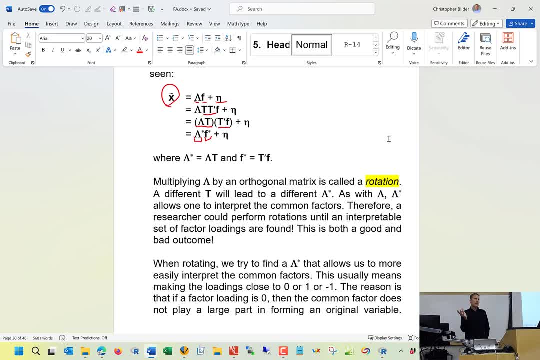 factors sent you as I want. yeah, that's what I'm saying. If I have different common factors, I have different interpretations of my data. This is the number one problem that people have with factor analysis because of this: The non uniqueness of these common factors. But 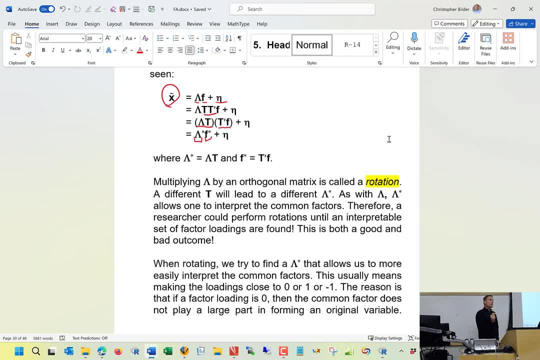 this is also what other people say is a strain, Because maybe I could choose my t in such a way that I can come up with an easier interpretation of my common factors. We'll see that as we go along Now this idea of choosing a different t. 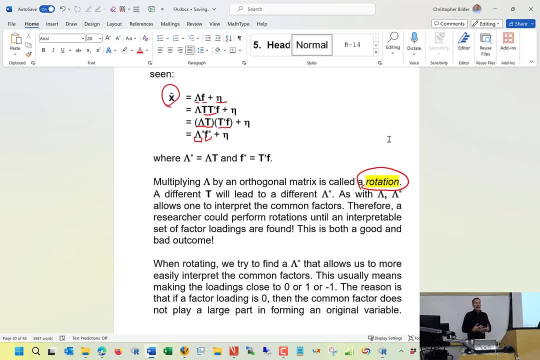 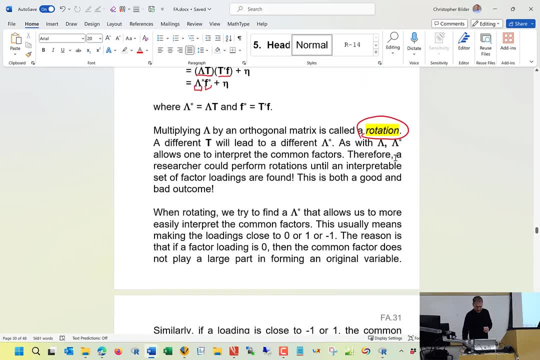 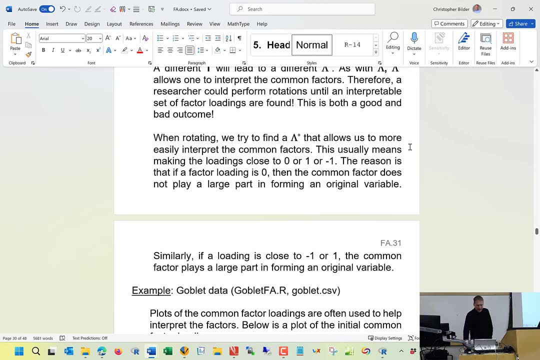 is what's often referred to as a rotation, And that's because there can be actually a geometric interpretation of exactly what we're doing here. I show that a little bit later coming up Coming up, And the idea here is that if I have different common factors, I can choose my t in such a way that I can come up with an easier interpretation of my common factors, And that's because there can be actually a geometric interpretation of exactly what we're doing here. I show that a little bit later coming up And the idea here is: 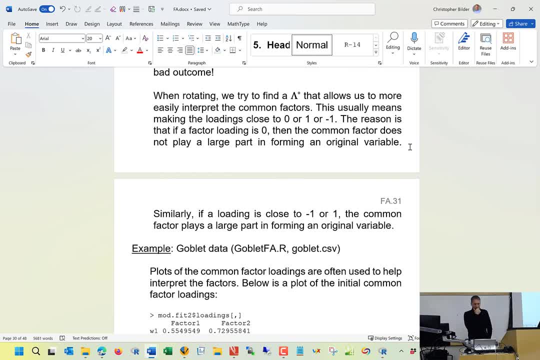 to try to choose a t such that the values that are inside our lambda starts, which control our interpretation of the new common factors. try to choose those values such that those values are either close to 0,, close to 1, or close to. 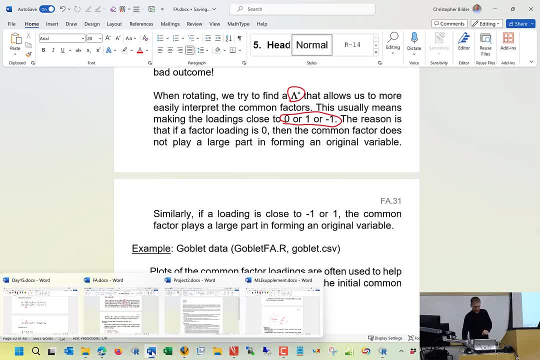 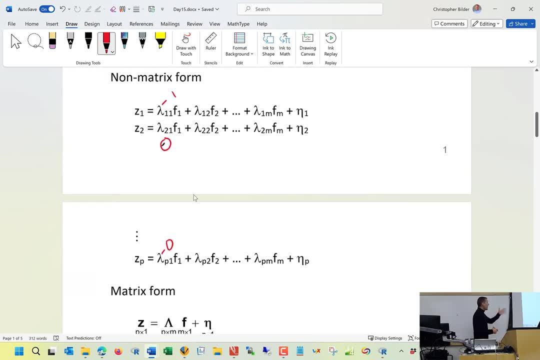 negative 1.. But why? Let's go back to back to our original model. So focus on the first common factor. If all my lambdas were 1, negative 1, or 0, that would really help me interpreting what f1 is in terms of the z's, And so that's why we want to try to choose a t such. 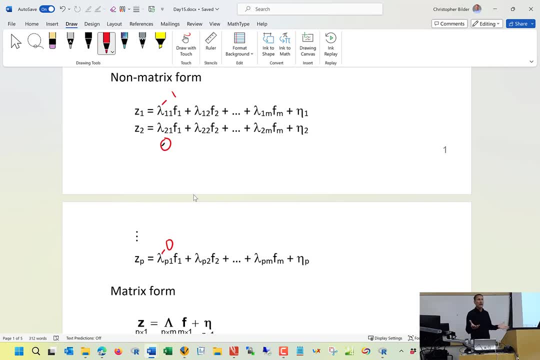 that that can happen or get as close as possible to that happening, Because otherwise, if I have, let's say, some lambdas that are 0.2, some lambdas that are 0.8, some lambdas that are negative 0.2, some are negative 0.5, it just kind of. 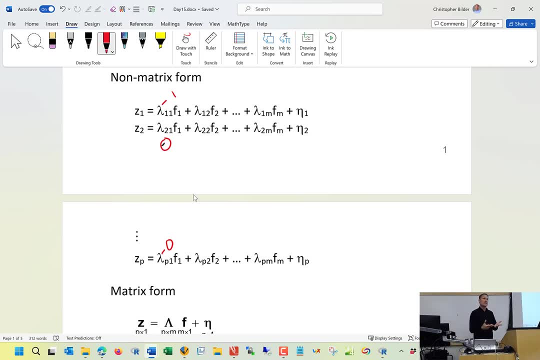 jumbles up interpretation, But especially if we can get some that are essentially close to 0. That means, you know, if lambda 2, 1 was 0, that would say, okay, z2 has nothing to do with f1.. That's okay. that makes it a little bit. 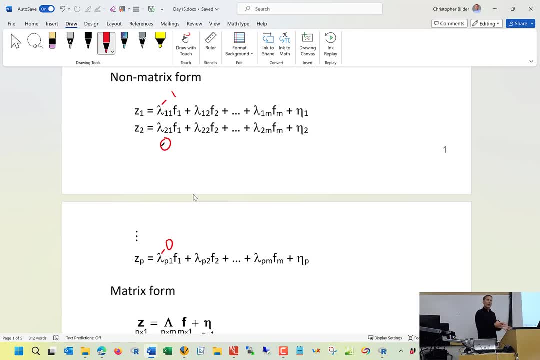 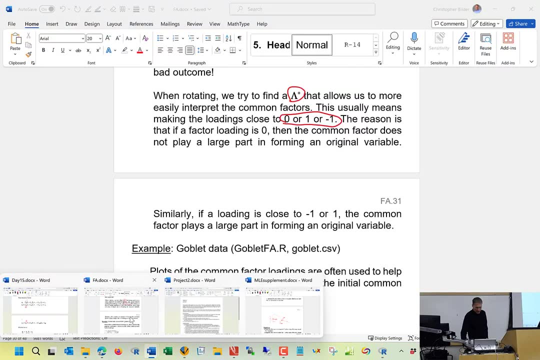 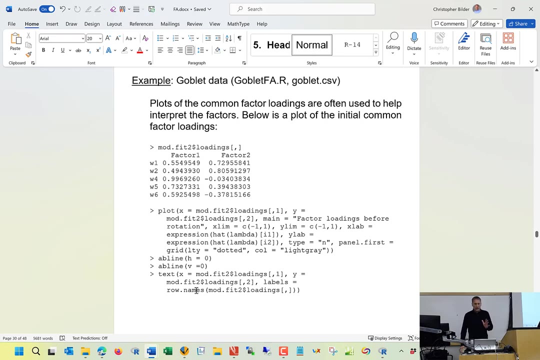 simpler than to interpret what f1 is. That's what we want to try to get, Okay, Okay. So to give you a brief geometric interpretation of this, let's go back to the goblet data. So here's our factor loading matrix. So this is our original. 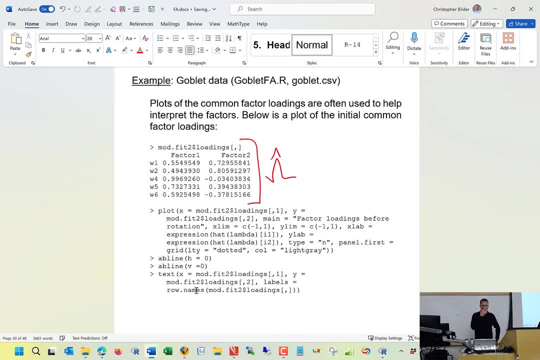 let's say lambda hat- We've extracted that before- And let's say, if I, let's do a plot of these factors, factor loadings, estimated factor loadings, that is. And so all I'm going to do for my x argument for plot, just take that first column, So that will be. 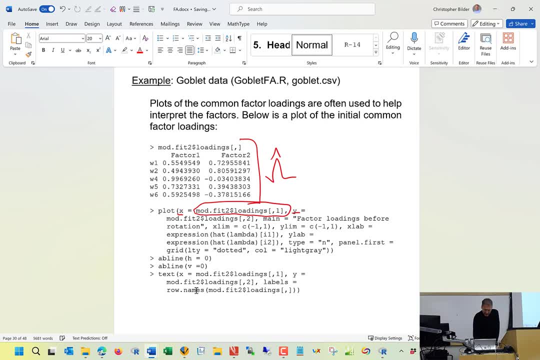 corresponding to the first factor. Y-axis is going to be my second column. of the factor loading matrix, I'm going to say type equal n- I think we've seen this before- Which basically says don't put any plotting points in the first column. 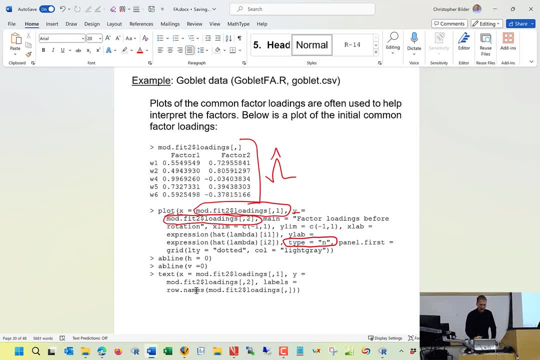 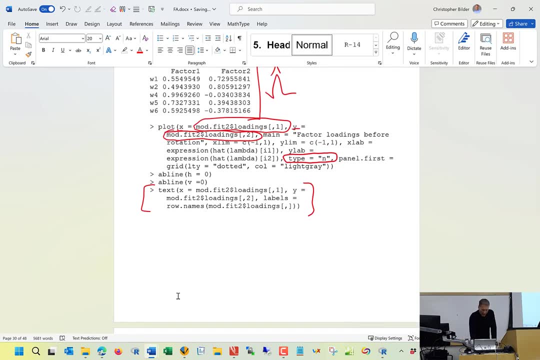 Put some plotting points on there. I actually googled, put some plotting points on there using my text function that we've seen before. Where am I going to plot these? these like just regular old texts. Well, exactly at where the factor loadings are, And I'm going to. 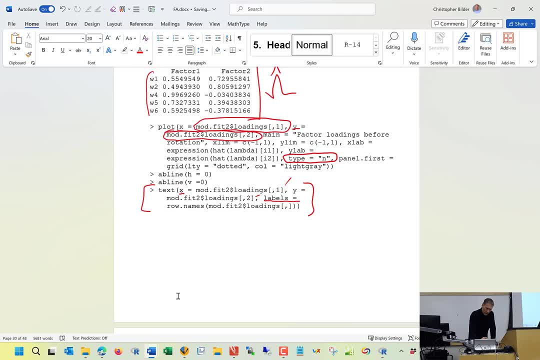 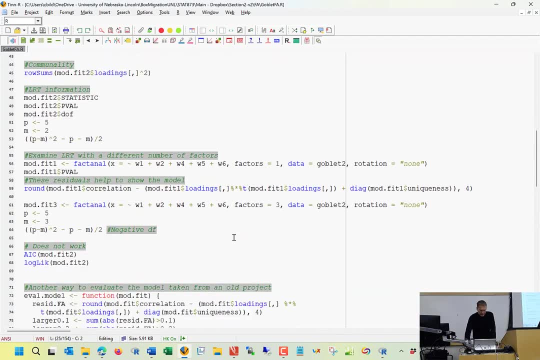 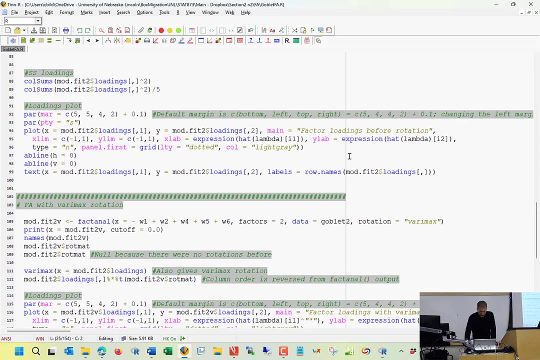 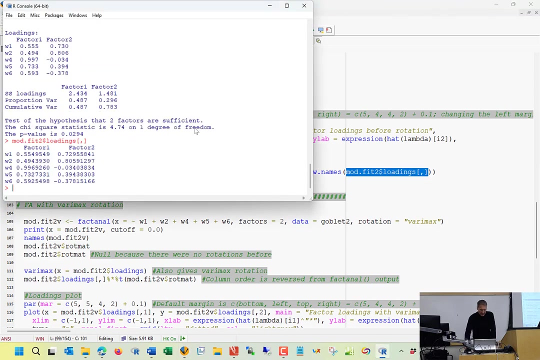 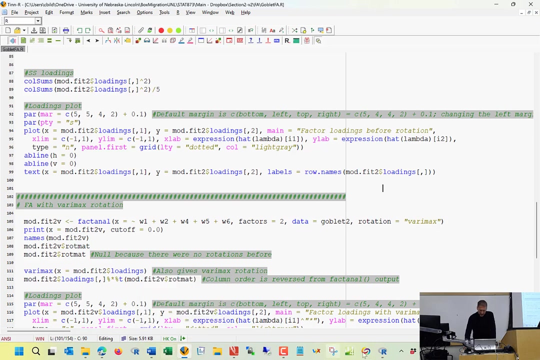 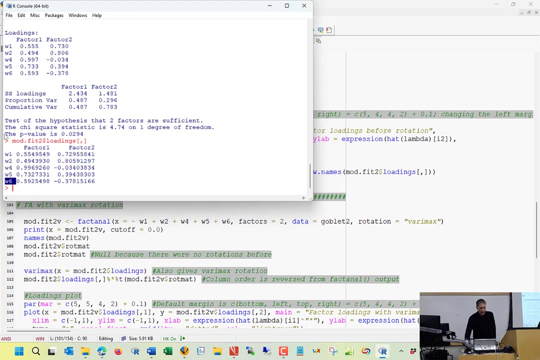 plot labels corresponding to these row names in my matrix, And so that rownames is a function we have not seen before. So here again are those estimated factor loadings. Notice how R has put basically some names associated with each row. Notice you don't see anything above. 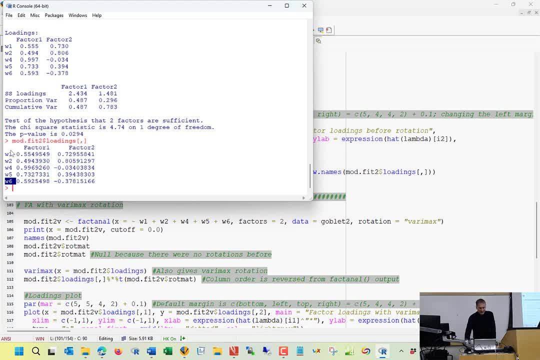 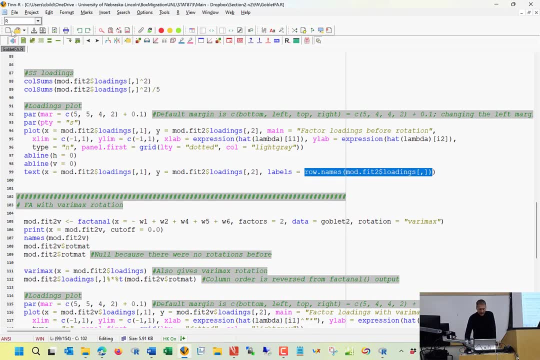 So it's not an actual variable in this. It ends up being a matrix, And so the way I can extract it is use a function that's intuitive rownames, And I get w1, w2, w4, w5, w6.. 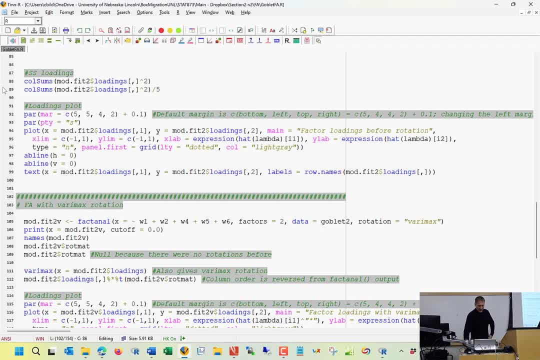 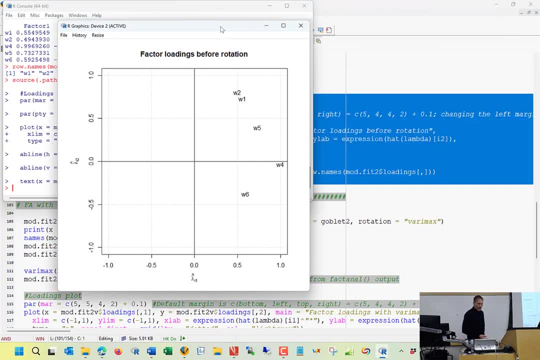 Okay, I'm going to use those as labels then when I do my plot And this is what I get. So on the x-axis, I have the lambda hat corresponding to factor 1.. Y-axis, I have the lambda hat corresponding to factor 2.. 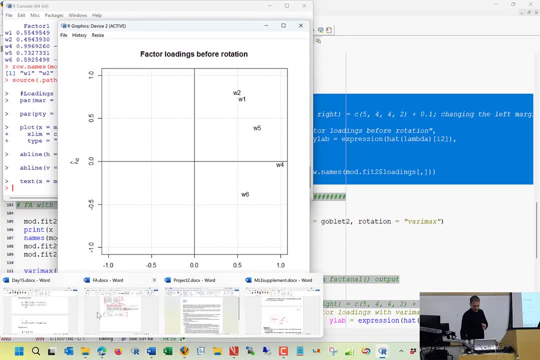 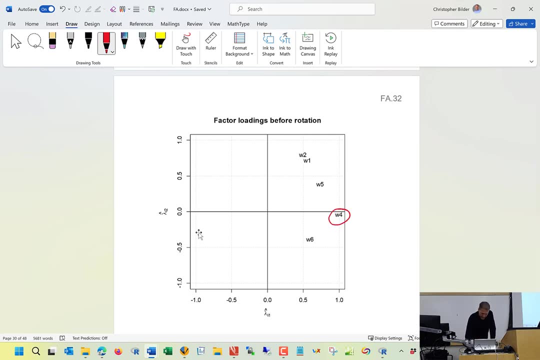 Now notice where w4, let me actually jump on over here to my notice where w4 falls. So it has a lambda hat 1, when I would write out the model that is quite close to 1.. Let's actually just to verify that. 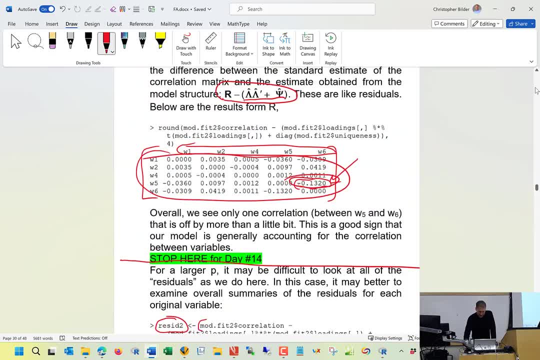 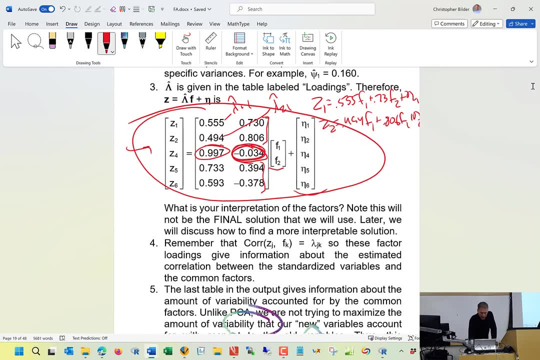 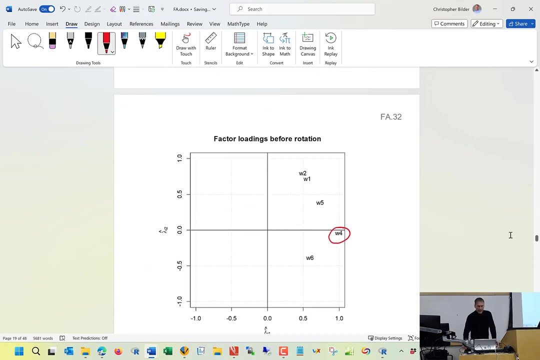 Okay, And we actually did write out the model. Notice how that was close to 0.. Notice how this was close to 1.. And we see that geometrically on that plot. So it's easy to understand how the common factors Are representing, how they correspond to w4. 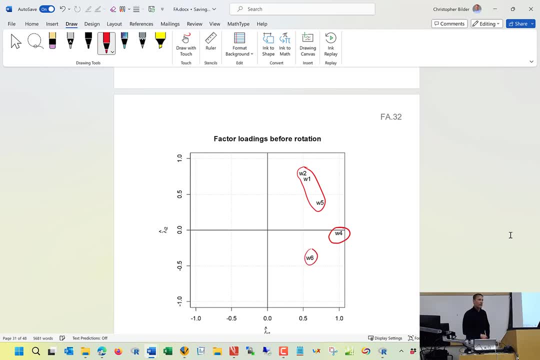 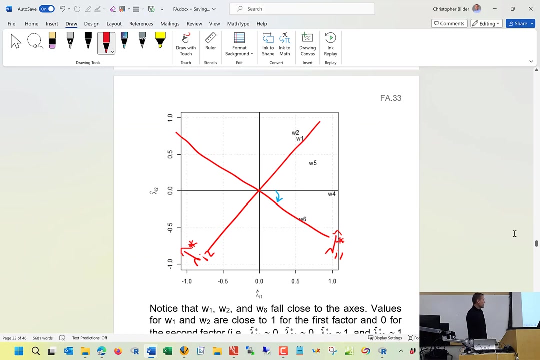 It's not as easy for these. Okay, But what if I could somehow, let's say, rotate that x and y-axis- We kind of talked about this before with principal component axis. Suppose I rotate it in the following ways: If I rotate it, that's what's represented in red, And that blue arrow there shows how. 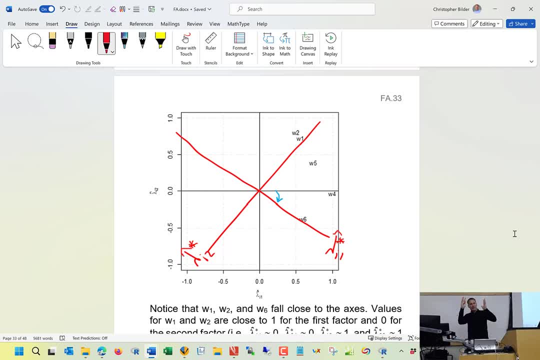 I'm actually, let's say, rotating the axes there. Now we can see that I have, let's say, a new, let's say, x-axis here, A new y-axis here. Look how close w1 and w2 now are to that axis, Meaning it's going to be 0.. Have a lambda. 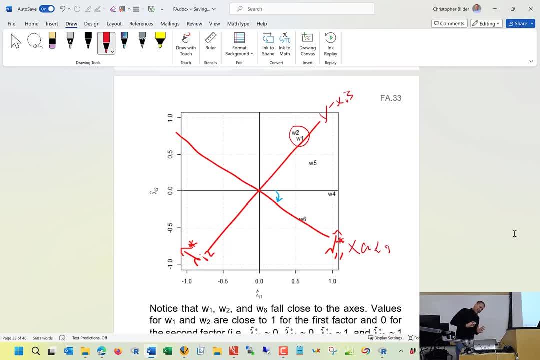 it will have a. have a look at it this way: It will have a 0.. at it this way: It will have a lambda hat 2. that is close to 0, lambda hat 2 star. let's call it that. that's my rotation. lambda hat 2 star. that's close to 0.. I'm 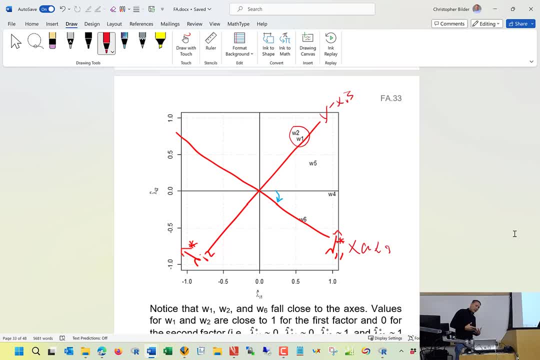 sorry, I got that wrong. It will have a lambda hat 1. that's close to 0.. We'll have a lambda hat 2 that is positive in a way, Okay, maybe kind of close to 1.. Look at where W6 is. It will have a lambda hat 2. that is about 0, a lambda. 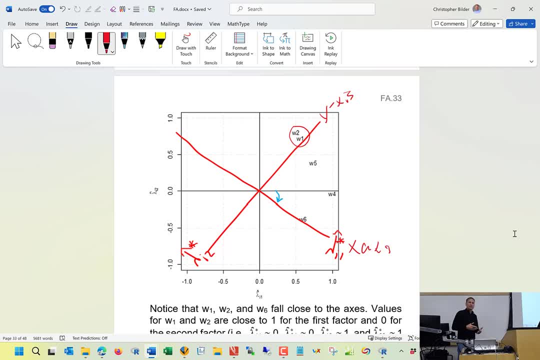 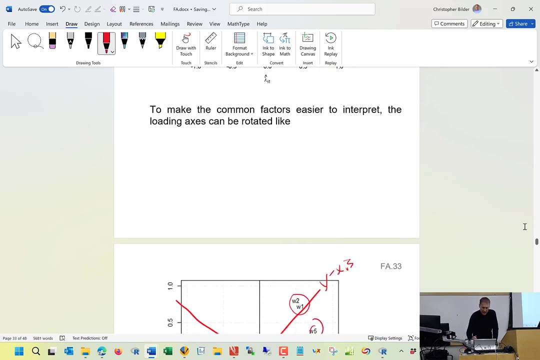 hat 1. that's going to be positive in some way. Now our factor, now small, is going to be a little bit easier to interpret than what we had before. Is it perfect? No, because we still have that. You know if we could somehow ideally do a rotation such that you know. 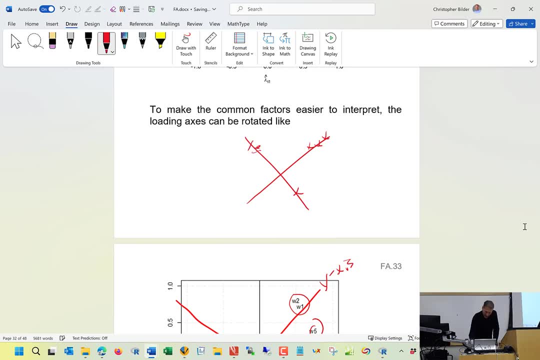 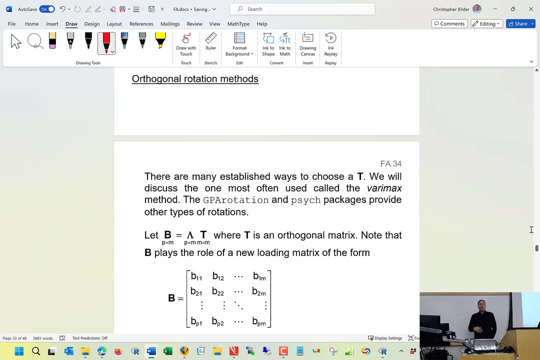 here. Let's say those factor loadings, and they all are right there. That would be great, but we don't have that here. But now we're getting a little bit more interpretable model. Ok, so this where we want to get. How do we get there? Well, there are multiple ways to do this. 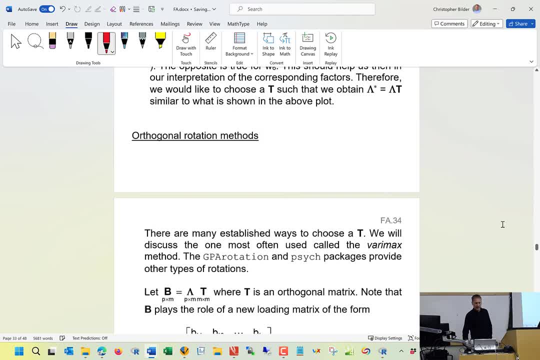 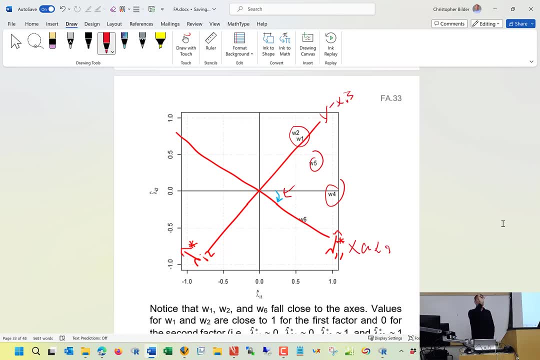 rotation. Now let me also give you a little bit of a side note. There's actually ways that you can figure out what that angle of rotation is. You can say, well, that's a 30 degree rotation. I've taught it before, but in the end I don't. 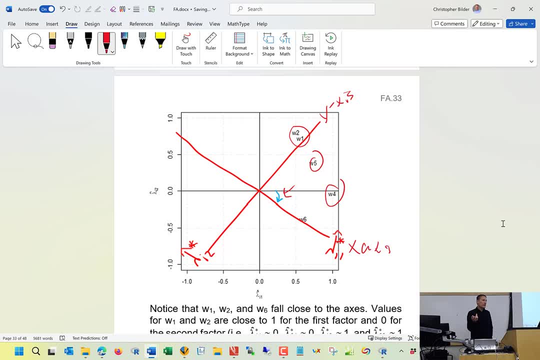 think it's really worthwhile to talk about, because you can only see this in two dimensions. So if I go to three common factors, four common factors, five common factors, it's going to be hard to see it, And so all the time that's spent. 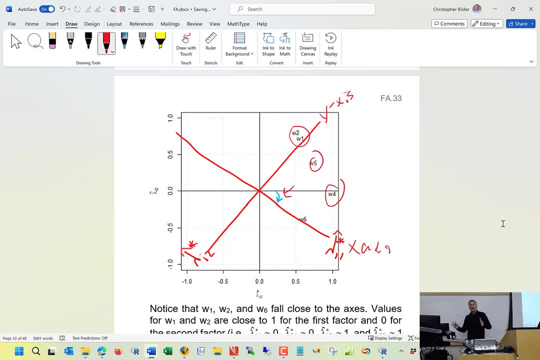 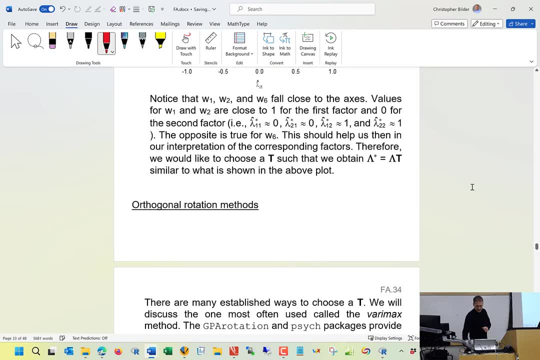 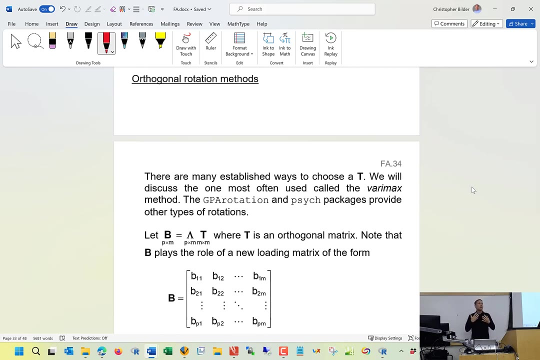 trying to figure out this, all the geometry that's involved with it. it's just not worth it, And so that's why I just leave it more in this intuitive explanation of what's actually happening. So there are multiple ways to figure out how to do this rotation, In other words, to come up with 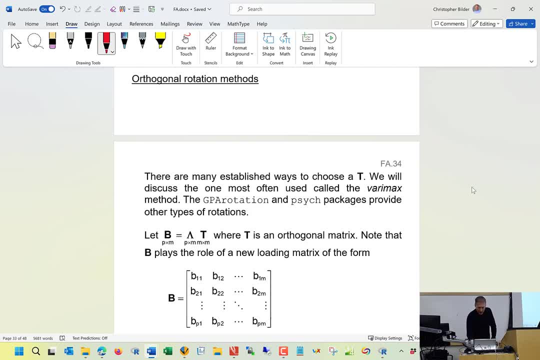 this orthogonal matrix. The most common way is what's called vera max. Notice in its name ver, which actually stands for variance, max, which stands for maximum. You'll see why that's coming up. This is what we're going to use. There are other rotation methods here, some packages that give you. 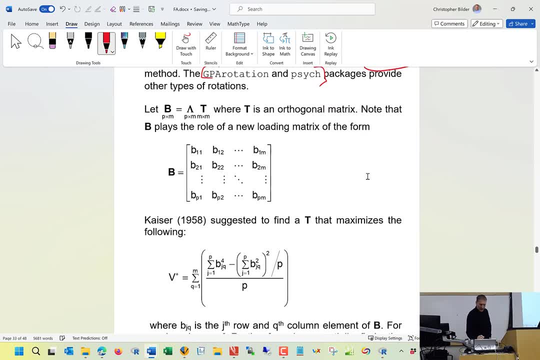 access to them if you were interested. So let's call this lambda t, lambda times t, rather than call it lambda star. let's just make it a different letter. It just helps with the notation. Let's call it b, for the lack of a. better, a better. 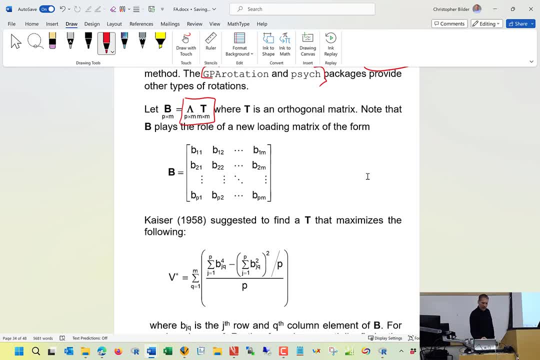 letter And so anyway. so what we want to do is find a t matrix such that we get this b matrix, And ideally so. these will be our new factor loadings, And what we just saw is that- and what makes this easier to work with is when the b's are- 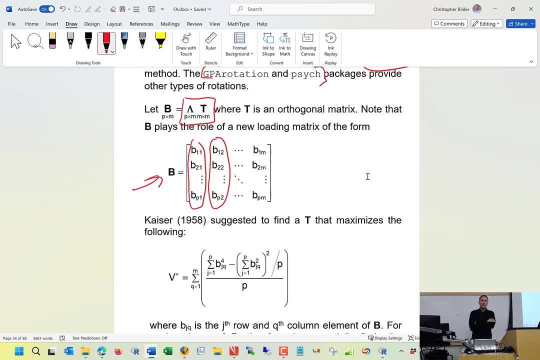 close to 0, or close to 1, or close to negative 1.. And all we're basically going to do is as follows: Since I have a negative 1, and I have a positive 1,, how about we think of the b's squared, so that I always have? 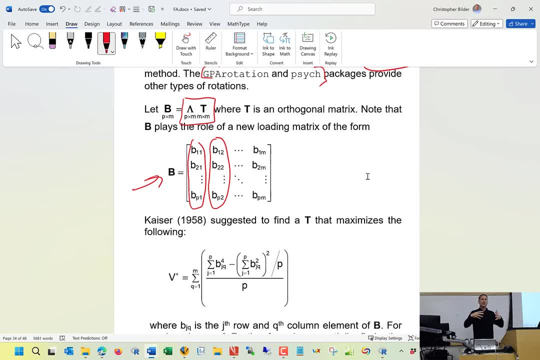 just you know, negative 1 squared is 1, 1 squared is 1.. Okay so how about we look at the b's squared and our goal is to find them, find a set of b's that are always close to 0.. I'm sorry. set of b's squared. 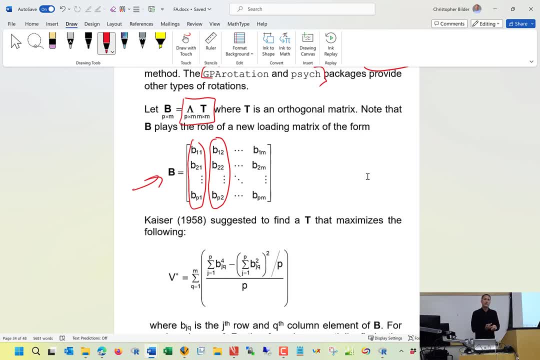 So these are the b's squared that are always close to 0, or close to 1.. So, from an intuitive point of view, what do you essentially want to do with each of these columns, of these b's? Again, these columns are how you're interpreting, let's say, common factor 1,. 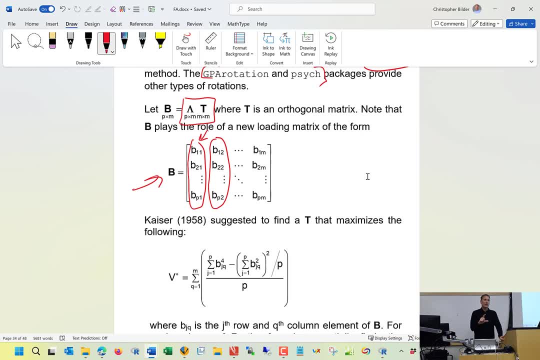 common factor 2, and so on. What would you want to do with these b's? You want to maximize their variance. Again, think about, let's say, if all the b's were either 0 or 1, versus a setting. let's say the b's were about, you know, 0.4, 0.6, 0.5,, in which case are 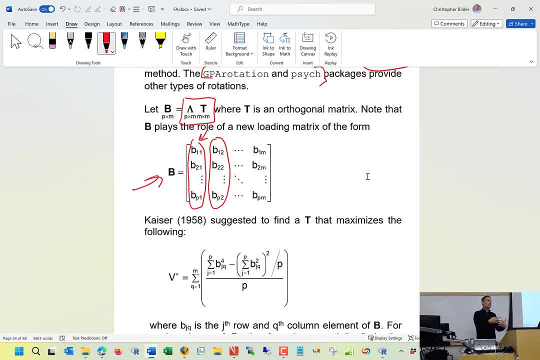 you going to have the maximum possible values of your b's squared, It's when they're all zeros and when they're all ones. So that's why we want to maximize the variance of a column of b's in terms of b's squared. So what we end up doing is this: we try to. 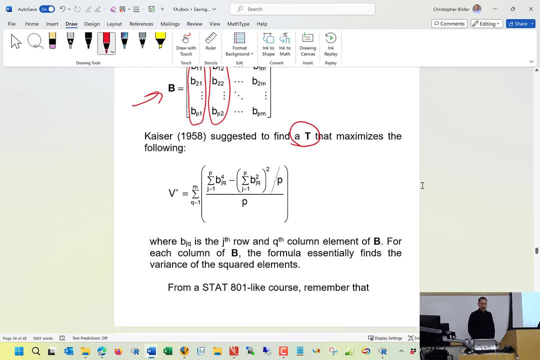 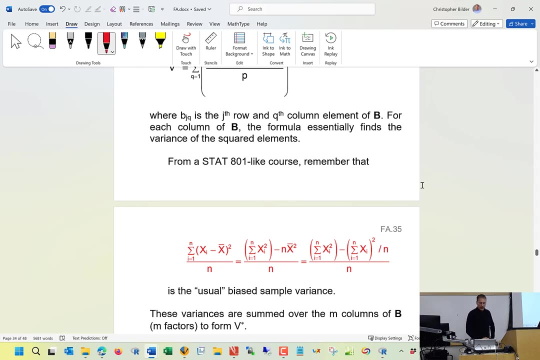 find a t. Okay, That will maximize this expression here, And on the surface you might be thinking: oh, wait a second. that doesn't look like what you just told me about. we were trying to maximize these variances of the b's squared, But in fact it is. 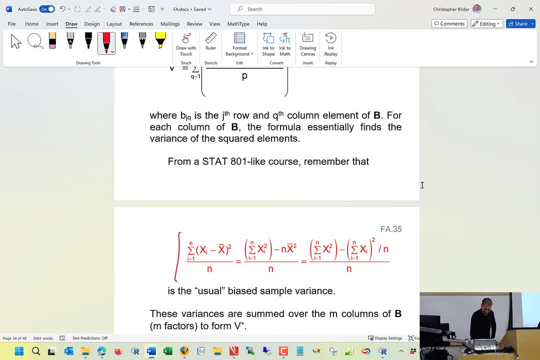 So in your first SAT course you learn about the sample variance expression. Let's say that our data is in the x's. You know we had a sample variance that looked like this: some of the x's might be in the y's. 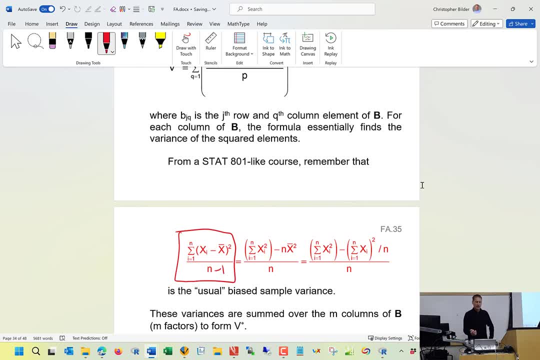 So we're going to do this. So we're going to do the x's minus x bar squared divided by n minus 1.. Let's just work with the bias version of this to match up with what what actually is. it's going to end up happening for us. 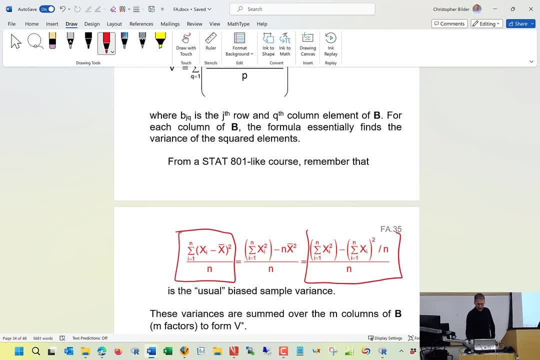 One can do a little bit of math and show that this expression can be equivalently expressed like this: The sum of the x's squared minus the sum of the x's, that quantity squared divided by n, and then the whole thing divided by n. 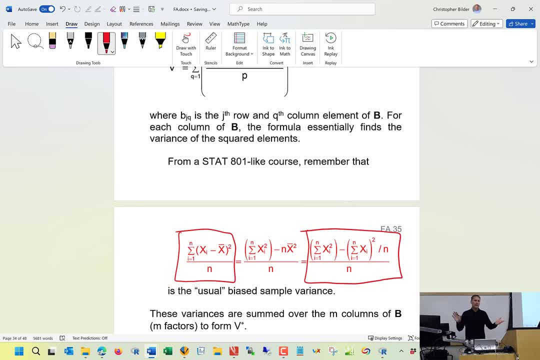 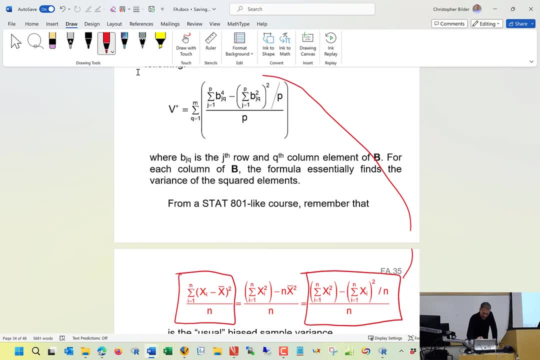 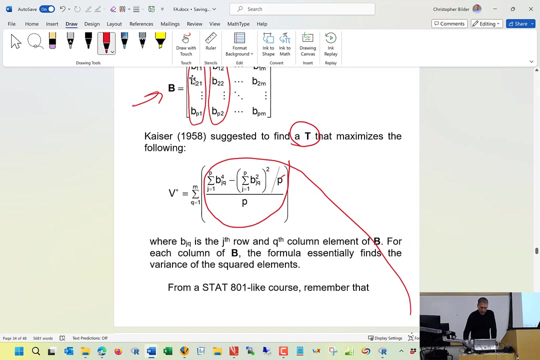 Okay, it's just using some algebra, don't worry about it. though, notice how that expression here it's very similar to this expression. that's in parenthesis. the difference is that the X's now are B squares. okay, that's the only difference. the P here that corresponds to the end that we saw here. P remembers the number. 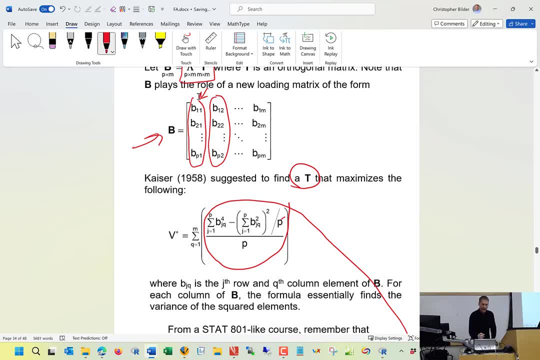 of the original variables that we have, which means the number of rows that we have for our B matrix. so, in other words, what we have here inside the big parentheses, is a variance of B's for a column. you now we have multiple columns, we have M columns, remember M will be the number of. 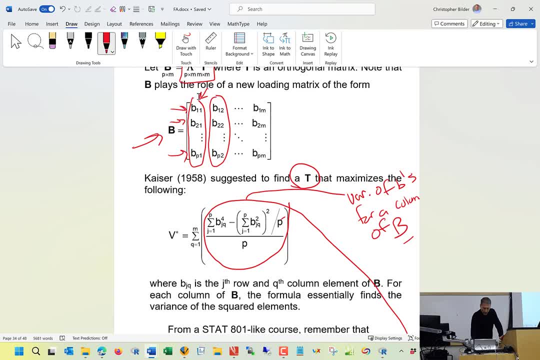 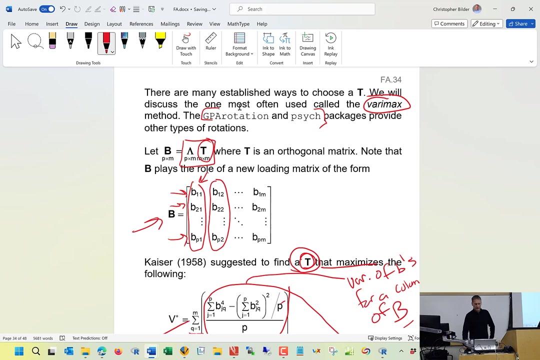 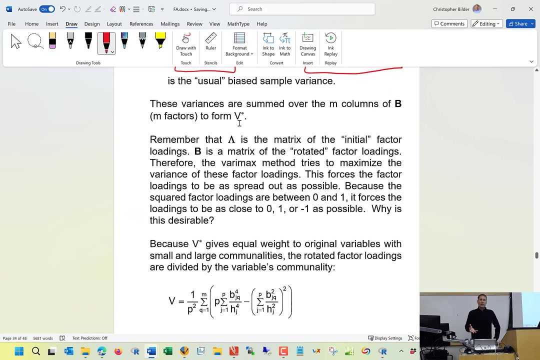 common factors. so how about we just sum over all those columns, these variance expressions, and in the end we want to find a T that maximizes the summum negative? Again, remember where t falls, where it comes about. There are numerically iterative procedures that automatically will find that t for you. 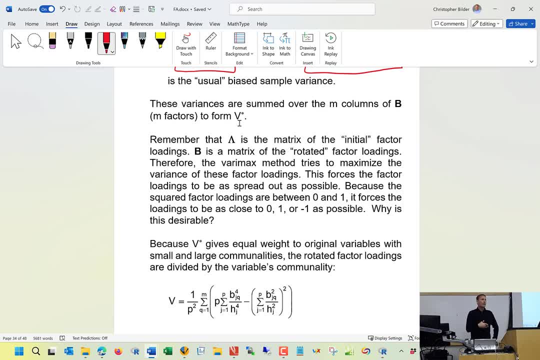 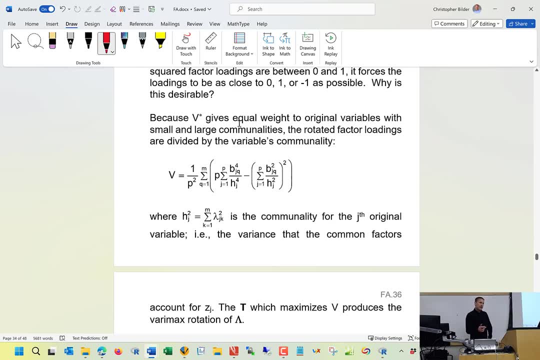 Find them in the corresponding b-score. The fact-anal function will automatically do it for us. In the end, we don't use this expression in the way that I presented. exactly the same. We make a little bit of a change. We divide by the communalities of each of the variables, which just correspond to some. 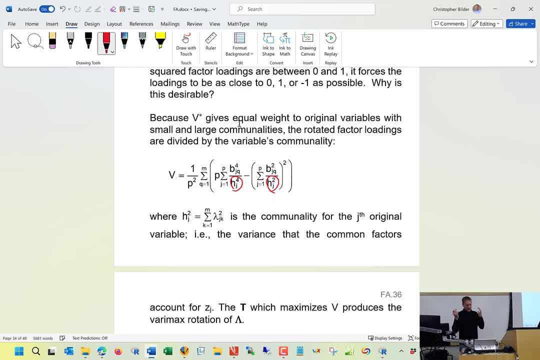 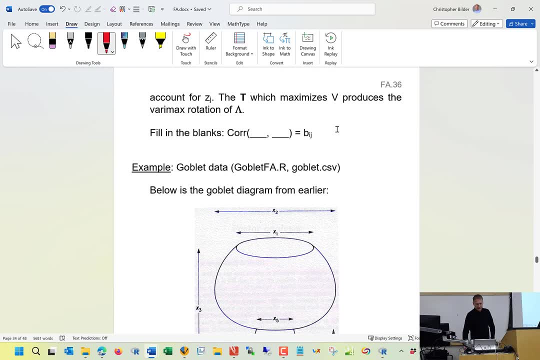 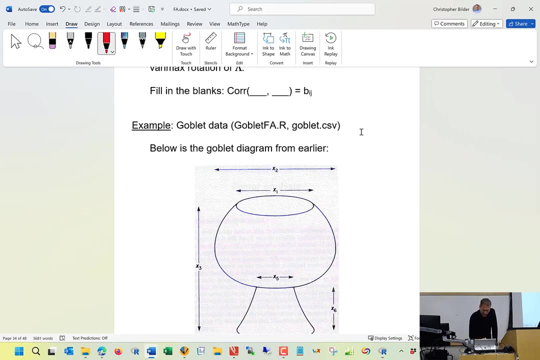 common factors that account for more variance of the original z's than others. Just a very small modification, Okay. Okay, We're getting a little bit short on time here, so I'm just going to fill in the blank for you here. This b represents again it's like a factor loading. 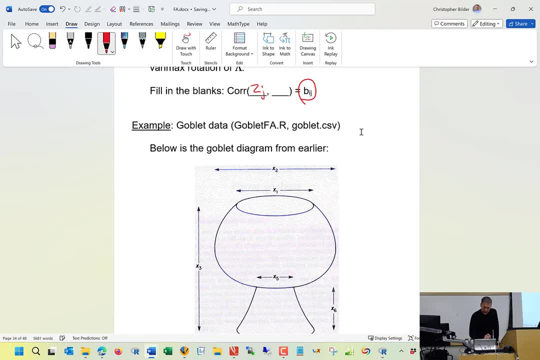 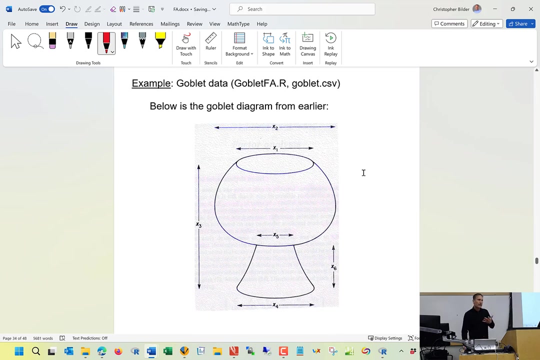 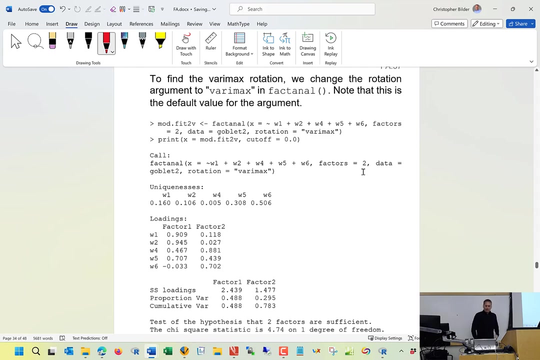 What's going to represent is the correlation between the j-th original variable and now the i-th new common factor that we have. Okay, We'll compare that to what we originally had with the original expression of the model. Okay, Let's get into this goblet data. 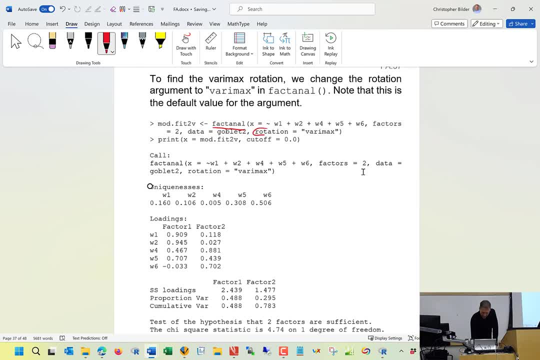 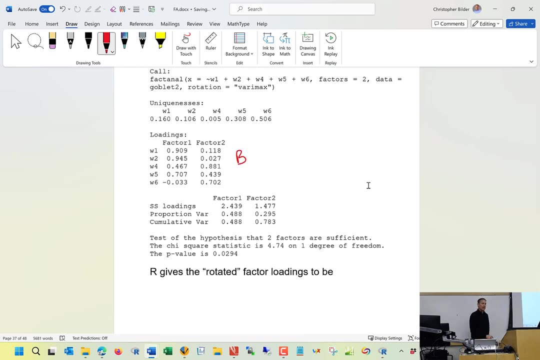 We use the fact-anal function just like before, except now for rotation. Instead of saying none, we say variance: Okay, Okay, Okay. What the R then gives us is: this is our B matrix: Okay, Note that this hypothesis test that we talked about about 15 minutes ago, those results. 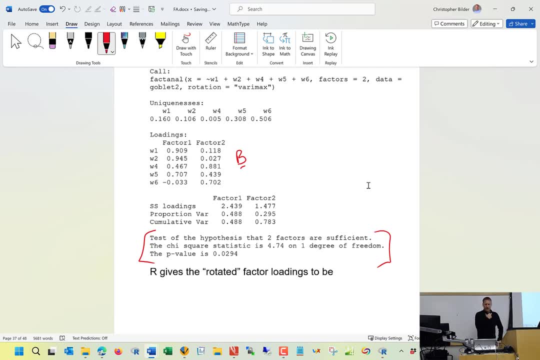 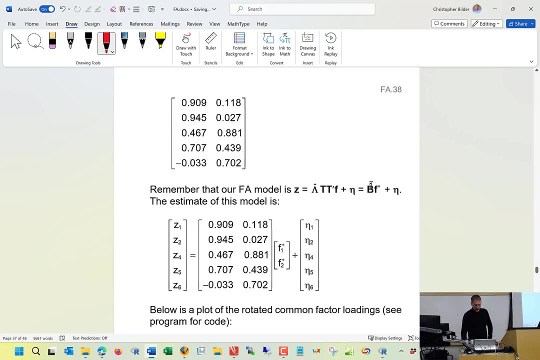 will always remain the same, So don't worry and think that that's going to change. If I were to- let's see here- Write out now my factor analysis, now model, using a very max rotation. this is what I would get, and it's the very 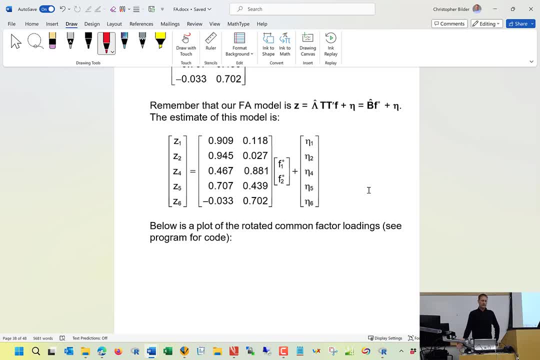 common question that I would ask on a test. now let's interpret this notice for common factor one. so this would be like f1 star. this would be f2 star, representing common factor 1. we can see that, hey, z1 and z2 have a very strong. 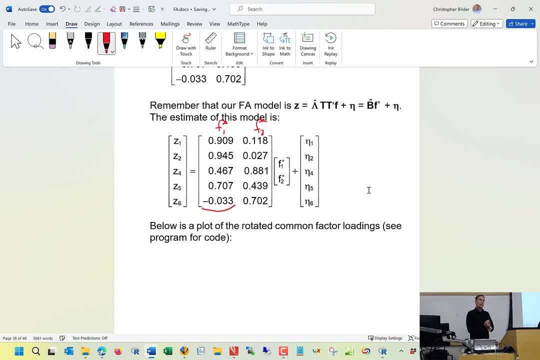 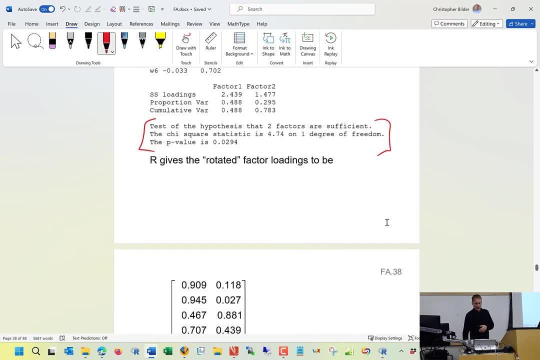 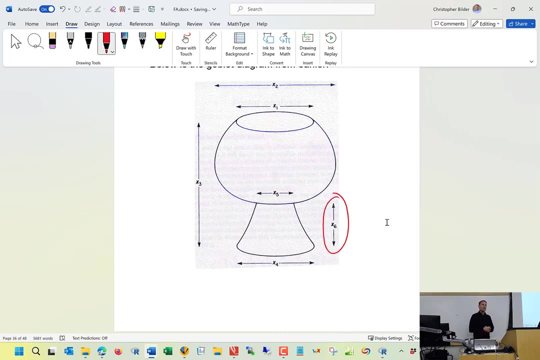 relationship with it, and it has really no relationship with z6. z4 and z5, though, are also related to common factor, so let's think about what that means in terms of this goblet. so z6 is the only thing that's not really playing a role. 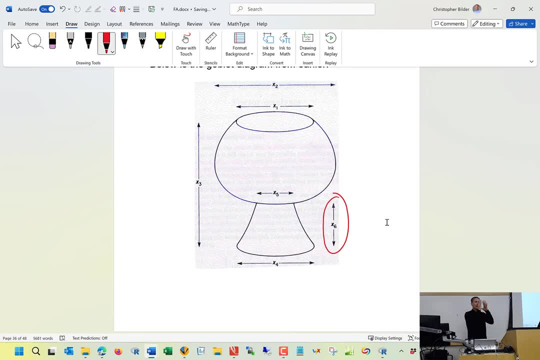 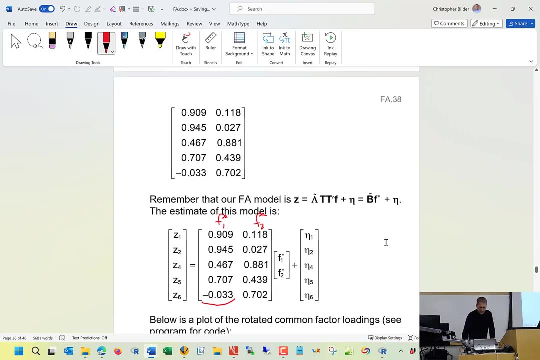 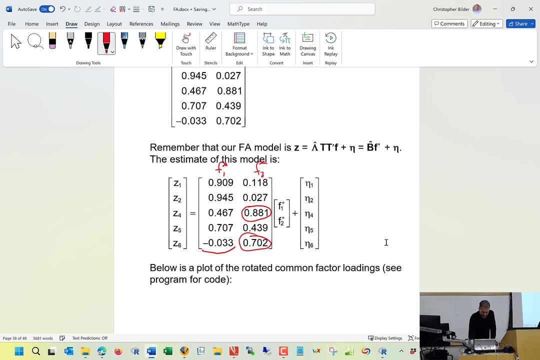 and so what we can see here is common factor 1 is representing essential, the width of the goblet. Let's look at common factor 2.. Strong relationship with Z4.. Strong relationship with Z6.. Very little with Z1 and Z2.. Okay, What are Z1? 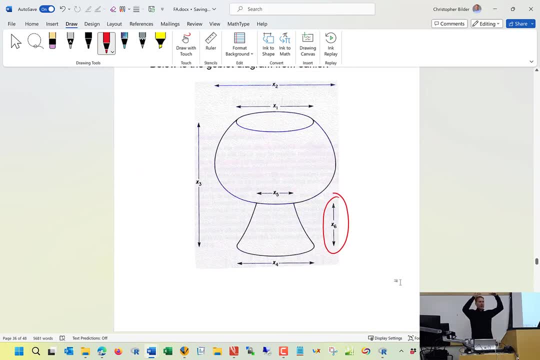 and Z2?? Remember, they represent the top of the goblets. Well, Z1 represents the opening of the goblets And Z2 is the width of the cup, And so the other variables are playing an important role for common factor 2.. So 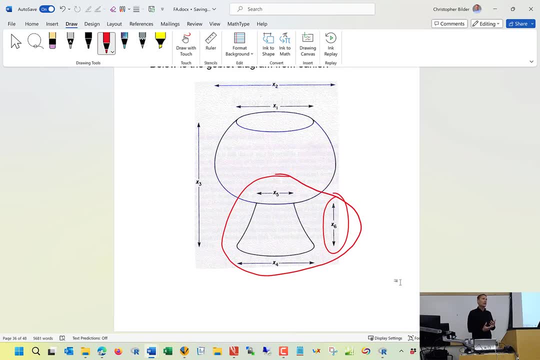 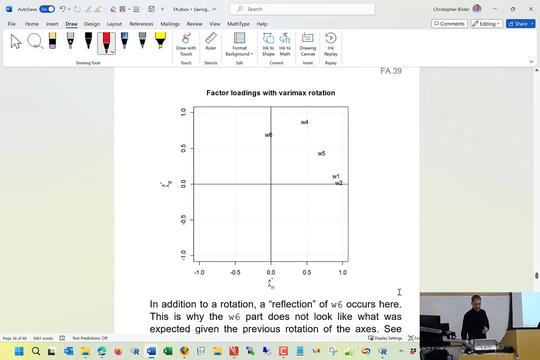 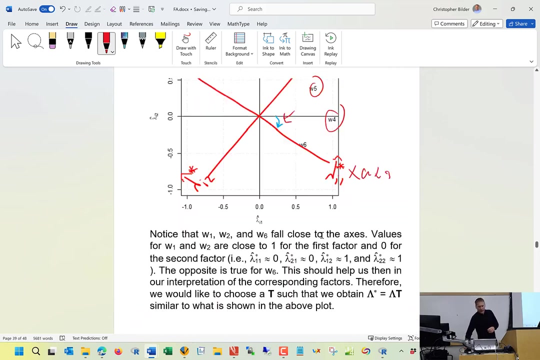 we can think of now. common factor 2, after this rotation is representing the base of the goblet And so, using similar code as before, I actually did a plot of those common factor loadings. This looks very, very similar to this kind of ad hoc way of me doing the. 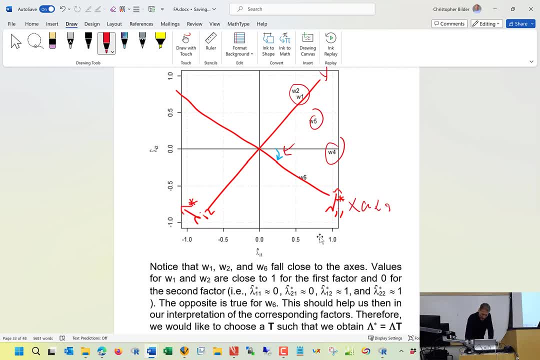 rotation. The big difference, the only difference, is this: right here, This W6 is actually represented up here, And the reason being is because not only is there a rotation with some of this stuff, there can be what's called a reflection, And 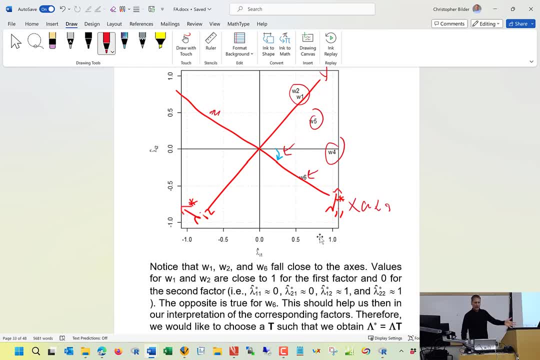 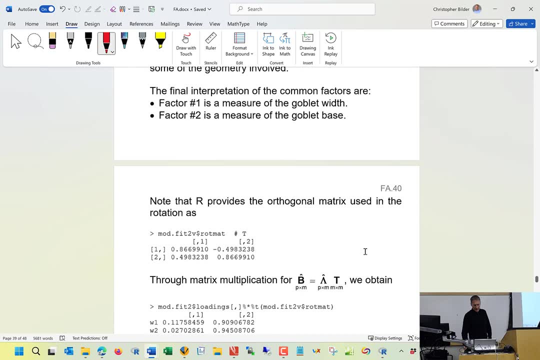 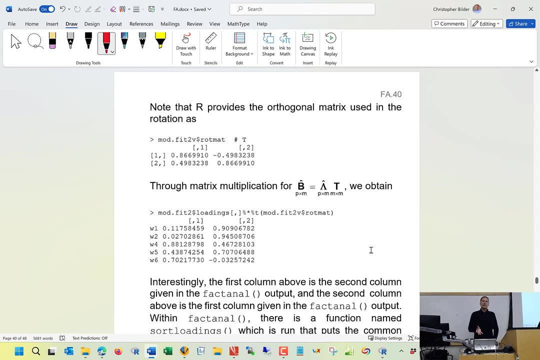 basically, this W6 has been reflected to the other side. It's not a big deal. That's why it looks a little bit different. Okay, Now you might be wondering: okay, what was the T matrix that did this rotation for us? Well, you can actually extract it from the results of 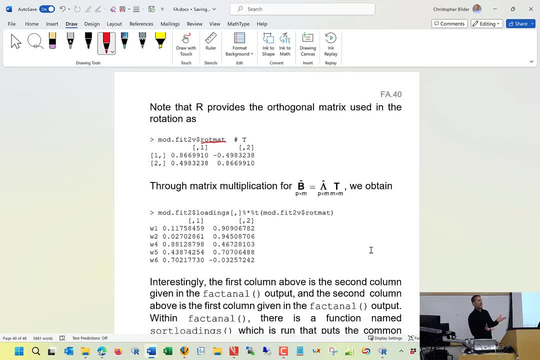 estimating this model. There's a rot, not rotation matrix component. This is my T matrix. So if I took my original lambda hat matrix when I did not do a rotation, times this T matrix, then what I will get is my B. The columns are actually reversed. It's. 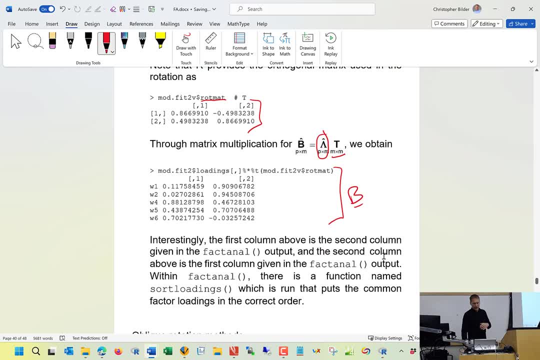 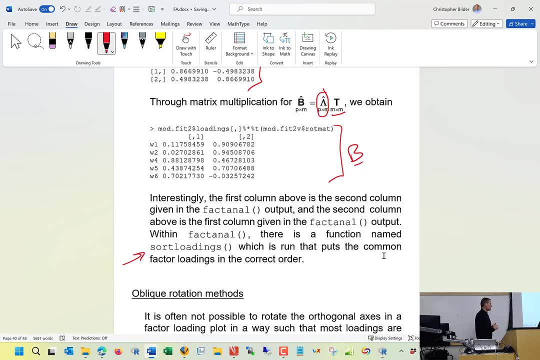 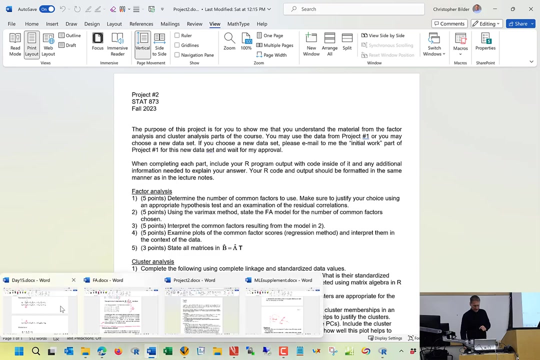 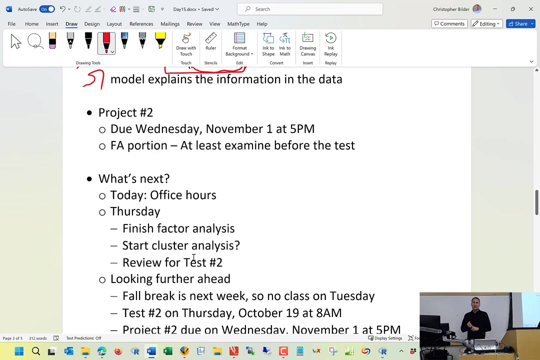 not a big deal there. It's just that's what can happen sometimes in R with inside effect, and it will actually make the correction Okay. This is a good place to stop with the notes. Really briefly, I'm going to talk about project number two. This is due Wednesday, November 1st at 5 pm. Same. 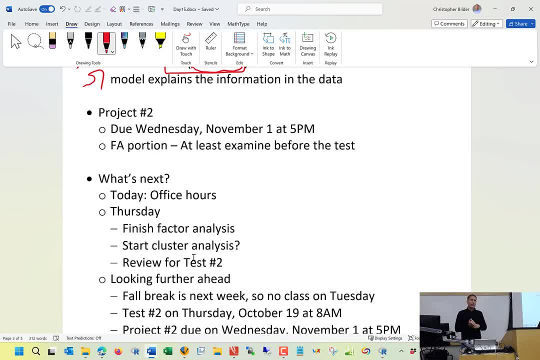 format as the previous project, All the groups should be able to use their previous data sets for project number one. If you have problems conceptualizing- conceptualizing how you would use it- I don't think you will, but if you do, just let me know. 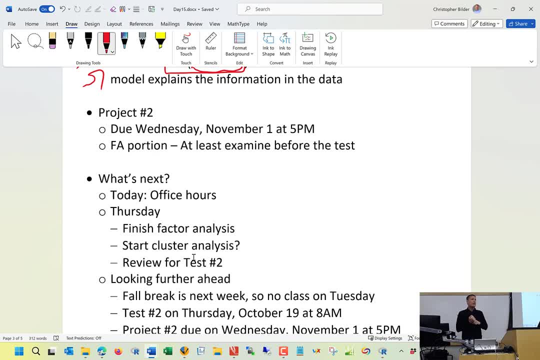 If you want to use a different data set, that's okay too, but you need to get the data set approved by me first before you do it yourself. This project has two components: Factor analysis part and a cluster analysis part. The cluster analysis is the next set of notes of what we're going to do after factor analysis. 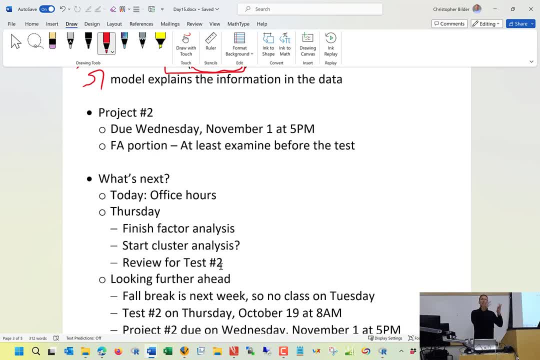 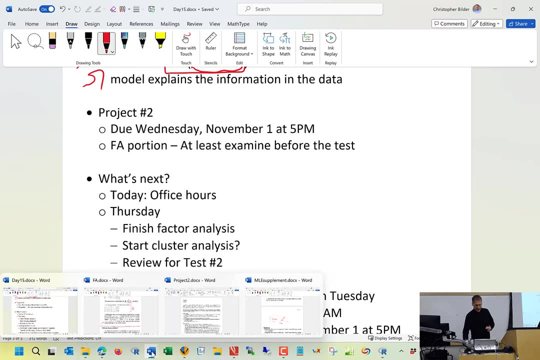 There's not always a good way to assign projects corresponding to the tests. In this particular case, factor analysis is on test number two, which will be next week. So what I recommend that you do is that you take a look at project number two here. 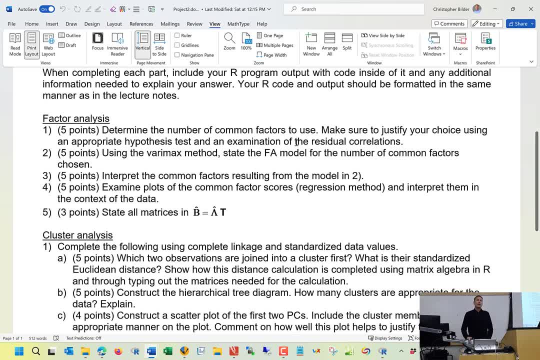 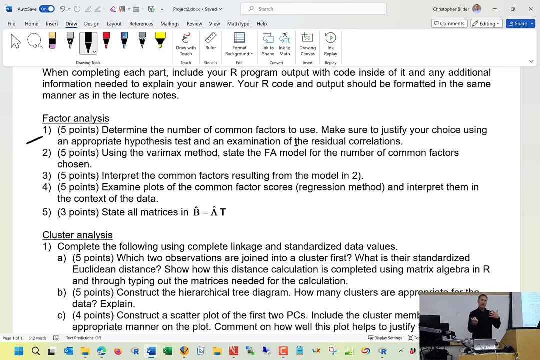 and only focus on the factor analysis part for now. You have five problems there. This is what I think is important about factor analysis: for you to know for the test, Determine the number of common factors used. We talked about that today, You know. use the residual. the correlation make, I'm sorry, use the residuals. 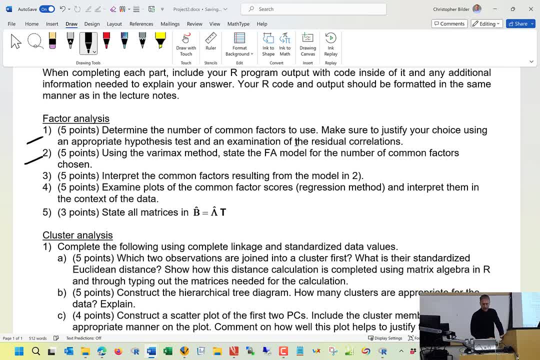 in addition to the like ratio test to help make that judgment. Be able to use the Verimax method to come up with a new factor analysis model. be able to interpret the common factors- This is what we did at the very end- State all the matrices corresponding to that rotation.